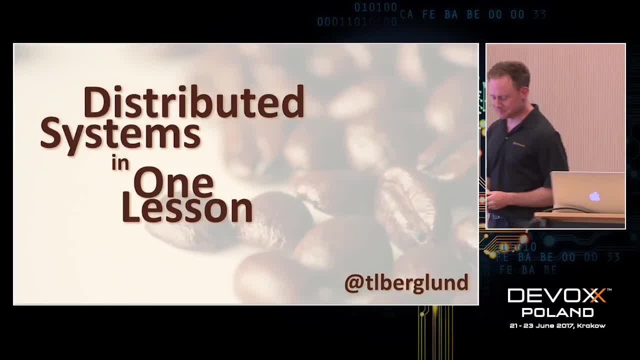 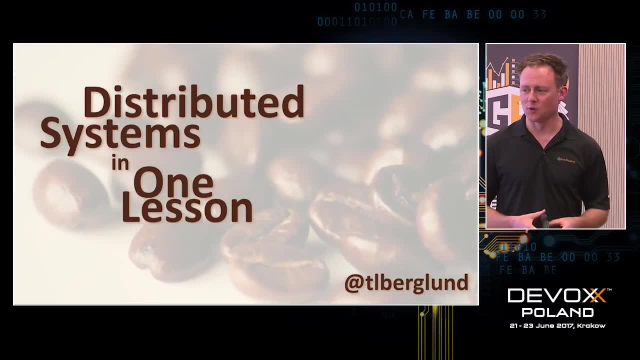 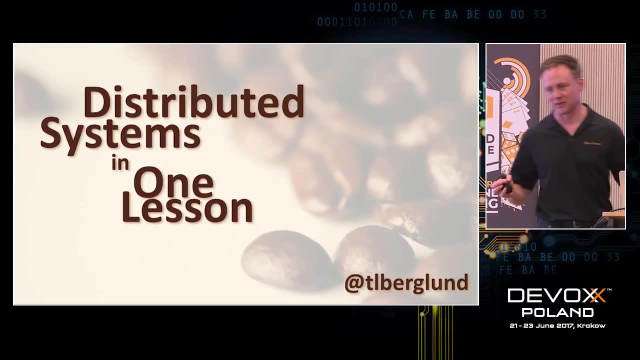 in One Lesson, then you are in the right place. A little bit about me. I already said my name. I'm Tim As of a couple of months ago. I work for a company called Confluent And a lot of my attention is shifting to Kafka and that whole ecosystem. That's what Confluent does. 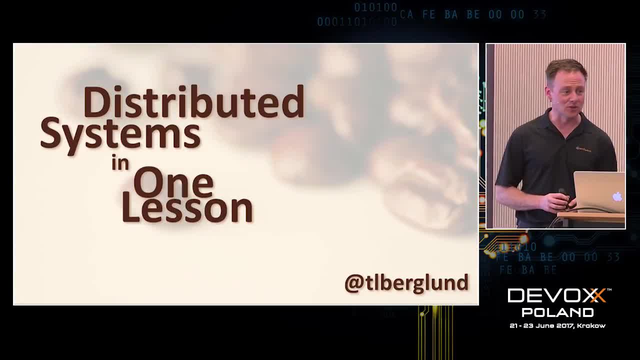 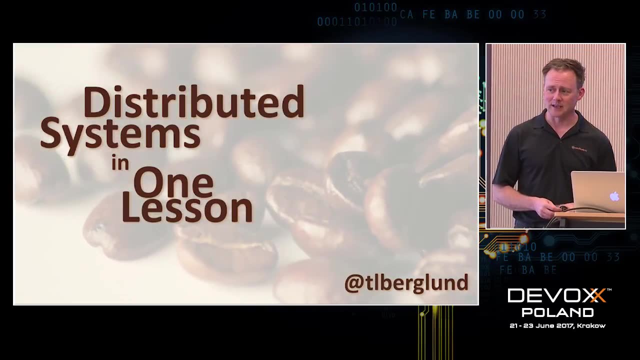 I'm the director of developer experience there, So my team is in charge of documentation and evangelism and making sure meetups are staffed and training and all those things. So it's not a big team yet, but we're hiring And it's an exciting time to be at Confluent. 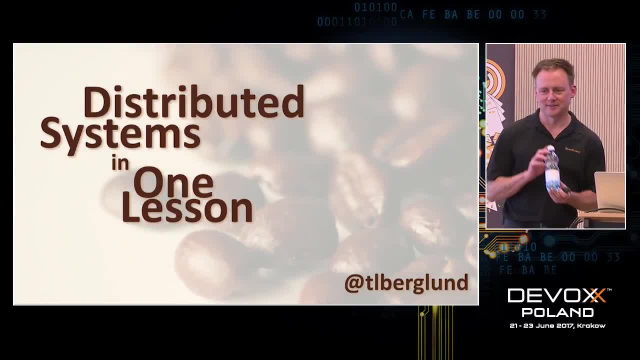 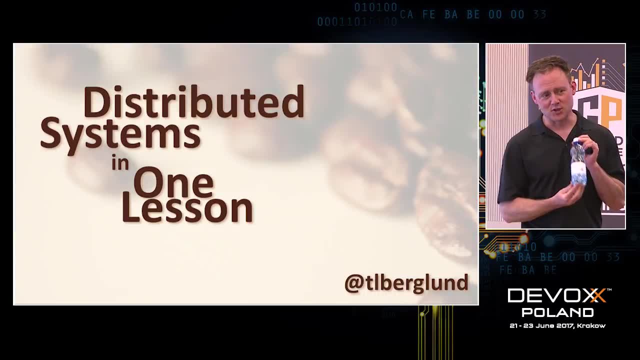 Also an exciting time to be here. I realized, just so you know. I picked up a bottle of water and I thought it was still water And it turns out it is light, sparkling water. And do you guys know, when you have a microphone, if you have a choice between still water? 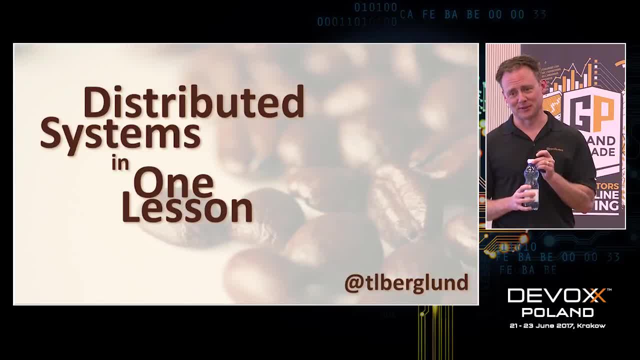 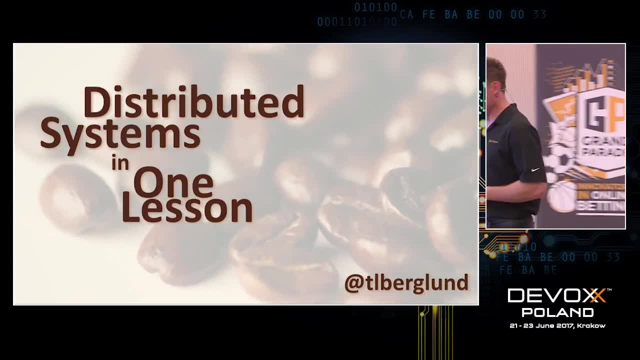 and sparkling water always go with the still water, So I might not drink very much of this. Anyway, we've got about 50 minutes to spend together And I want to talk about what a distributed system is and why they are terrible. Now this might seem strange. 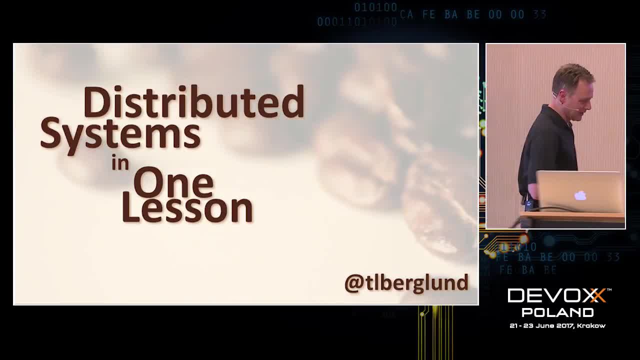 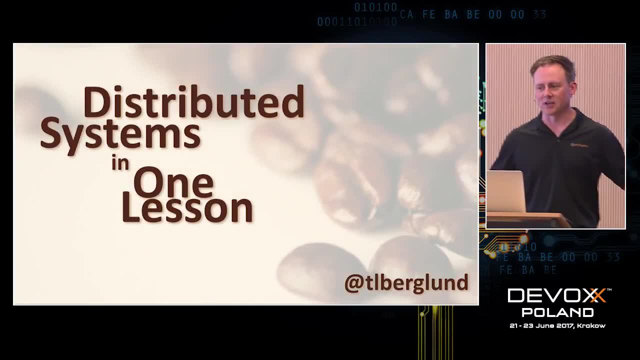 coming from a guy who makes his living in distributed systems- and has for some years- But that's kind of a theme of this talk- is you really? if there's anything I can do to talk you out of building a distributed system and choosing a simpler life, I want to. 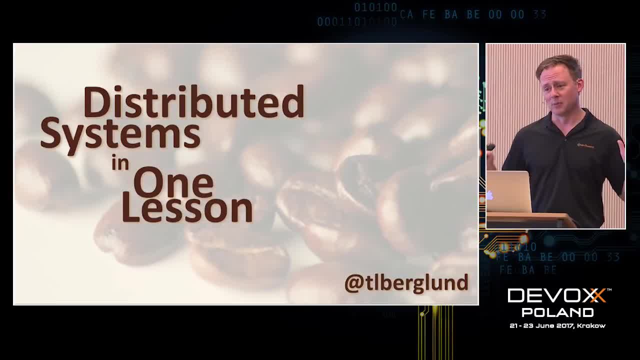 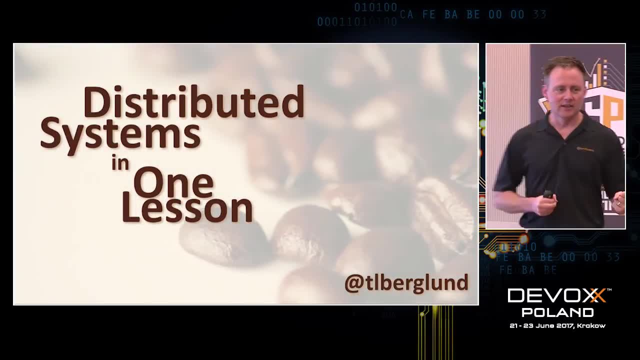 Now, I know I'm going to fail. I know you're going to do it anyway. I know you're going to fail, But we'll talk about the various things that go wrong. when we try to do simple things like store data, compute data, move data from one place to another. All of those things are relatively 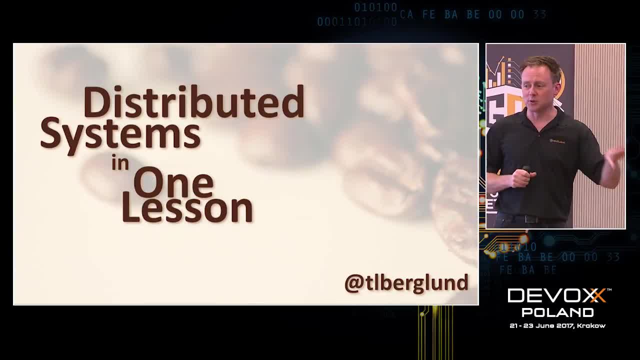 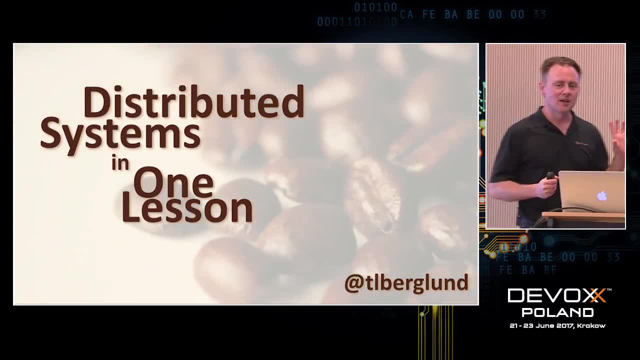 easy at small scale on a single computer. When we get multiple computers involved, they become terrible. So I'm going to show you the things that go wrong And for each category of things we'll talk about storage and computation and messaging. For each category of things 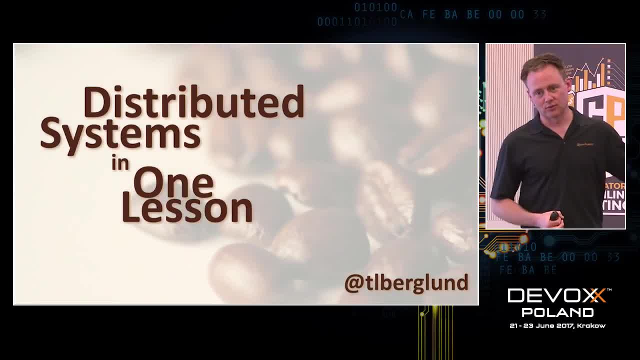 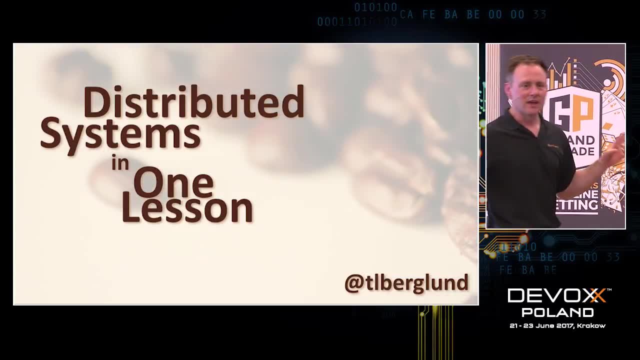 I'll try to dive into an open source technology that addresses that problem. That's really what we're doing today, Kind of an introduction to some topics, an introduction to some open source technologies that solve the problems that come up when we build distributed systems. 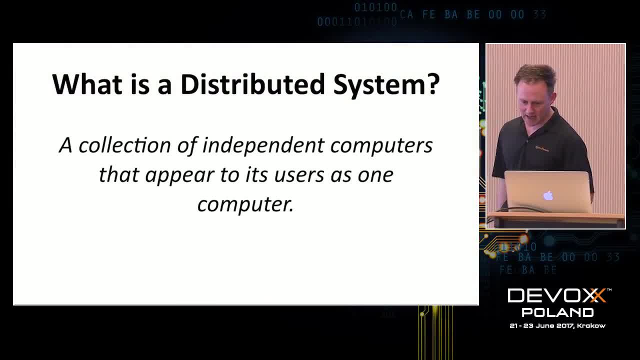 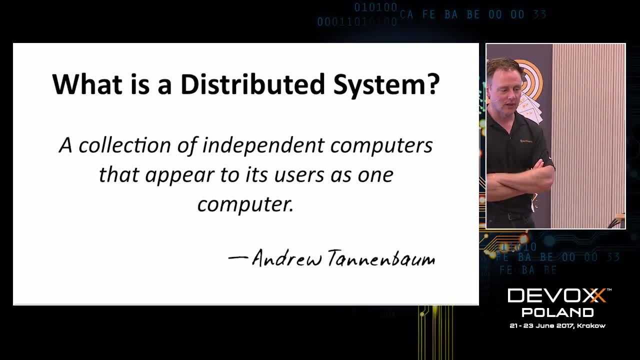 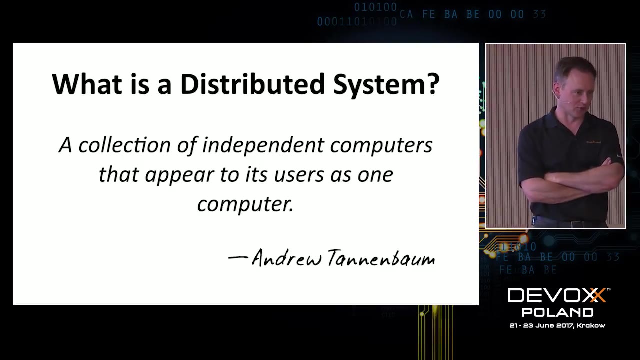 A definition might be in order. Andrew Tenenbaum defines a distributed system as a collection of independent computers that appear to its users as one computer, So you might say something like Amazoncom. I guess it looks like one computer. So that would be a distributed system, A Cassandra cluster, a Kafka cluster, all of these things at one level. 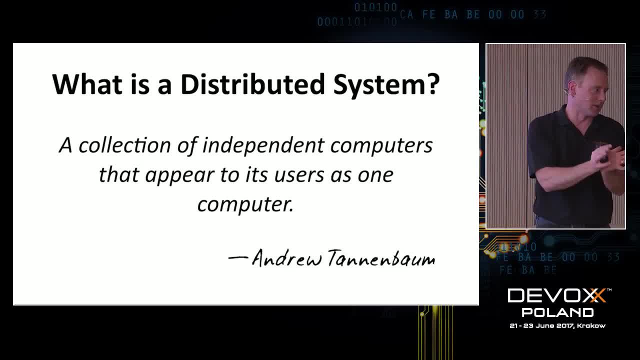 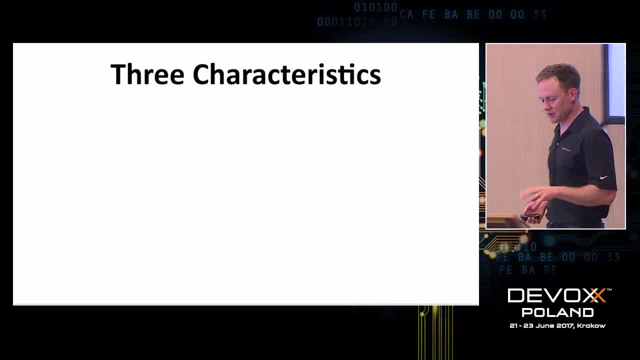 of abstraction or another, they act like a single system, But in fact they're composed of many computers. Now, distributed systems have three characteristics. for something to qualify as a distributed system, It has to be made up of lots of computers. They have to identify the 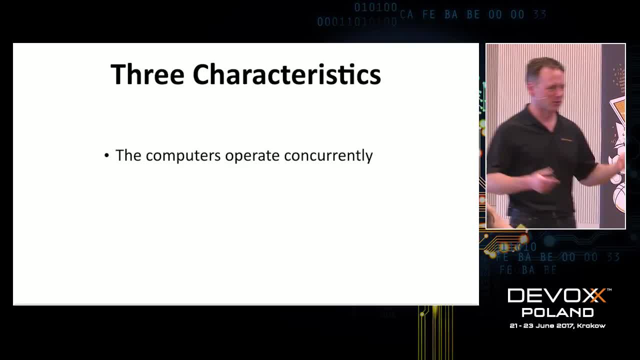 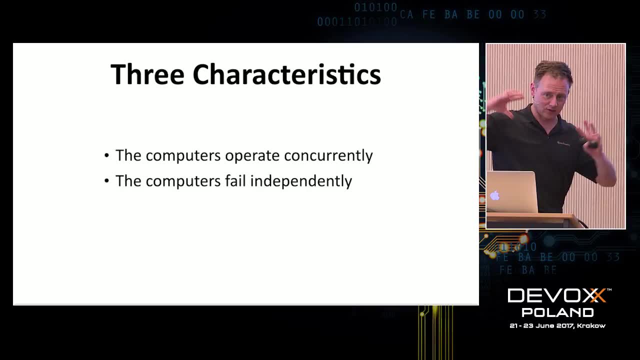 computers that operate concurrently. That's kind of obvious, right. These computers are all running at the same time. They might fail independently, And the possibility of one of our machines failing is a specter that is always looming over us. We just have to deal with that, And here is those. 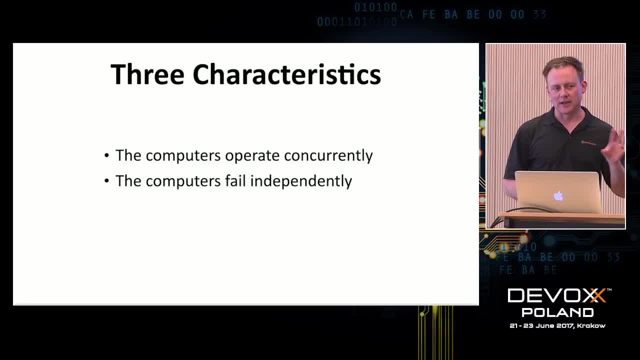 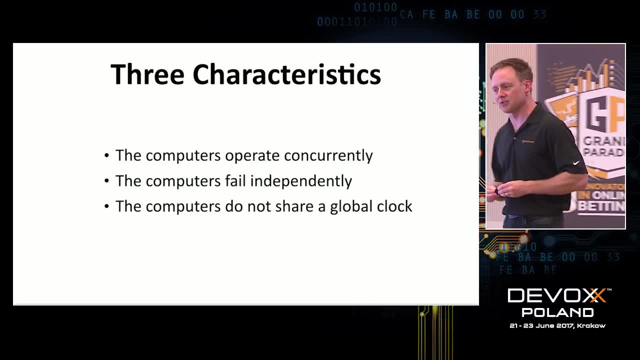 are, frankly, are two trivial things. This last one is a little subtle, And this is what makes things interesting. The computers don't share a global clock, So if you ever have a collection of processors that are in some sense synchronized, that their clocks are synchronized, that technically is not going to function as a 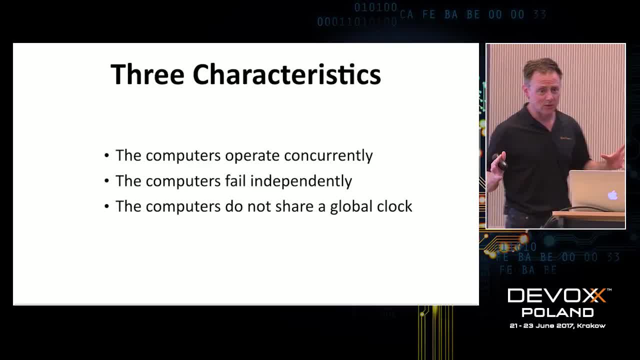 distributed system And all of the various terrible things that happen when we build conventional distributed systems. some of those terrible things won't happen if you have a global clock, But that's just not practical. That's not how we build real systems in the real world. So 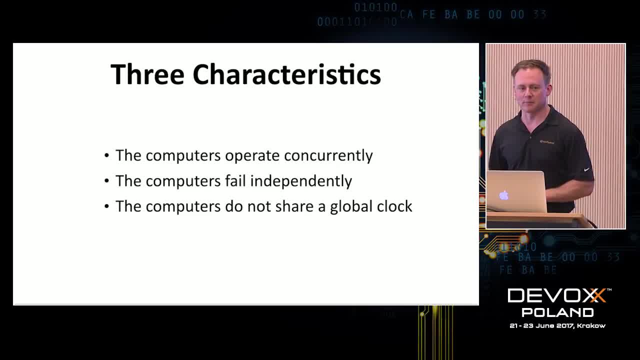 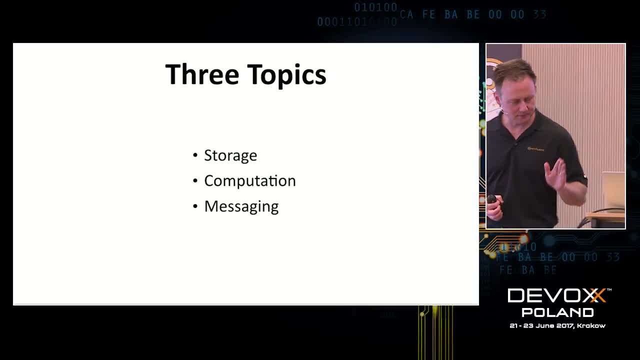 we have independent clocks, independent failure and, of course, computers operating concurrently. That's what I mean when I say distributed system. So, as I said, we will dive into three topics here: Storage, computation and messaging. Now in the single server, single processor, even single thread. 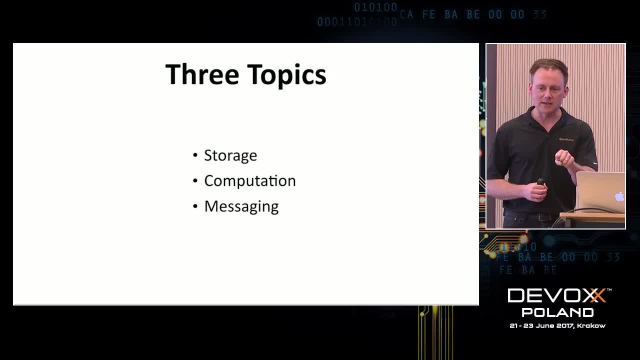 version of these three things. life is grand. These are more or less solved problems And everybody knows how to do them, Like everybody knows how to use a single master relational database. That's a fairly commodity skill. Everybody knows how to do computation in a single thread If you're a. 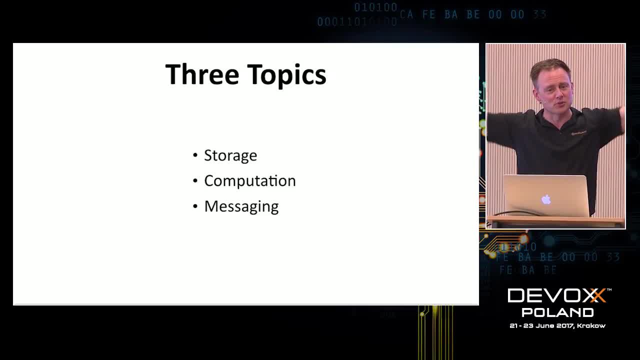 programmer at all, you know how to do that. But when we try to distribute these problems more broadly, life gets real hard And, like I said, I'll look at each one of those And it's my goal here again is to convince you, don't do this, Get an easier. 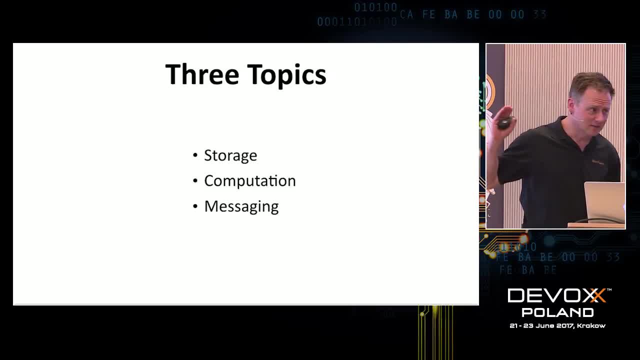 job, Build a smaller system, Live in the country, Slower pace of life. I'm just looking at you. I know you're not going to do it. I wish you would. I'm trying. I got a few minutes left to convince you, But 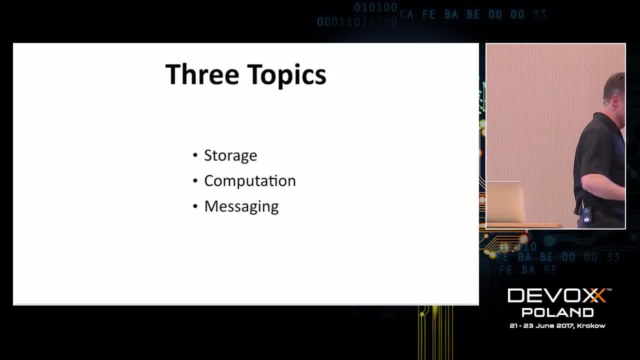 let's see where I get. Also, by way of a shameless plug, there is also an O'Reilly video available on Safari with the same title: Distributed Systems in One Lesson. That's like three or four hours long. I go into more detail And yeah. 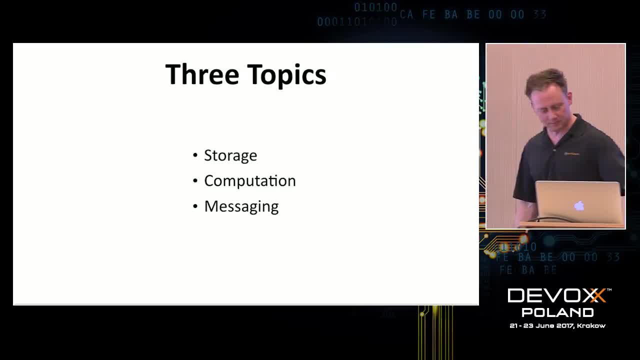 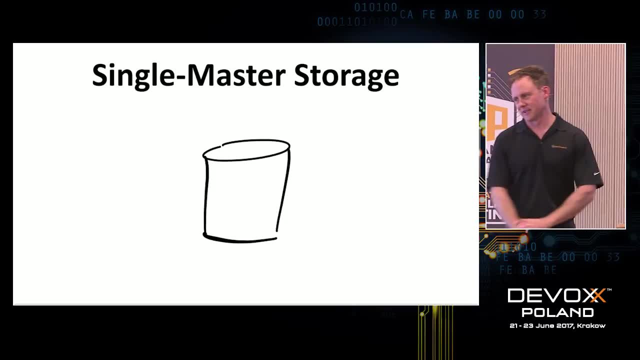 it's by me, So that's the shamelessness of the plug. if you're interested and want more, All right, Let's talk about storage Now. to remind you, single master storage, the pleasant life you used to lead, the salad. 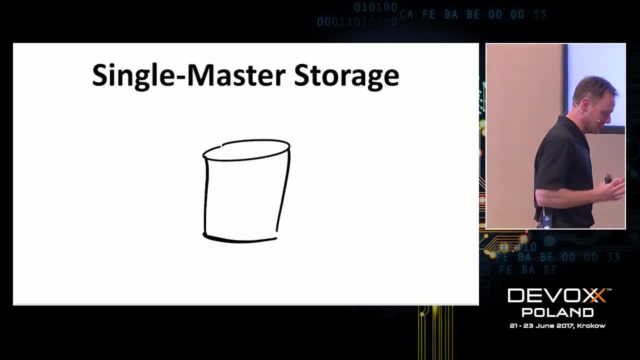 days, the simpler times You have a database on one server, Life gets hard, life gets complicated And if you could imagine the behavior of a database and if you had a slider where you could turn the scale of the system up and down, Certain things happen to us as we crank that scale slider up and the 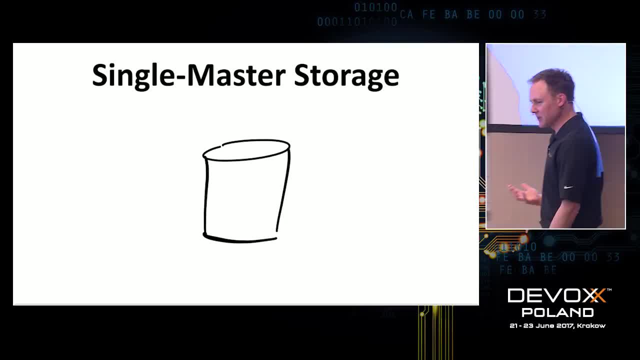 system gets busier and busier. In a lot of web systems there, when everything is simmering in the system, there is always a time that makes the claim. That's the point. As soon as your data has become useful, then you can run it and play some games or whatever, use the diminution block and so forth. So I only have 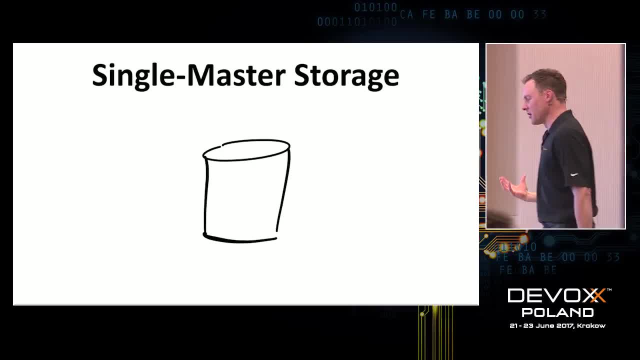 5 minutes to finish this thing here. I wanted to give everyone in the audience a couple of hour ejeuries, but would like to quickly introduce some key points. When you're exploring one behind the camera that you brought in a lot of web systems, there are more reads than writes right. There's more read traffic. 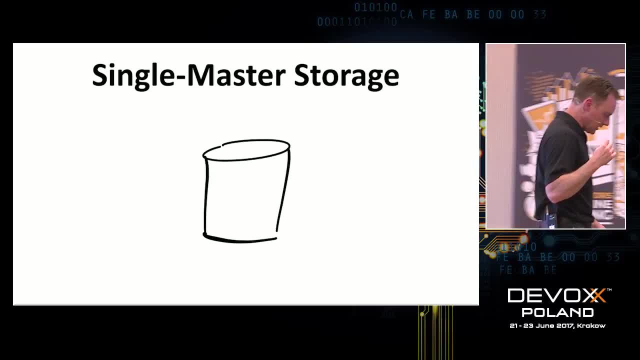 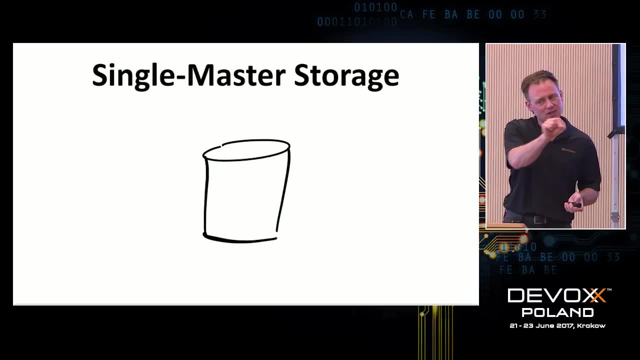 than write traffic Now in a relational database, reads are usually cheaper than writes, so that's okay. But imagine, as we're turning this scale slider up, at some point this single server runs out of gas. we've got all these reads happening, not as many writes happening. 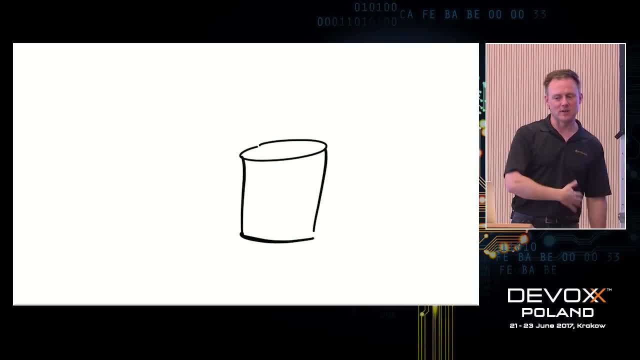 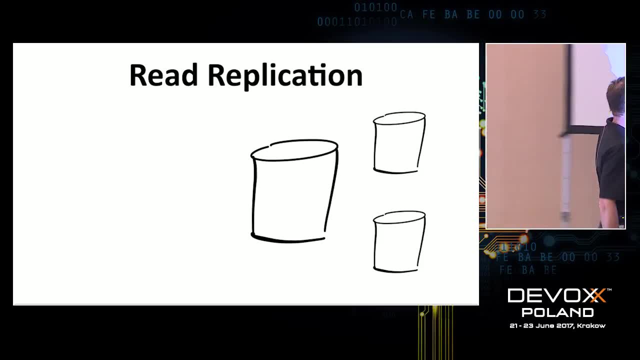 and we need to scale reads. What do we do? We all know the answer: We do read replication. Okay, that's easy enough Here. we'll take writes that go to the master and we'll propagate them to the two follower servers and you're able to do reads against those. keep the writes going to. 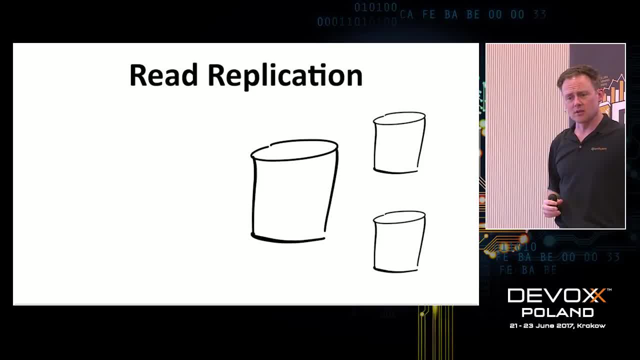 the master and you buy yourself some time right as this scale slider is turning up. Now you've broken something already. You've created a distributed system, a distributed database. It's just not a particularly intentional one yet. And what is the thing that we have broken? 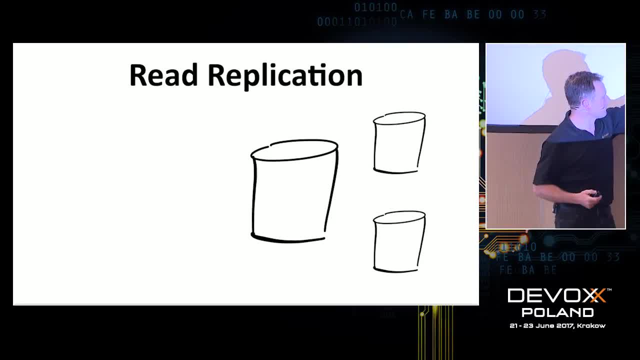 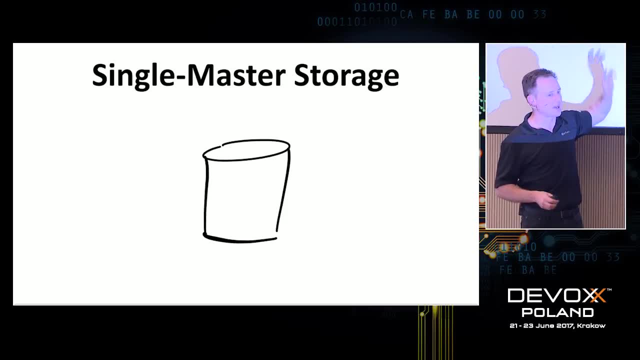 We have broken consistency When we were back in the simpler days can't say I didn't warn you. anytime I write to this database and then I read from it. I am always going to read the thing that I wrote. That is a guarantee and for any database we're. 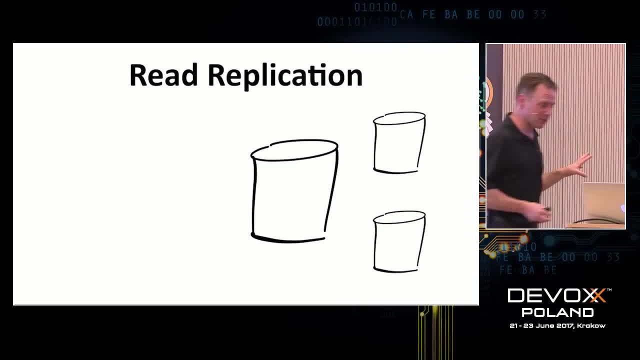 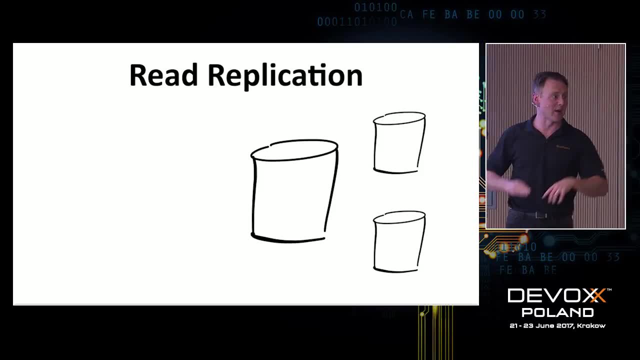 ever likely to use. we're going to read the thing I write Now when I go to read replication. that's not necessarily true. I'm going to write here, and when I read here, that read may not have propagated yet. so I now have an. eventually. 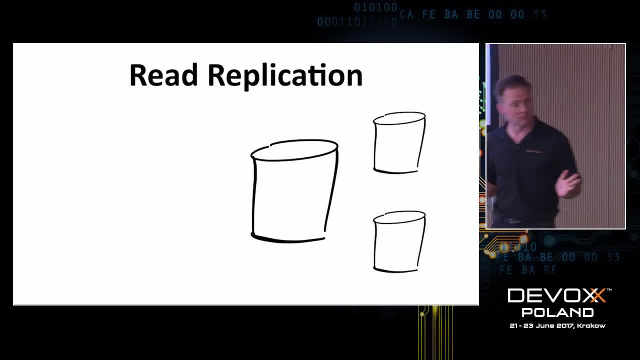 consistent database Accidentally, And the bummer here is that I may be telling myself: well, wait, this is a relational database. I've got strong consistency guarantees, It's okay, but I've broken that, so a little bit of life has gotten bad. Also, this only works for so long. 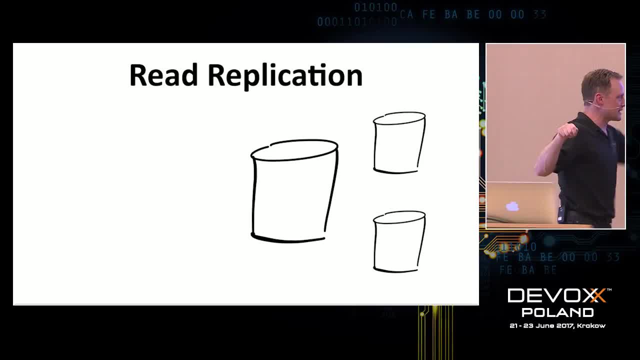 As I continue to turn up that slider. what happens? Well, I can keep adding follower servers for reads and scale my reads as much as I want, but all of the writes still go here, and so I'm going to run out of gas on the database. 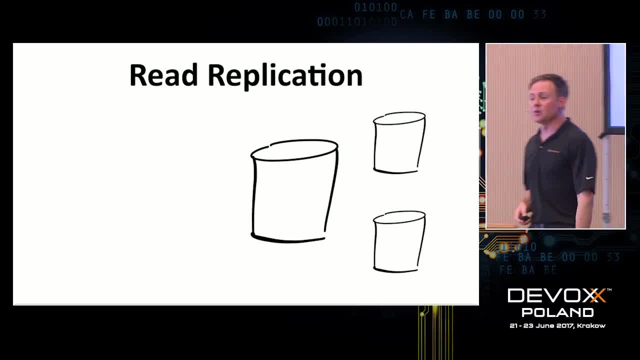 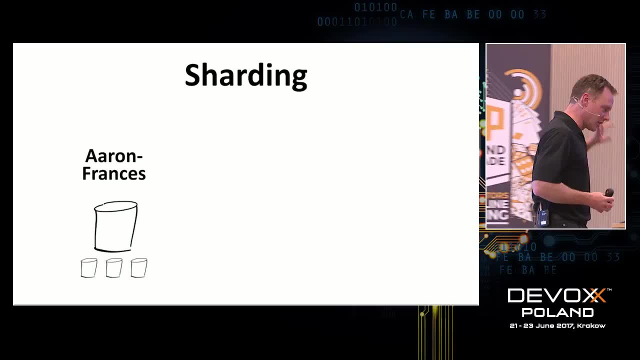 The master on the leader server. So then, I do an even more terrible thing, and that is sharding. Again, this is not a new technique. People have been sharding relational databases for approximately as long as there have been relational databases, but what I do here is I will. 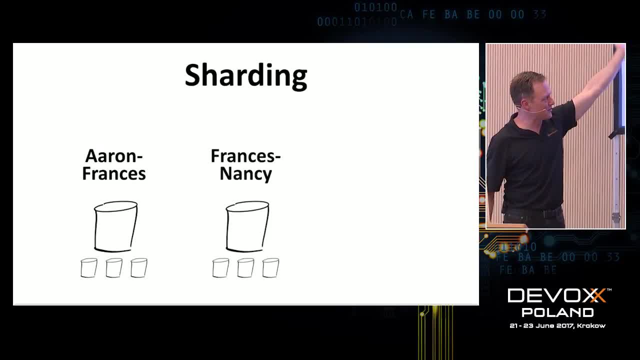 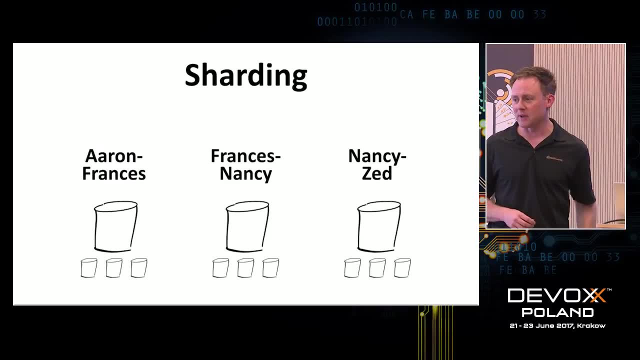 find some key. I'm using name here and I basically just break up the database into three pieces based on that key. So if I'm storing people's settings based on their username, let's say I will pick username as that key and put A through F here, F through N here and N through Z. 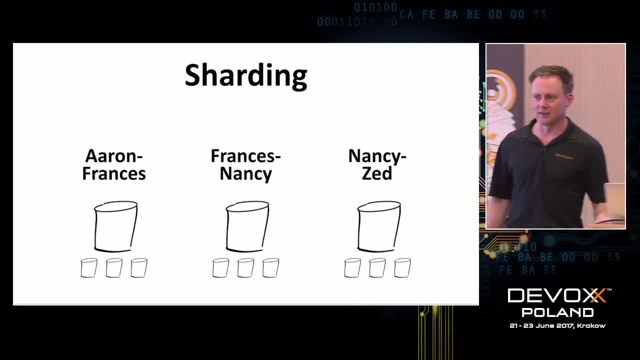 as my people say. on the last server, I suppose I should say Zed huh. No, I'm going to keep saying Z. All right, And each one of these is its own little read-replicated cluster, so I can sort of make. 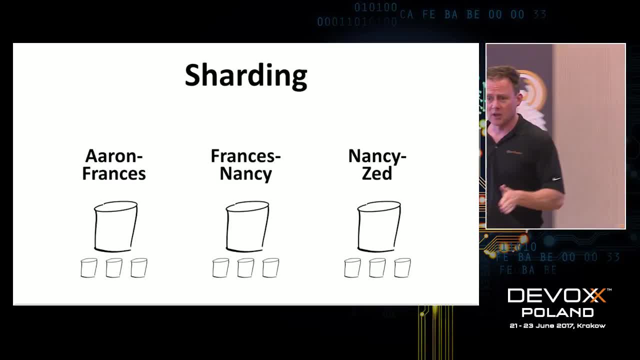 the database as big as I want there. but I've broken something else. I already broke consistency and now kind of I've broken my database. This is my data model. If this is a relational database and when one scales like this, it. 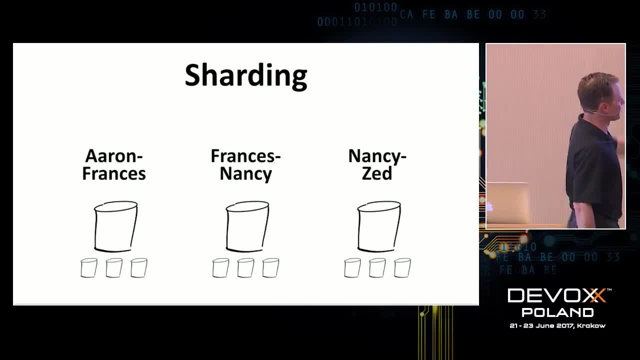 almost certainly is a relational database. Now, for example, I can't join across shards. I've got completely independent databases from shard to shard and that's a little bit of a bummer. That works sometimes. I have a talk later this afternoon where we're going. 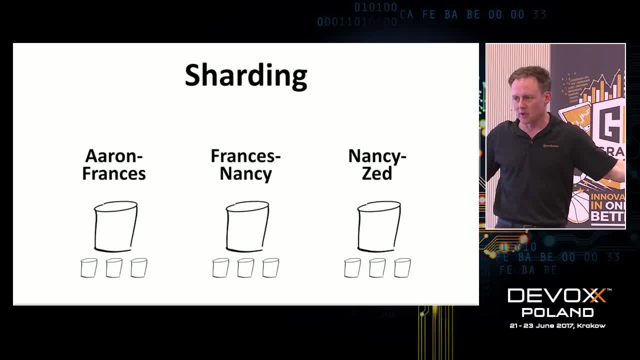 to talk about sharding as a way of scaling an entire system and, in that case, sharding a whole system. Sometimes I get away with that real well, sometimes I don't, and it can be a bit of a bummer. Anyway, briefly, that's just what you do with a database that's not built as a distributed 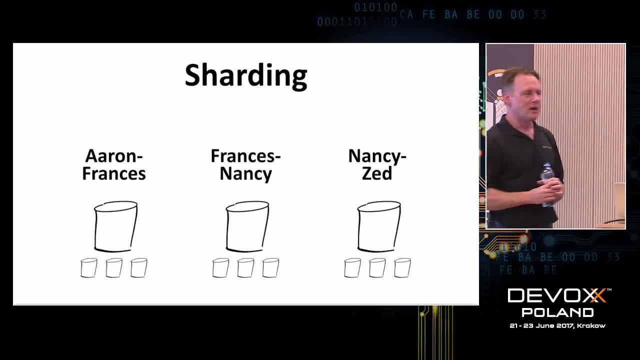 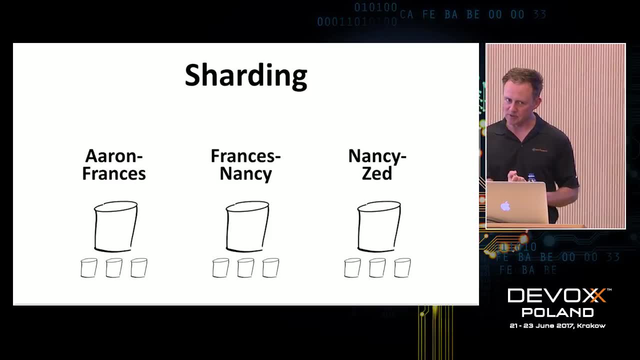 database. That's how you can make it get a little bit bigger Again. the bad thing is certain behaviors and guarantees and claims of a relational database that I start off with. little by little I give those up. In fact it's even. 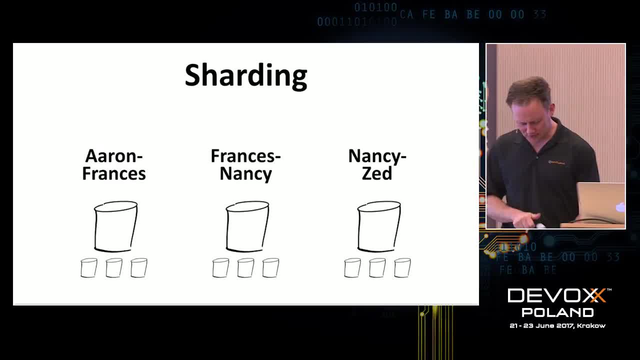 a little worse than that. There are other things. If you can imagine that scale slider going up and up, I have to do things with the topology to address that. I have to add computers and make a distributed system. I'll also have to take things away from my data model as I turn that slider up. 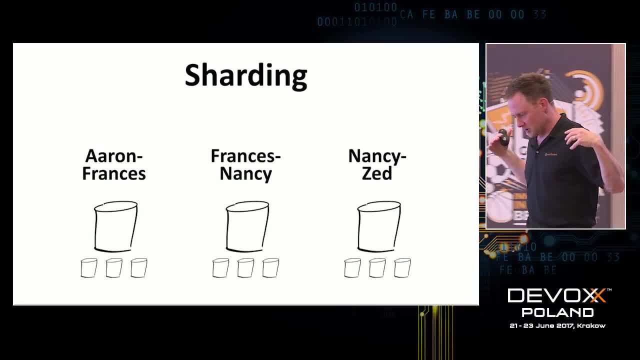 Suppose, for example, your database comes under pressure, latency is going up, you're having higher transactional volume and suddenly reads are not performing properly. What are you going to do? What's the force? What are you going to do? What are you going to do? 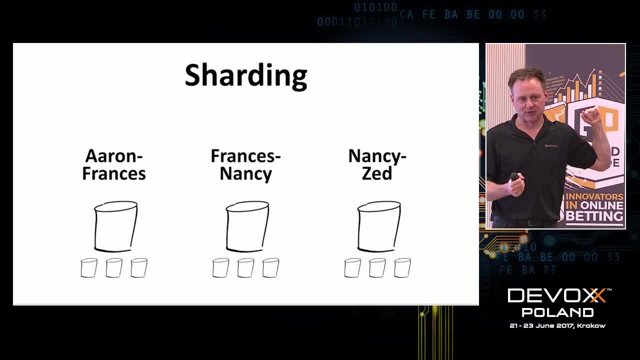 I have to make my data model and I have to make my database. What are you going to do? One of the first things you'll do in response to that, Most people will say at this point: add an index. Kind of an okay answer, right? 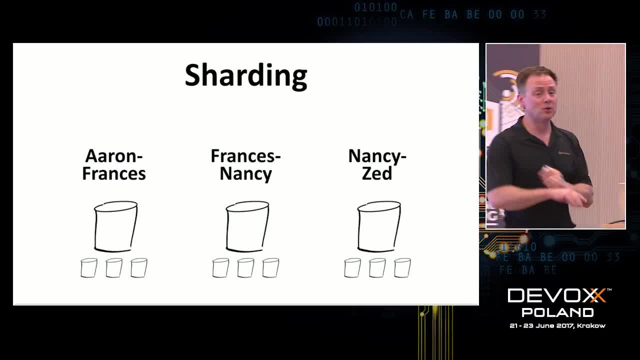 Maybe that'll help. Maybe you're missing an index. That's good, Suppose you've already done all the index optimizing you can. That's trivial After that. what you do is you realize, oh wait, The reason reads are slow is because of this wonderful relational model. 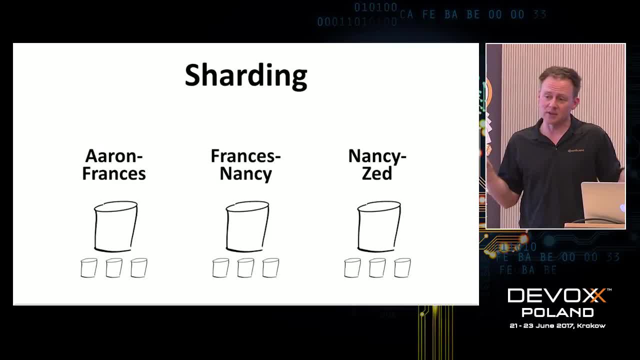 I'm doing all this joining because my schema is properly normalized. I have to take joins away in order to make reads perform. And how do you take joins away? Well, you denormalize, which we all know is immoral. right? That's what we're taught in school. 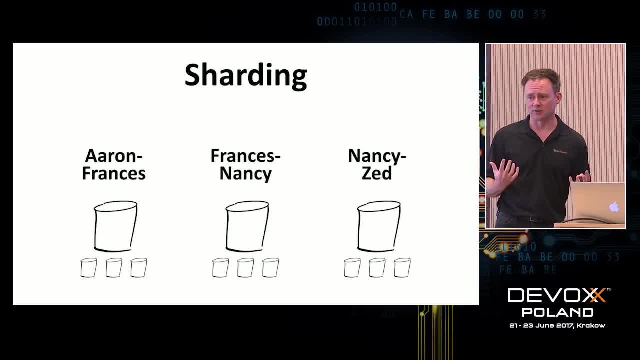 So you actually become what you think is a terrible person and you denormalize because your scale is forcing you. You have no choice. Also, if your first answer was to add indexes, that is another pressure that you'll come under on the right side. 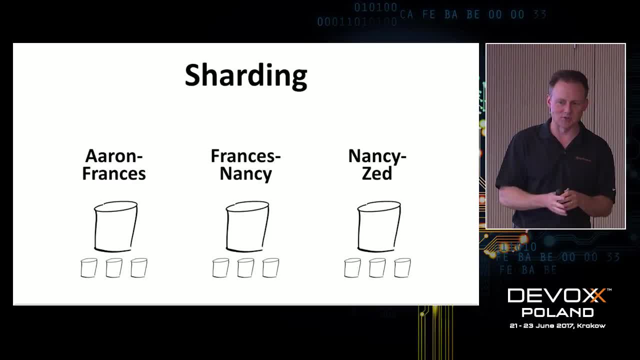 As write, traffic increases before you shard, or even after you shard, you're likely to give up on indexes, which will then have further pressure on you denormalizing your data model down the line. So all of the wonderful things that you thought were true about your database when you started. 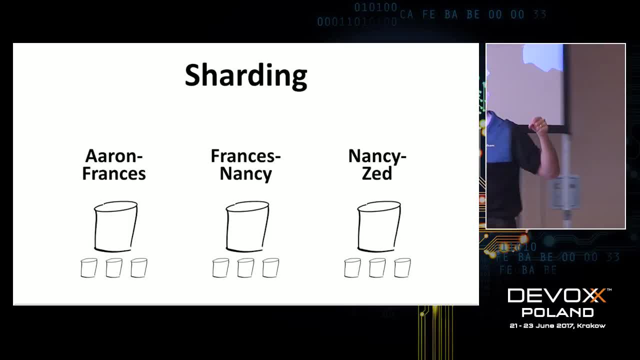 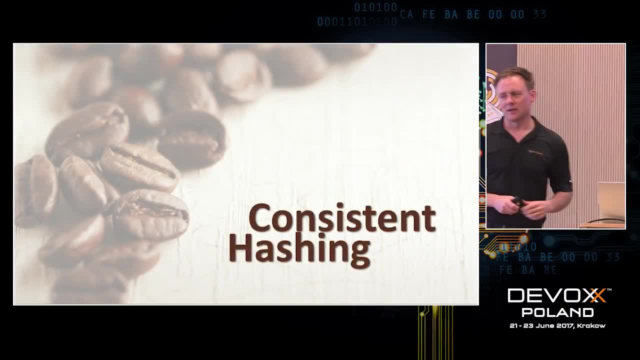 they're just gone, They're taken away from you by the time. you have to scale it and you end up with something that doesn't really look all that relational by the time you're done. So why not just do it right? And here is an approach that is taken by 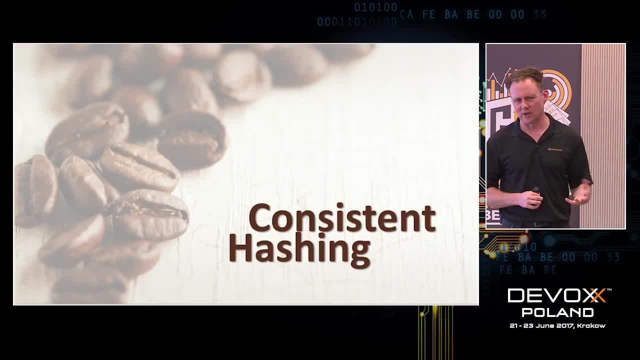 really I'll be talking in terms of Cassandra, because it's a database that I know fairly well. but this is sort of: if you look at the scalable non-relational databases, that family of products, they all kind of work like this: 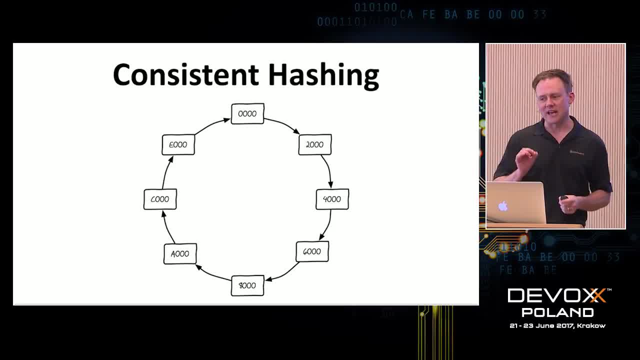 They use a technique called consistent hashing. In fact, consistent hashing is a nice thing to know when you're looking at other systems and other open source projects in the distributed systems world. This method is often kind of pokes up its head and is like winking at you from various systems. 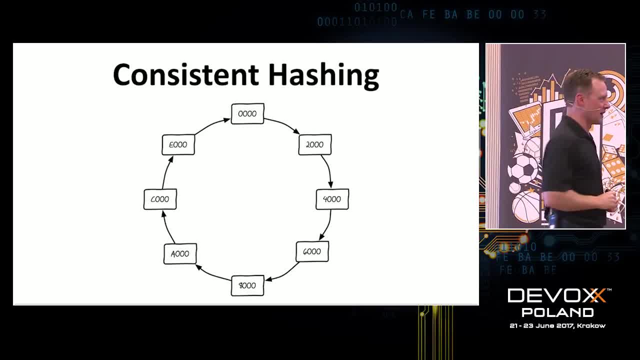 It's front and center in Cassandra, but it shows up in other places, so just be advised. Now here's an example of how you build a database from the ground up to be distributed. Now it's still doing bad things to you all, right. 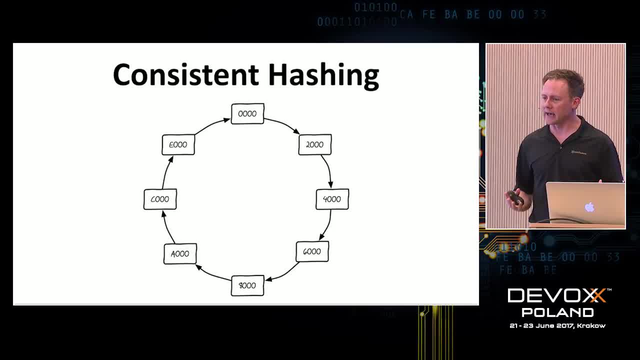 There's still lots of features. Cassandra is not going to give you that you wish you had, but it's very upfront about it, right, Right from the beginning. it's saying: here are the limitations of the data model. Here's how scale works period. 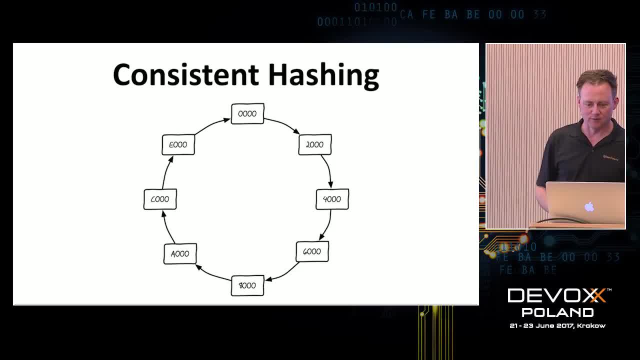 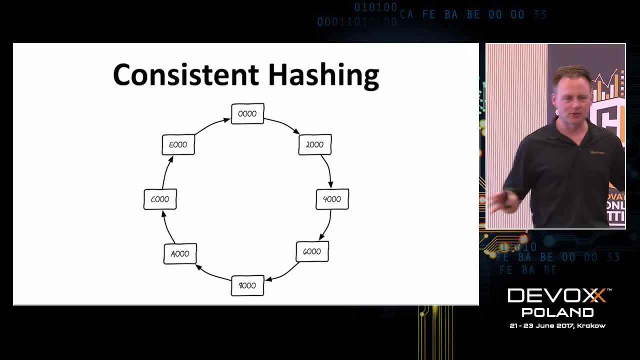 And sort of I'll just deal with it and move forward from there. So suppose I've got this database here. I've got eight computers and they're all the same, They're all peers. It's a pretty simple architecture. 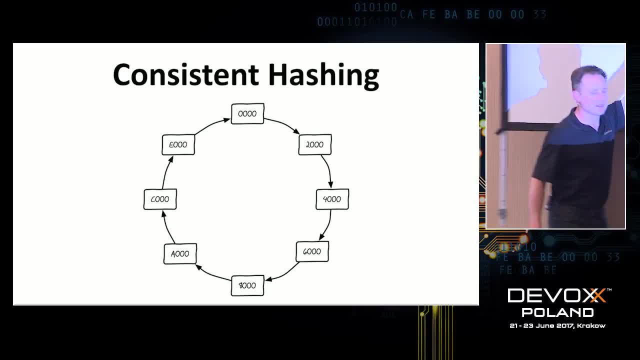 They're just identified with a numeric token, And in the case of Cassandra, we always draw this in a circle. Now, that's not because they're actually connected that way. You know, these are regular computers on an Ethernet network, just like you are, a normal person. 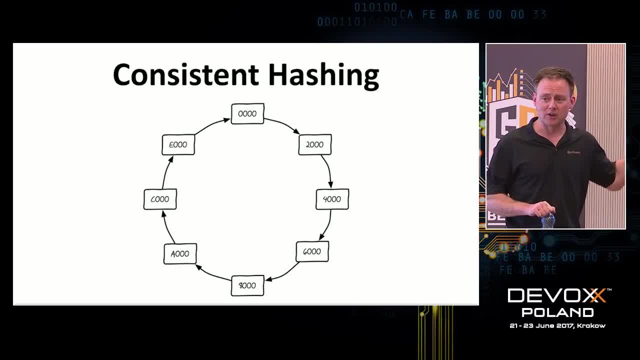 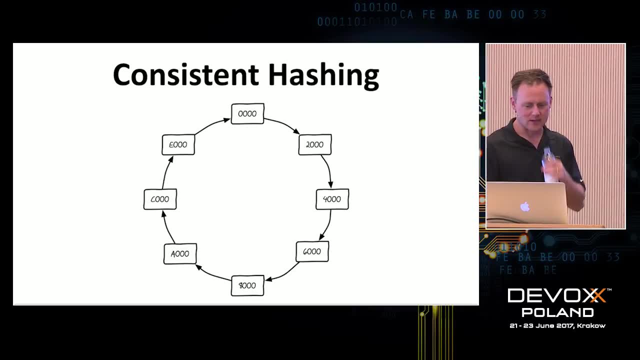 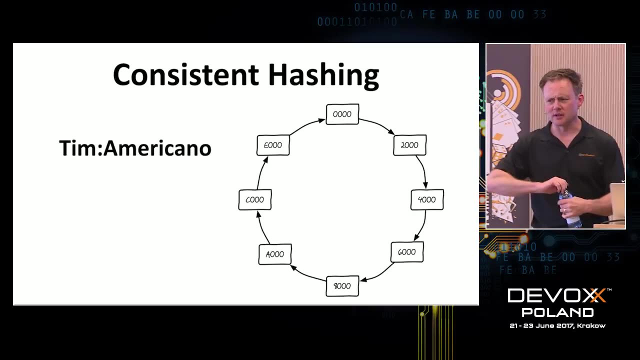 But they all have this unique token, this unique numerical ID, and it helps to draw them in order, clockwise, in a circle. And I'll show you why. right now I'm storing favorites and per the coffee picture. I forgot to say this at the opening slide. 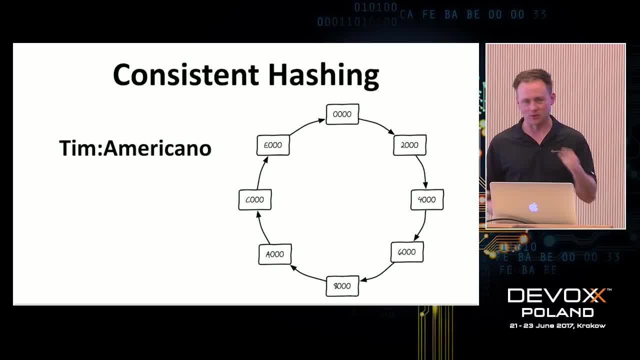 As many of these examples as possible I will draw from a coffee shop just to be cute. So suppose this web-scale coffee shop is trying to remember people's favorite coffee. Basically I'm an Americano guy. Sometimes if I'm feeling a little crazy. 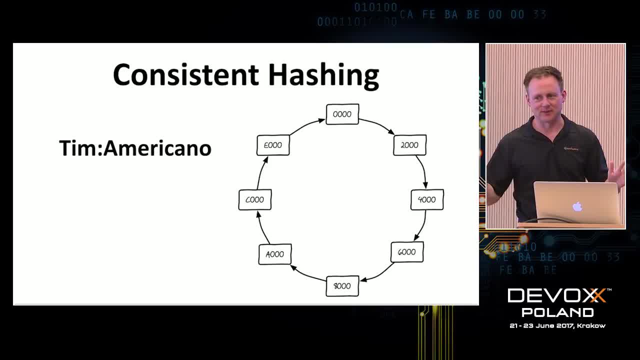 I'll have a crazy almond milk latte. That's about as fancy as it gets, But we want to store my favorite coffee, Americano. What we do is we take that key-value pair. Cassandra is not a key-value database, but this is an easy abstraction to kind of get on board. 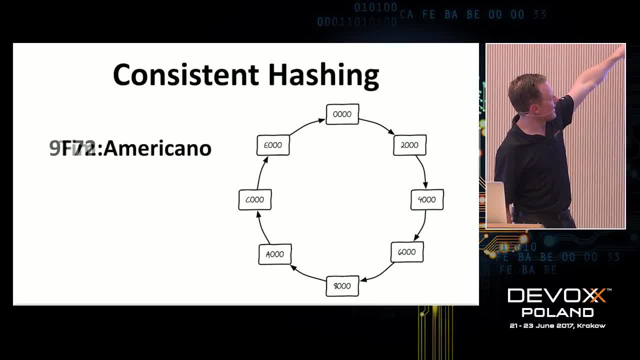 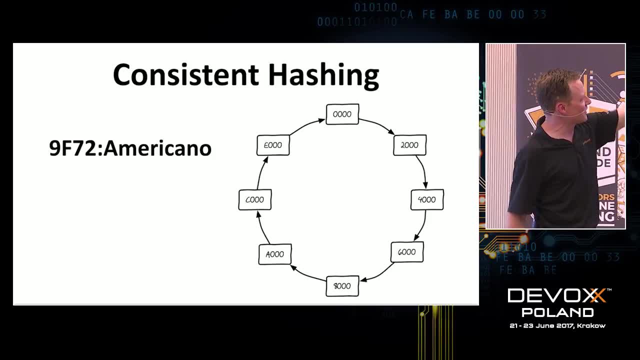 And this is as far as we'll go here in this summary. Take the key and run it through a hash function. Doesn't matter what the hash function is, as long as it's always the same hash function, We hash it and we say, okay, where is that number going to fit in this ring? 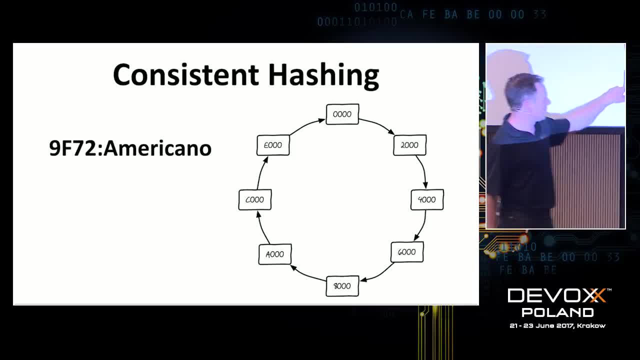 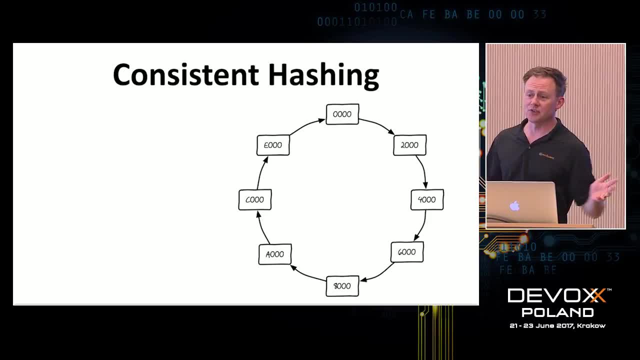 We want to see Bigger than 8,000, it's less than 8,000.. So just based on the way those arrows are going, I'm going to write that key into that node. Simple as that. Now the cluster can grow, the hash values can change. 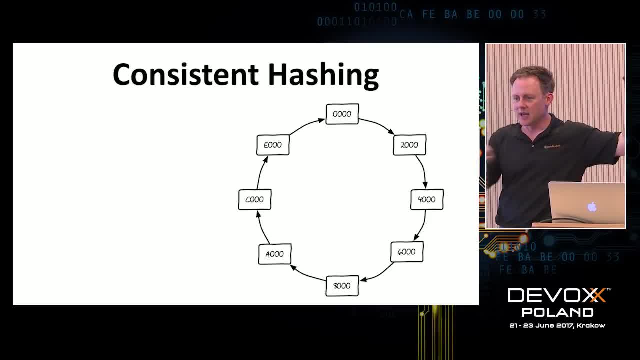 and as long as, internally, the database moves keys around. as those things change, all I ever need to do when I'm writing to the database is look at it and see what are your tokens right now. How many nodes do you have? 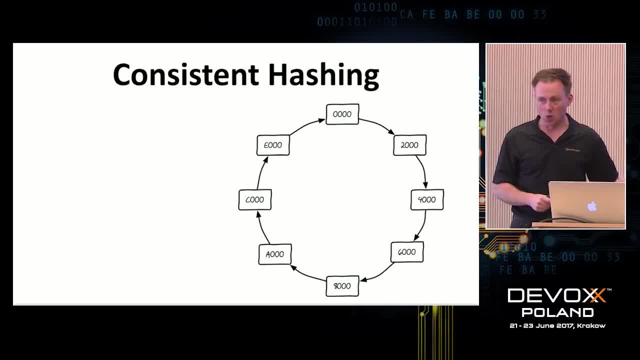 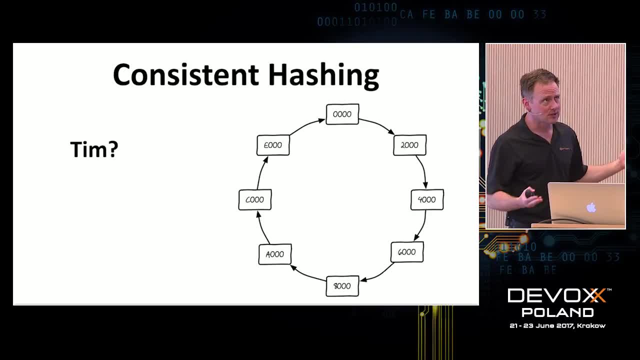 What are your tokens? And hash my key and I know where to write And I know where to read from Later on. if I say, hey, what's Tim's favorite coffee? There's a new barista. He doesn't know what my favorite coffee is. 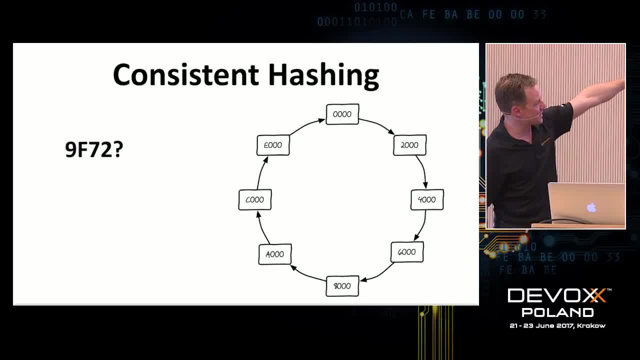 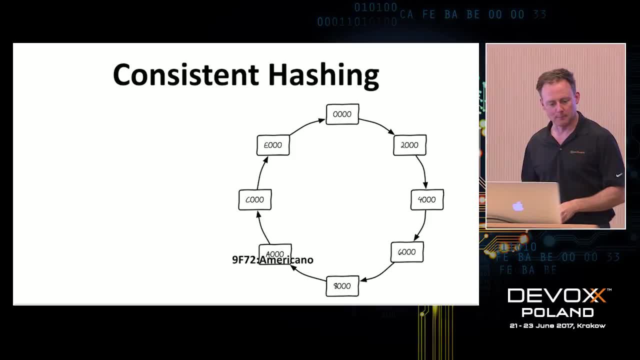 It's fine, This is web scale. He can't remember all those things. We'll hash that. We'll say, oh, 9F72.. Fine, That's going to come from 8,000.. I'll go there, get that key and pull it out. 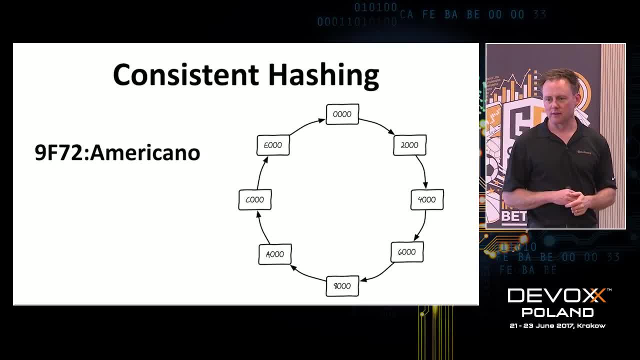 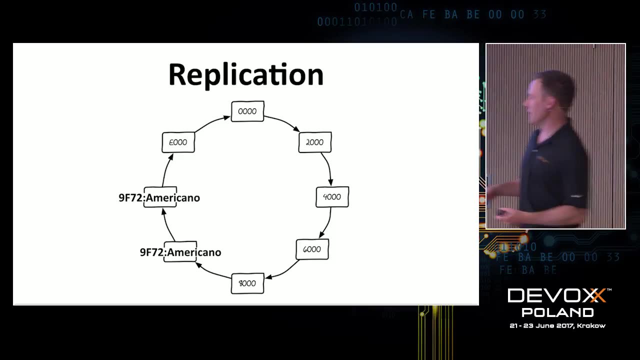 So that's basically how you read and write with a consistently hashed database. Of course we would never want to have just one copy of a piece of data, That would be crazy. So we can do things like replicate. If I say, well, the first copy would have gone to this node. 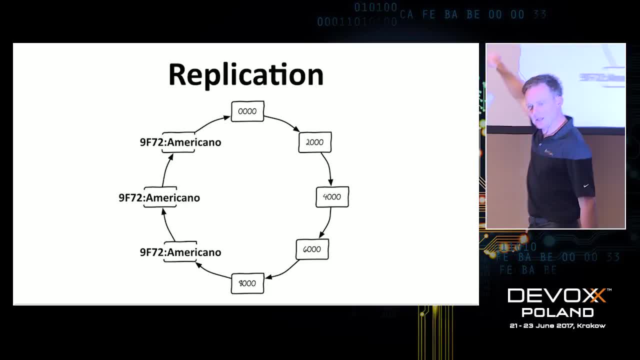 I'll just go to the next two nodes down the ring in the cluster and put a copy on those nodes as well. That fixes the problem of now that I'm in a distributed system. what was my second characteristic? Computers fail independently. We know this. 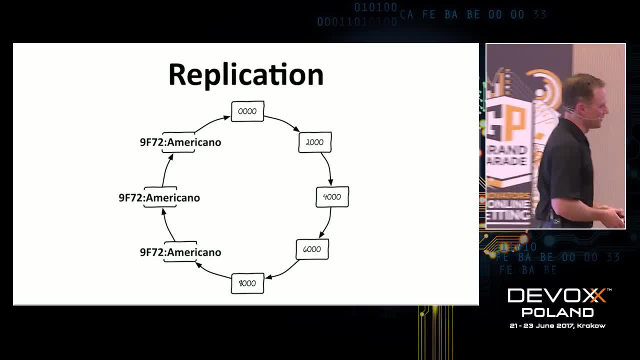 There's no way to predict when a node's going to die. I would never want a key in just one place, So now I've got three copies of it. I've solved that problem. I'm now able to tolerate hardware failure and be up. 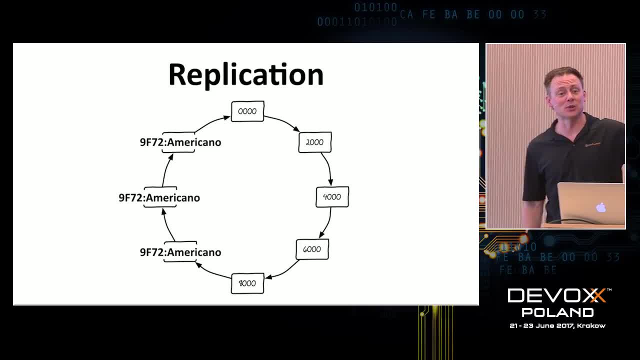 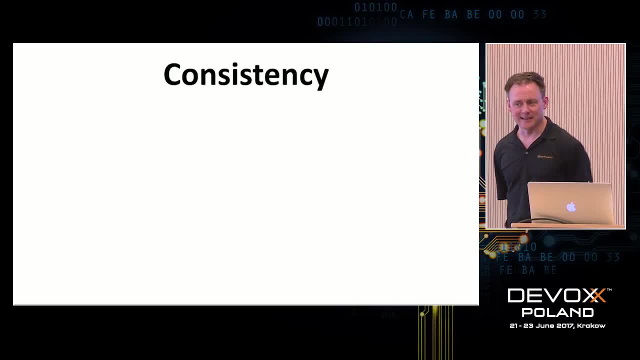 Sounds great. I told you distributed systems are terrible. I created a problem by solving one. And what is that problem? Consistency. I have three copies on three computers of something that can change. I'm a fickle coffee drinker. It's Americano today, tomorrow maybe it's triple skinny. 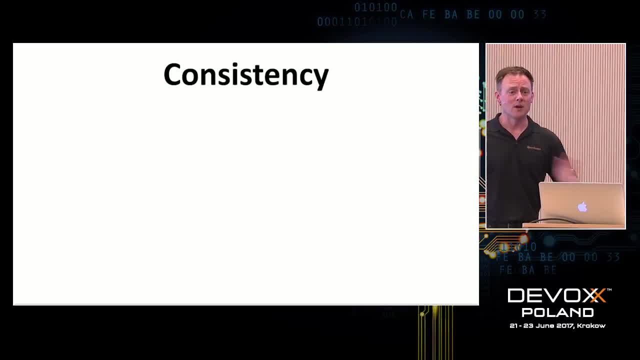 two-thirds decaf, half chocolate, no whip, grande mocha with extra foam. You have no idea what I might come up with tomorrow. I am the very definition of mutable state. So now that I have three copies of something that can change, 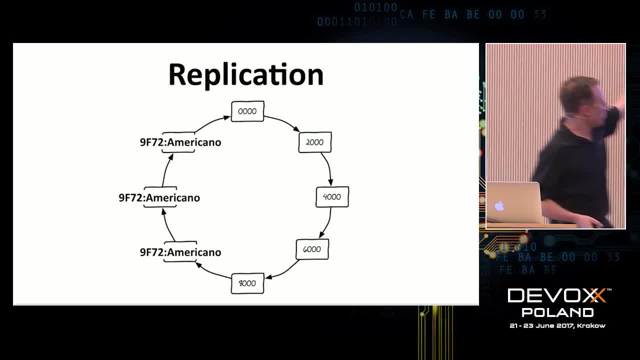 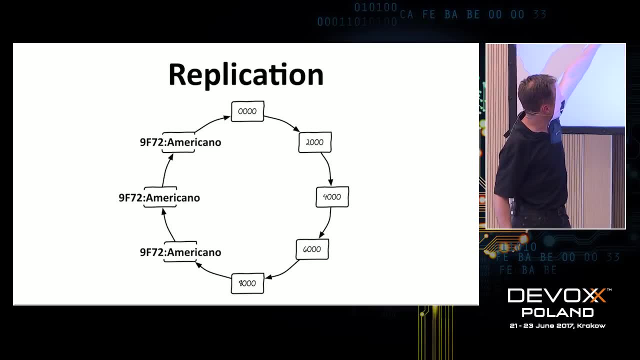 I have created a consistency problem And, to be clear, one of these: if I write tomorrow my new, that crazy thing I just said, maybe one of these nodes is down while I'm doing the write And it doesn't succeed and it has an old copy of the favorite coffee. 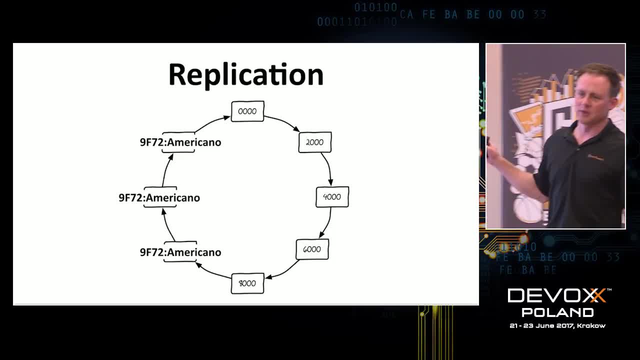 and the other two nodes have the new copy, Entirely possible. And then when I go to read, how do I know who's telling the truth? All of these things become problems. Now, basically, I want to give you a rule for thinking about consistency. in a database like this, When I write to the database, I'm going to require that a certain number of nodes take the write. So as a client, as a client application, I'm going to say: you two, at least two of you, need to succeed. 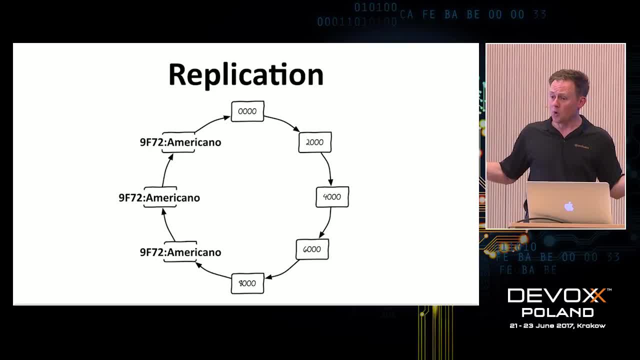 If only one of you succeeds, I'm going to consider it to be a failure. Or I'll say only one of you needs to succeed. I know I have three replicas, but I'm in a hurry I'll take one. Those are options that I have. 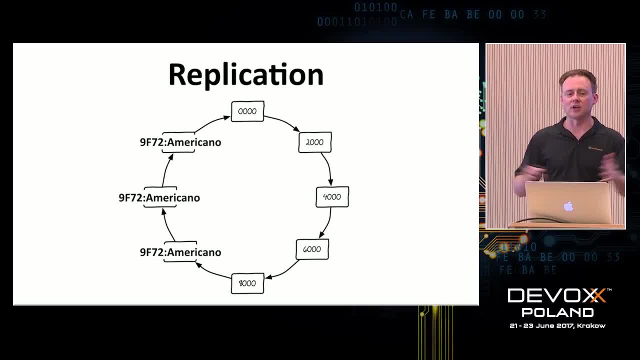 I could be particularly fastidious and say I need all three of you to succeed. Nobody would do that Really. just one and two are the practical options. Likewise, when I read, I need to say: well, I'm going to hear from two of you or one of you. 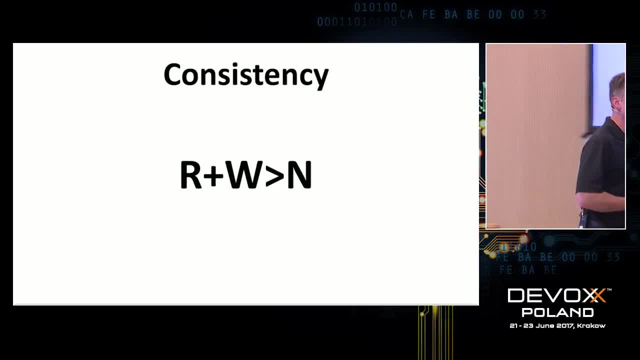 I have a simple formula here for knowing whether you are using your database in a strongly consistent way. If the number of nodes I write plus the number of nodes I read is greater than the number of replicas, then I have strong consistency. So if I write one and read one and there's three replicas, 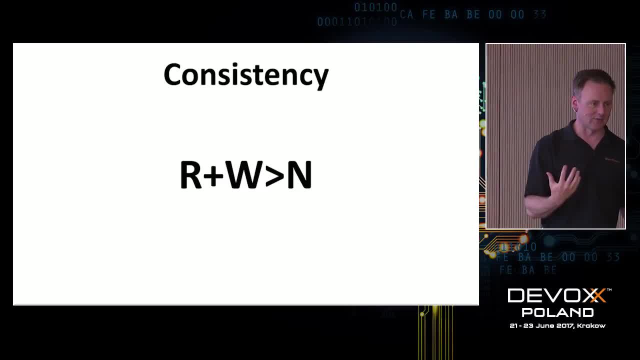 that's eventually consistent. If I write two and read two and I have three replicas, that's strongly consistent. Cassandra is a pretty cool database. If you want a big database, it's kind of the way to go, And it lets you tune this on a request-by-request basis. 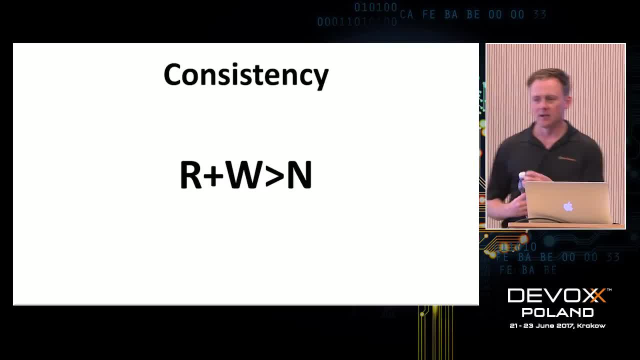 You can change your consistency semantics on the fly- Pretty cool. So even though everything's a problem in a distributed system and solving one problem creates another one, there are some things that have elegant answers, And Cassandra is one such: The CAP theorem. Should we talk about the CAP theorem? 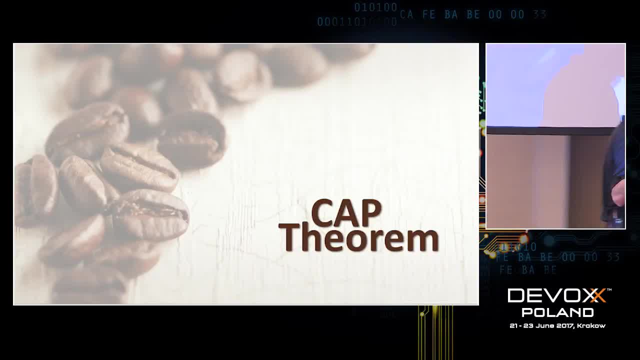 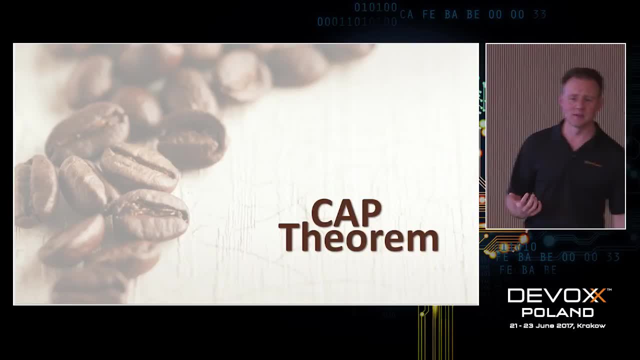 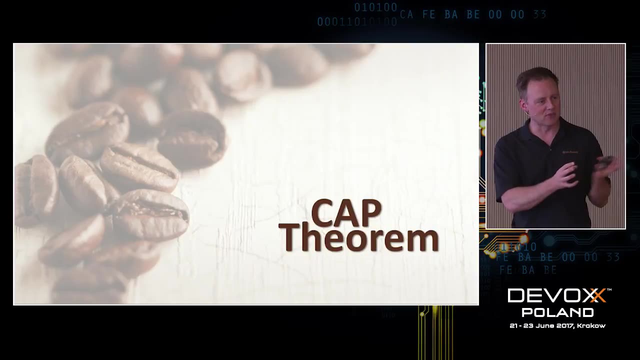 Just a tiny bit Back when NoSQL was new. it was like 2010,. reading Hacker News in the morning, which is a thing I do, it's like my newspaper. it was painful because about once a week there would be a new and newly misinformed blog post. 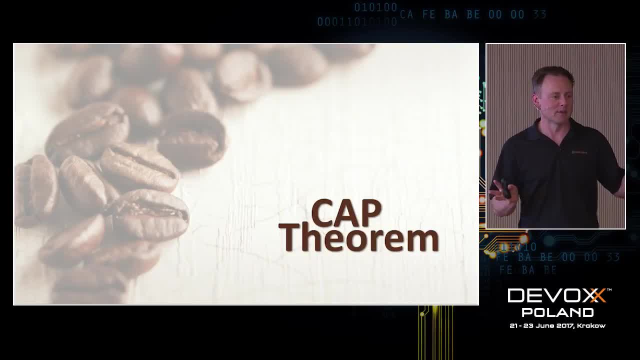 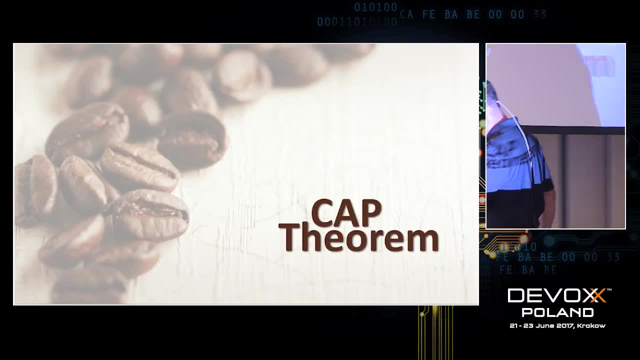 that would make it to the front page of Hacker News. that was something about the CAP theorem: Everybody cared all of a sudden because everybody was making scalable databases and so people had to blog about it and say things that weren't true. It's really not hard to grasp. 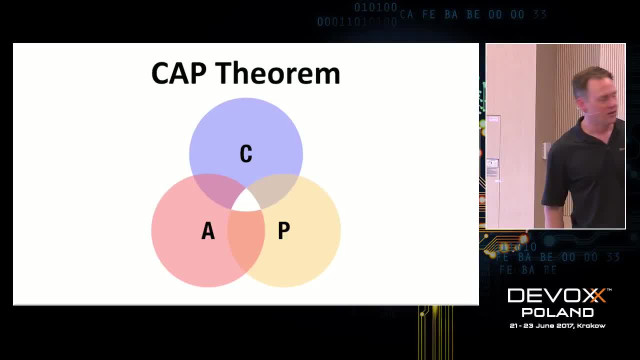 and it comes up sometimes still in distributed systems discussions. so I want to give you a simple way of understanding it. The CAP theorem says: if you're building- let's just make it simple- a distributed database. you want your database to have three properties. 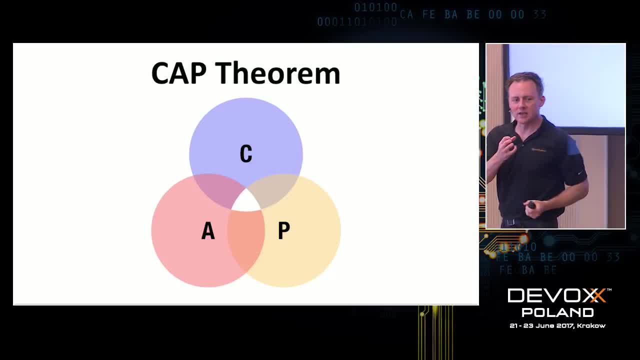 You want it to be consistent. that is. that's the C. if I read something, I want that to be the most recent thing I've written. So I write and then I read, and I see what I read. I want it to be available, and that simply means. 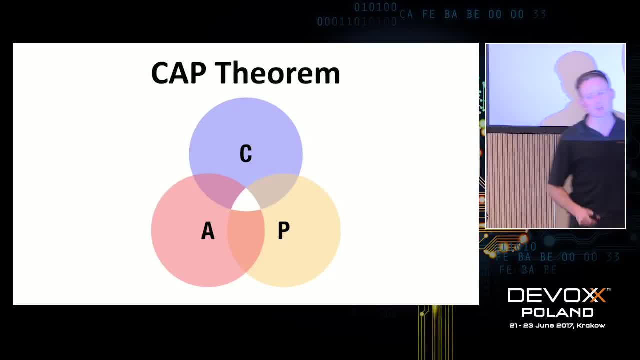 when I try to write it works, and when I try to read it works. I also want it to be partition tolerant. That means it's a cluster. I've got lots of nodes being a database together and if some of those nodes go away for a little bit, 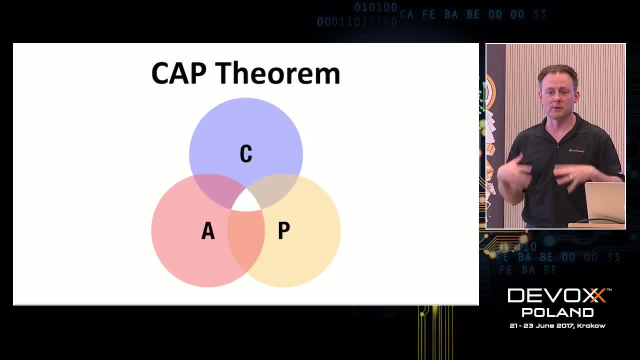 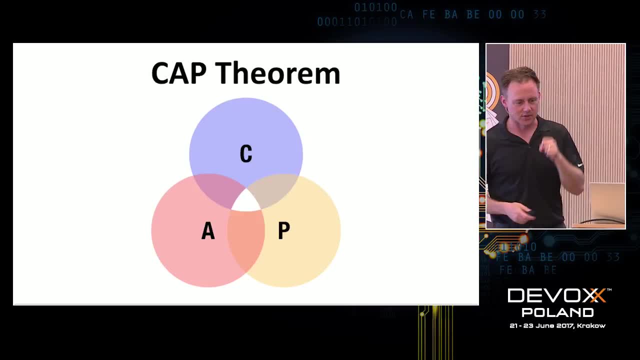 and then come back together. I don't want the database to completely fall apart. I want it to be able to deal with the fact that sometimes parts of the system can't talk to the rest of the system. that's partition tolerance. So imagine if you would. you're in a coffee shop. 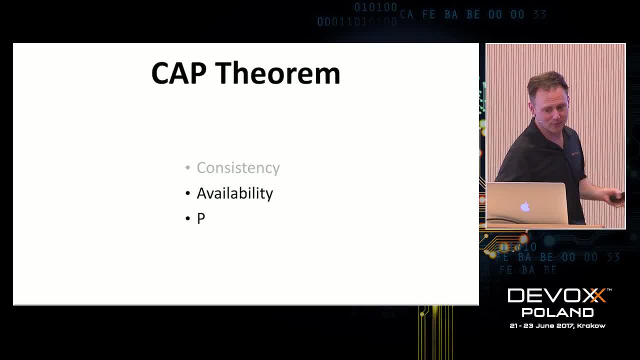 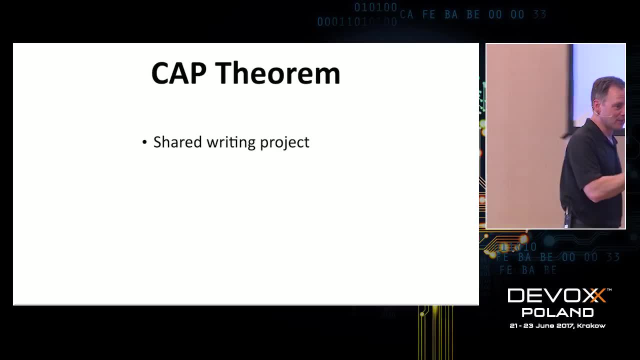 like I said, we're- oh wait, I forgot this slide- consistency, availability, partition, tolerance- you guys got this All right. imagine you're in a coffee shop, forget about databases for a minute and you are writing something together. 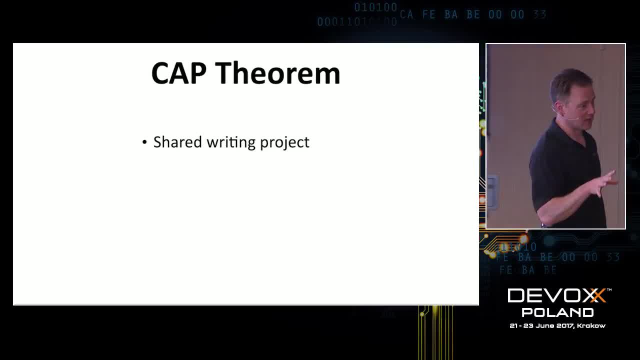 You're working on your screenplay with a friend, your co-writer, And you're old school, so you're doing it on a yellow legal pad with a pen. It's you, it's not me. I don't know why you're doing this this way, but you are. 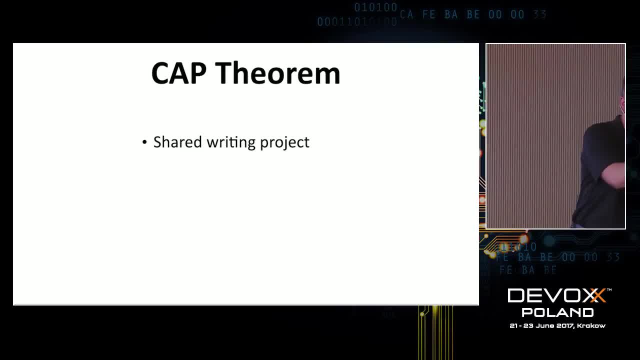 And both of you have a copy of the screenplay. One of you makes a change here, the other one makes a change on their copy. That person makes a change. you delete something. you keep your copies consistent because it's how you want to do it. 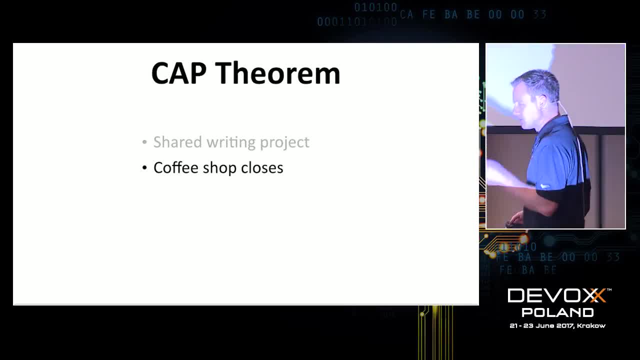 It's a little strange, but it's what you're doing: The coffee shop closes. I'm not going to judge you. I don't know why you're doing it this way, but you just are. Coffee shop closes, but you're in the zone. 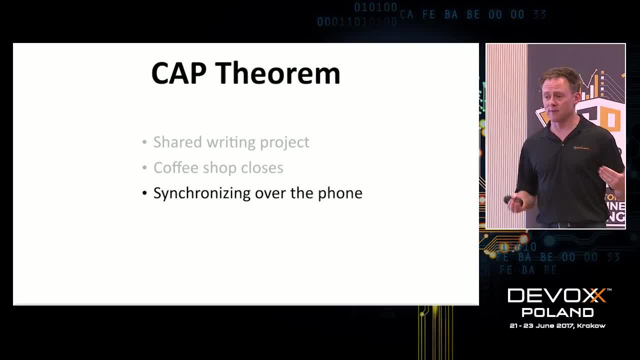 so you go home and you keep going over the phone and you keep in sync over the phone. You say, well, I added this line of dialogue, I removed this scene. here you're heading and you're keeping things up to date. 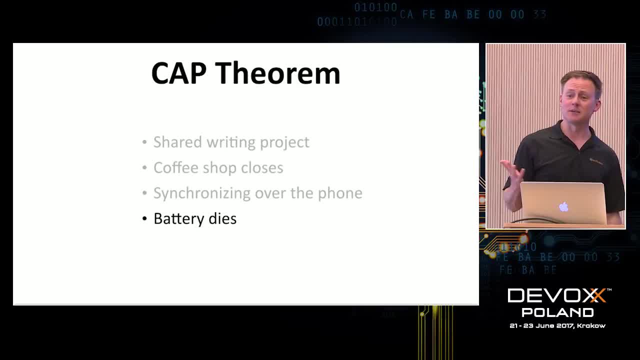 But then your battery dies and you can't talk anymore. You lost your charger. you now have a network partition. You keep writing because you're in the zone. presumably your partner keeps writing. Your spouse comes in the room and says: 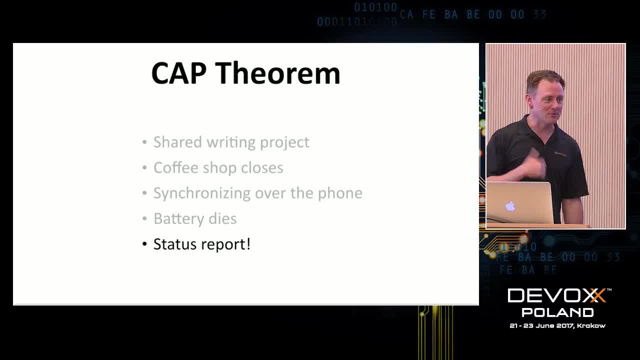 hey, how's the screenplay going? Read me back your most recent page, Which is great that your spouse is so interested. I think Here we have a decision. So back to the event. You can't have all three of these things. 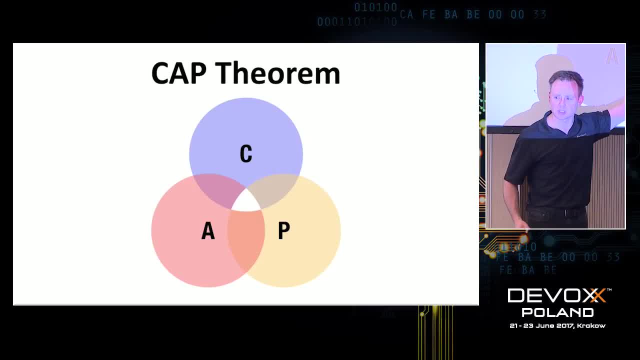 That's the fundamental insight of the CAP theorem In the presence of a partition. in this situation, you can either choose to be unavailable, that is, you say to your spouse: I can't tell you because I might tell you the wrong thing. 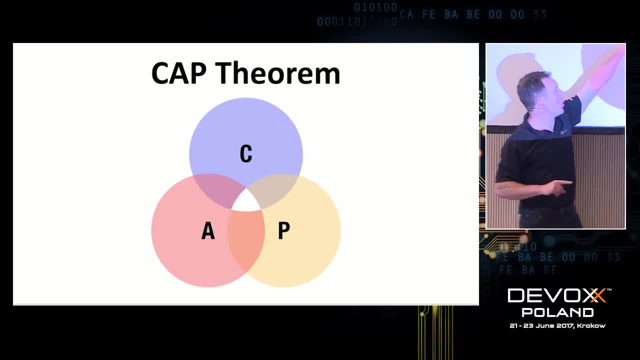 and I would hate to do that. That would be unfair to my writing partner. Or you could say: well, I'll just give you an answer. It might be wrong, So I could give up on availability and keep consistency by not answering. 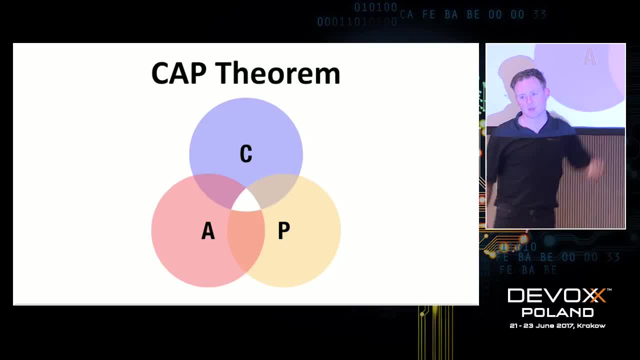 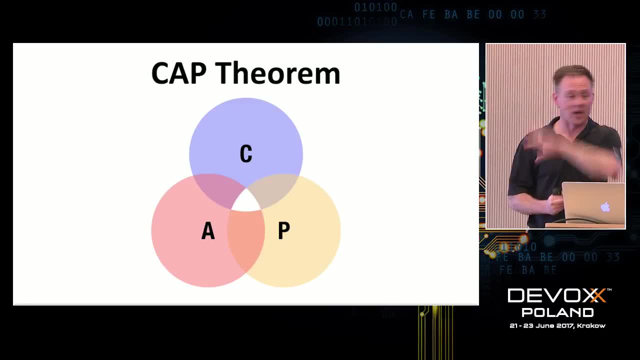 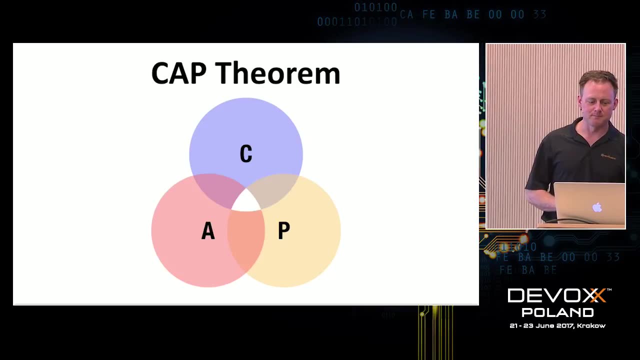 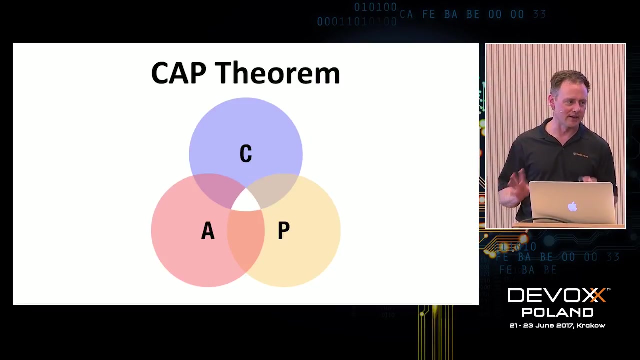 Or I could keep availability and give up on consistency. That's the fundamental insight of the CAP. theorem is: I can only have two of these three good things. I always want all three, But sometimes I can't have all three. It's again. there's a lot of writing on the internet. 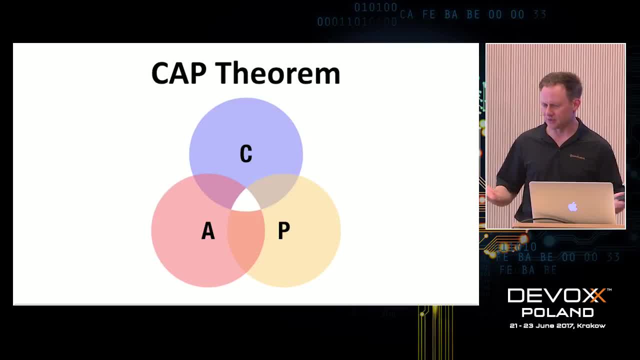 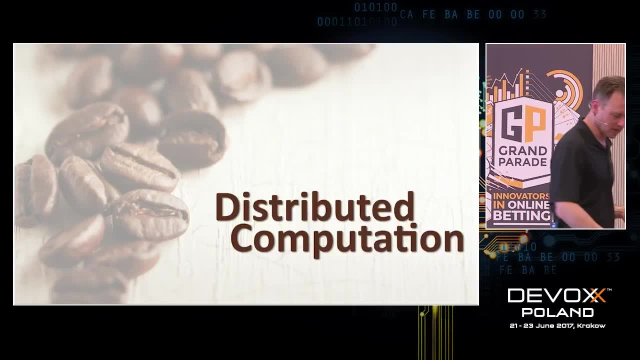 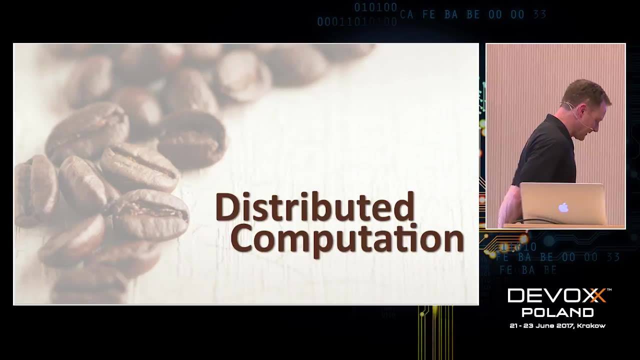 about what this means and what its implications are, and when it applies, and so forth. But just think of distributed databases. It's a simple trade-off between those three things that you want. All right, Enough of storage. Let's talk about computation. 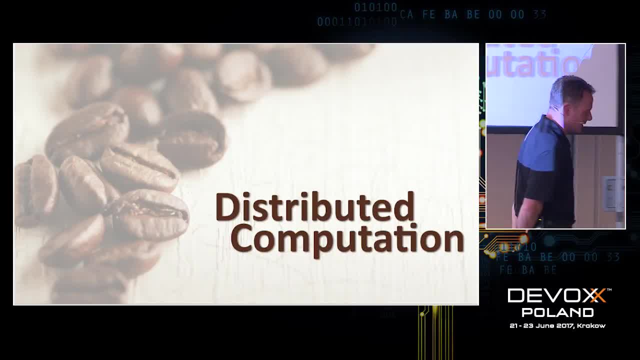 Again, computation is super easy if you have just one processor. If you go to multiple threads on one processor and you try to do computation in a threaded way, that's usually pretty terrible And there are talks at this conference about ways to avoid that terribleness. 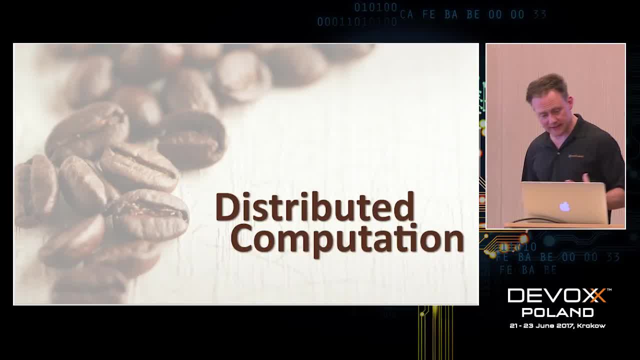 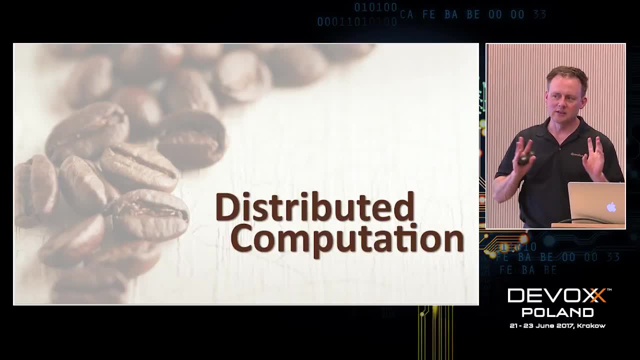 And I should say: but you got multiple computers and you're trying to distribute a computation task among multiple computers. life gets really hard And we've created some truly terrible tools for solving this problem. The good news is, life is getting a lot better. 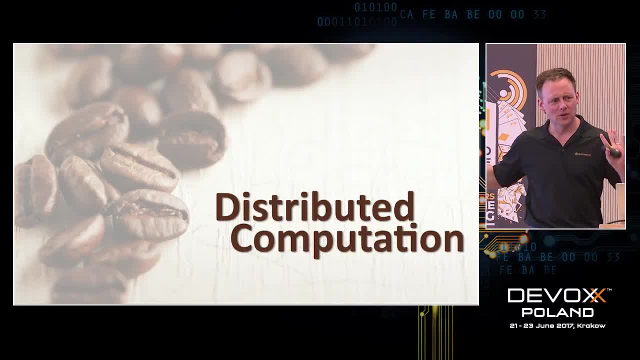 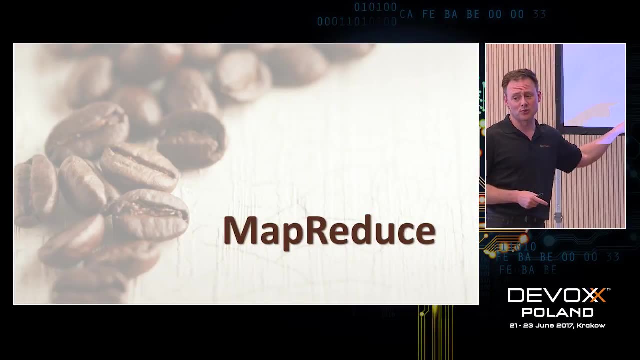 Trying to do this 10 years ago or 12 years ago was bad. Trying to do it now is starting to not feel like somebody is hitting you with a 2x4. So I think there's a lot of reason for optimism, And MapReduce is not one of those reasons. 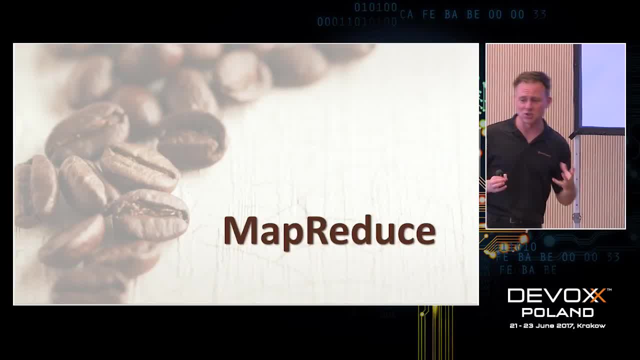 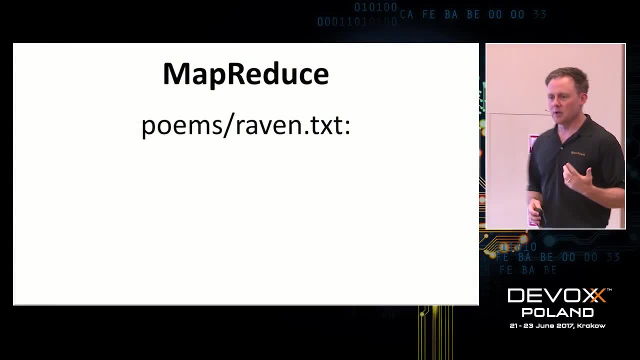 But let's talk about it just to make sure we're on the same page, and you know the badness that we've come from. So the typical way to explain MapReduce is with word count. And this is a union rule. people, I have to do this. 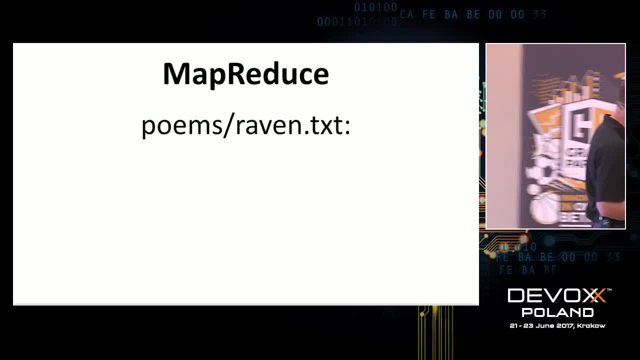 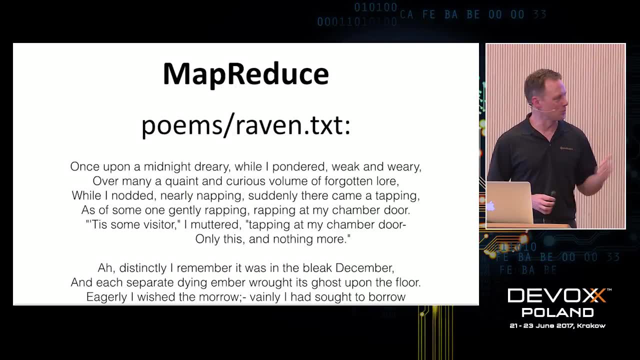 So I'm going to use a word count example just to show you basically what's going on here. So I've got this big table, I've got this big chunk of text. Now, if I'm actually- oh, this works really well in the US. 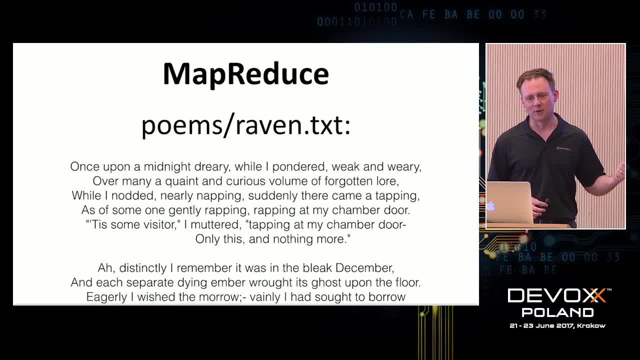 because everybody knows this. It's an American poet. He's from Baltimore. His name is Edgar Allan Poe. The American football team from Baltimore. Does anybody know the name of the team? The Ravens? because this poet is from Baltimore. This is his most favorite poem. 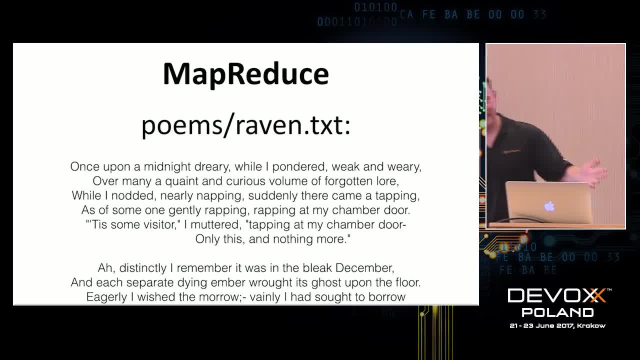 It's an amazing poem, strongly recommended, And I'm not even a football fan, But I kind of love the Ravens for this reason. Anyway, if you actually had the text of the Raven, I think it's about 1,800 words, the right way to count that. 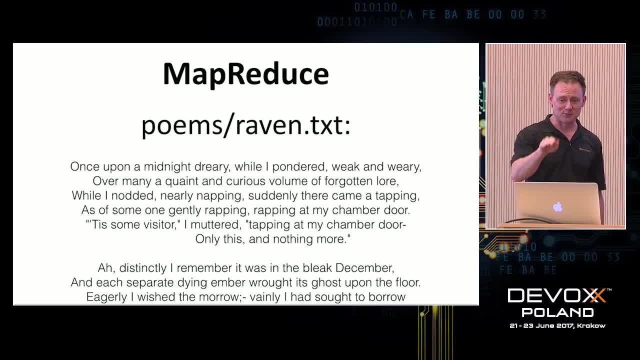 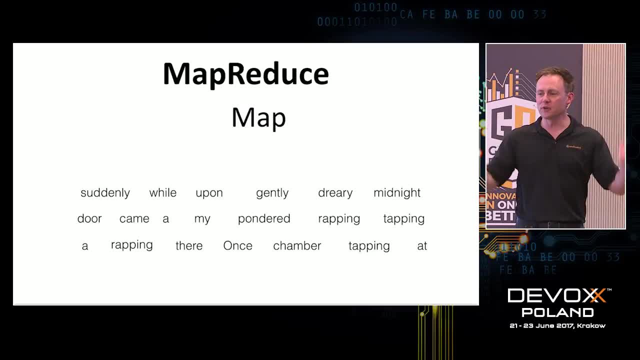 is to use the WC command. Don't screw around. That's a small data problem, But this is helpful just to see how MapReduce works. MapReduce funnels all of your computation through two functions, one called map and one called reduce. 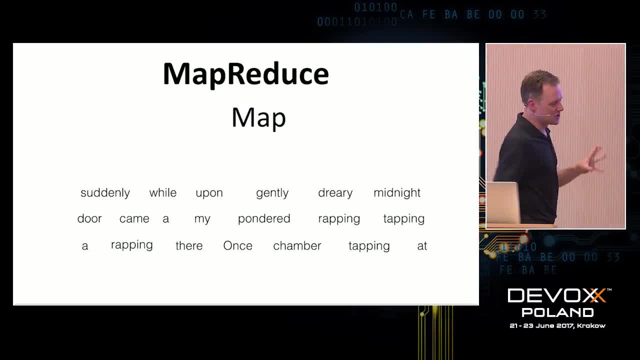 That is a terrible thing to do to a person, But here's how it works. I would dump the text into my map function And what map would do is it would tokenize it, It would split it up into words And then it would turn those words into key value pairs. 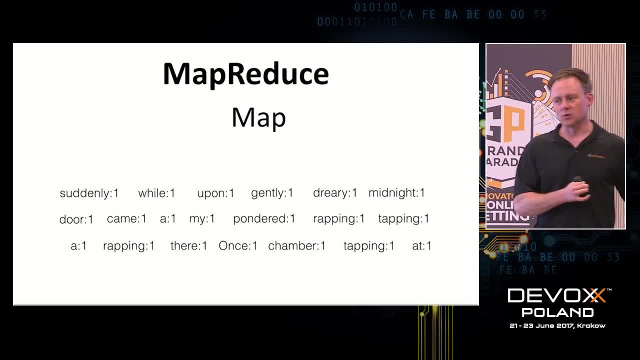 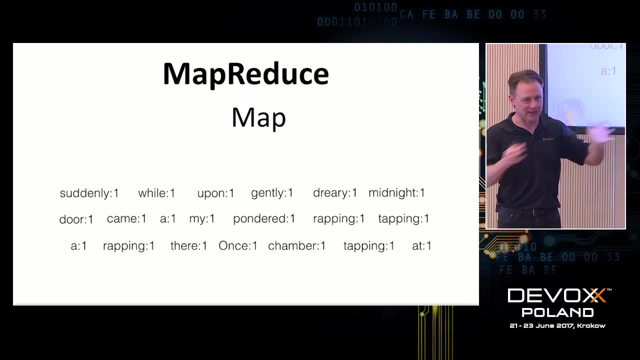 I like to go through this because this is kind of a neat insight into the way you would solve a problem like this in a distributed way. What we begin by doing is counting words. That is what I have just done here. That's the first step in the MapReduce canonical. 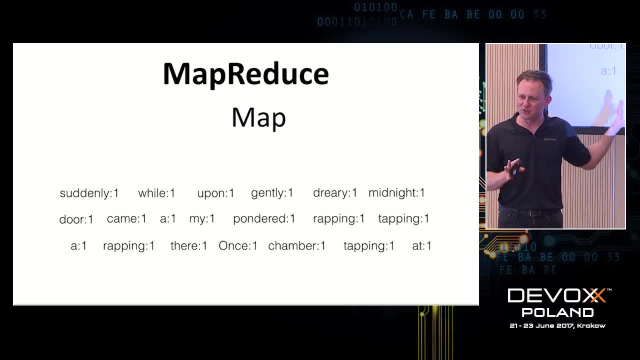 MapReduce. word count example is: you count the words. Now, what people say is: I tokenize the text and I turn the words into key value pairs. The word is the key and the value is the number one. Really, what I have done, though, is I've just counted each word. 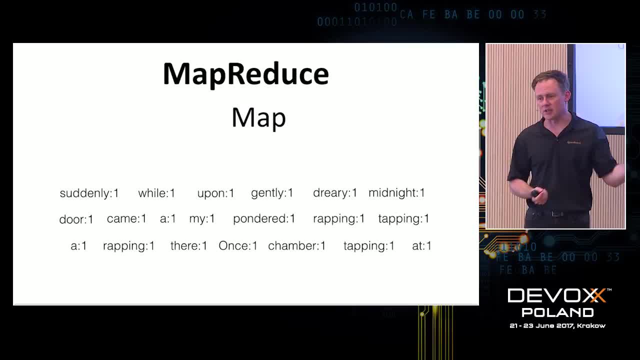 And I've seen each word one time. It's like very naive, stateless counting. I don't remember whether I've seen the word A or came or wrapping before, I just count each one one time. Then there is a step in between that always gets ignored. 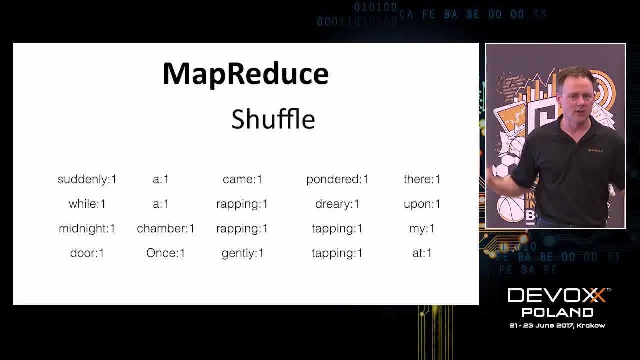 It's called shuffle. So after I do that mapping I count all my words once. Then potentially I have to move these words around the network to different computers to make sure similar words are nearby each other. So at, or rather A wrapping tapping. 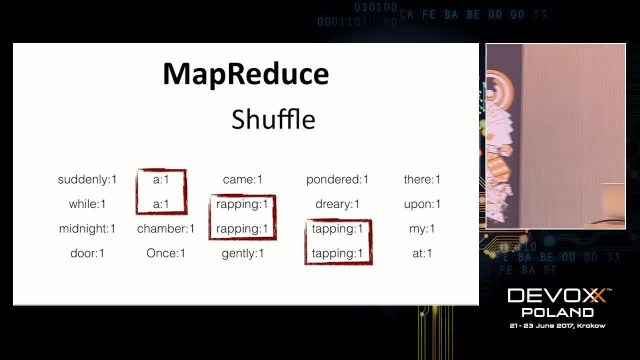 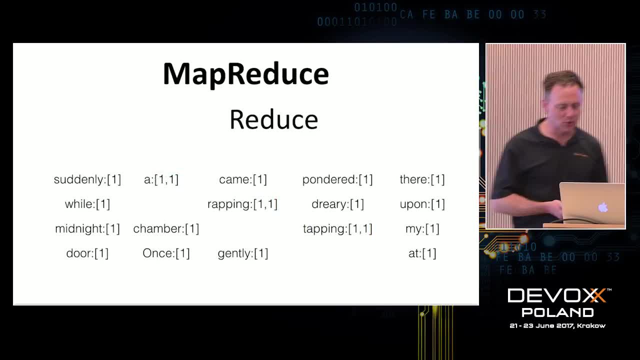 I want to get those in order. Then I take these collections of similar words and I dump them into a function called reduce, And what reduce is going to do is basically add up the numbers. So it's a less naive counter. It says: well, I counted the word A 3,000 times. 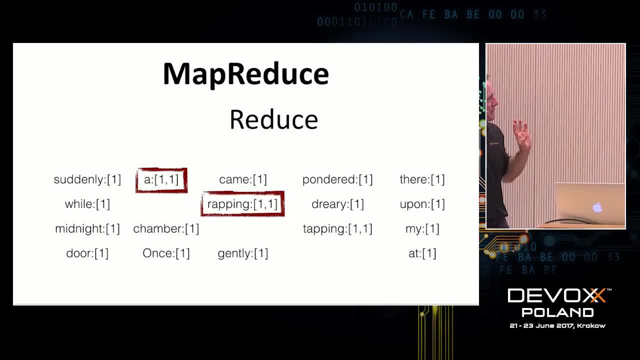 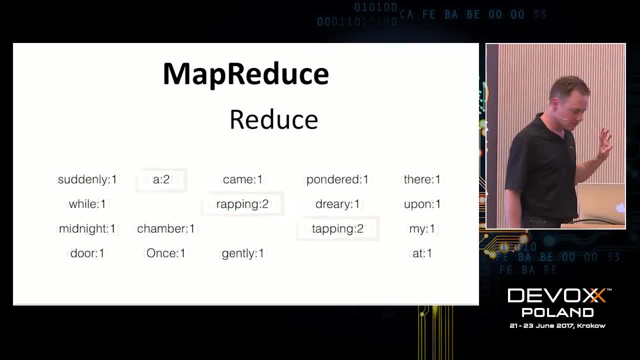 Let me just add up all those numbers Now. I am skipping a bunch of steps here in the spirit of summary and a bunch of complexity here in the spirit of summary, But I end up with counted words And I'm able to do this. 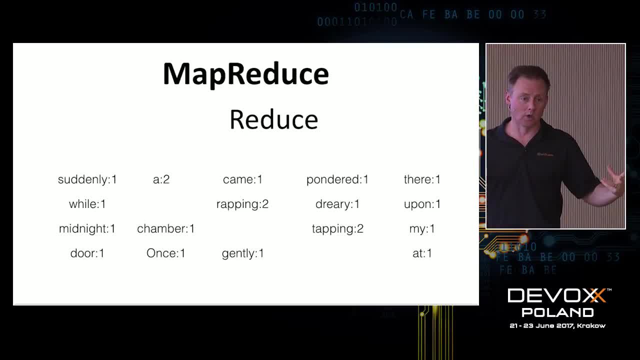 I'm able to split up the work of mapping and the work of reducing and distribute it among lots and lots of computers. This is a really good idea if your data is already, say, in a distributed file system. If you've got so much data that you need 300 computers. 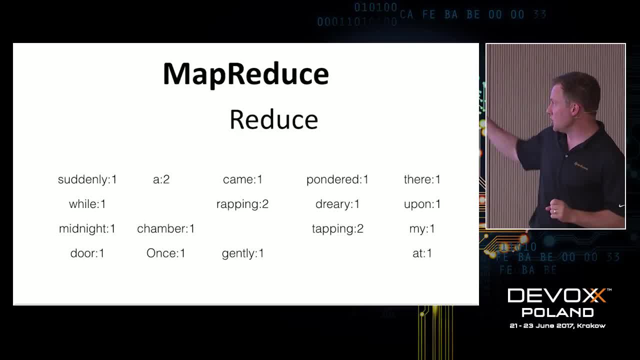 to store it all and replicate it all, then doing your compute this way. it seemed like a good idea at the time And it was a moderately good idea. A lot of people built- I shouldn't say a lot. some people built systems using MapReduce. 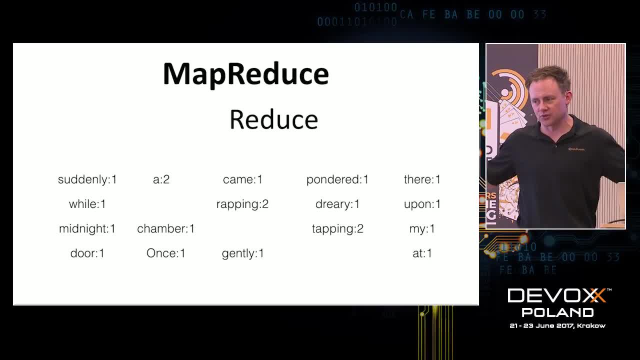 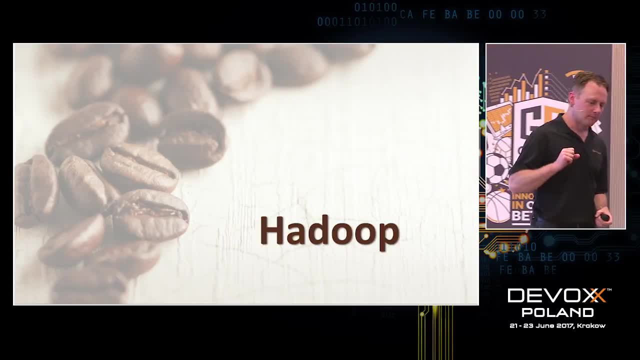 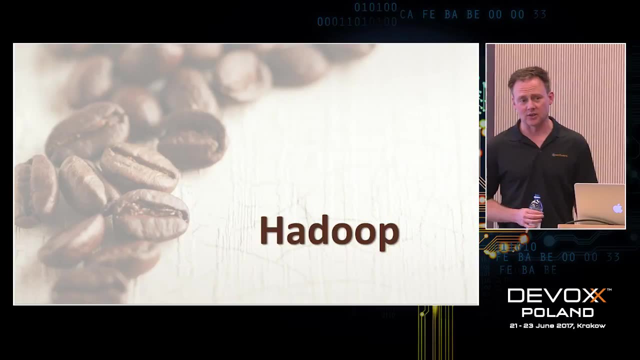 that were worthwhile, all right, And it by itself, MapReduce is just a pattern. it's not a product, But it's the pattern, the compute pattern used by Hadoop. Hadoop is still widely deployed, rapidly becoming, in my view and the view of many others, a legacy technology. 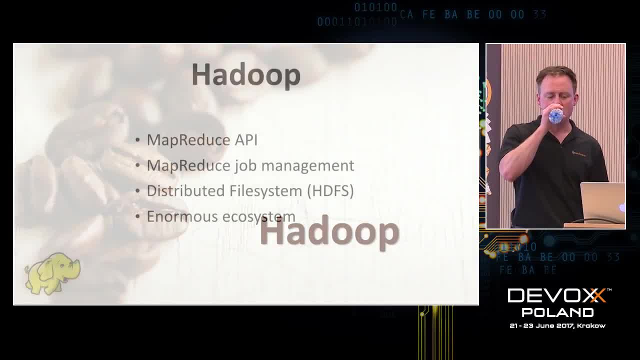 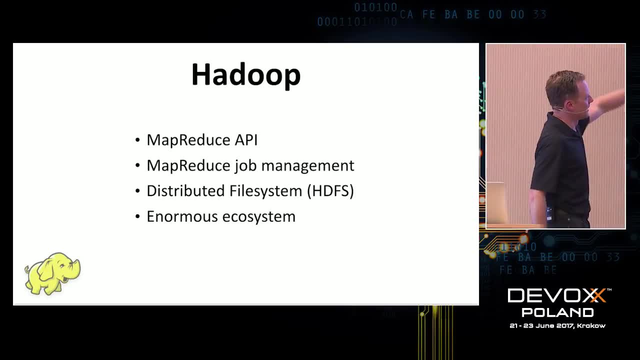 It is not the cool new thing anymore at all, But you should know that whole MapReduce thing. yep, that's the fundamental layer, the bottom of Hadoop And the other- I think, more long-lived part of Hadoop is the distributed file system, HDFS. 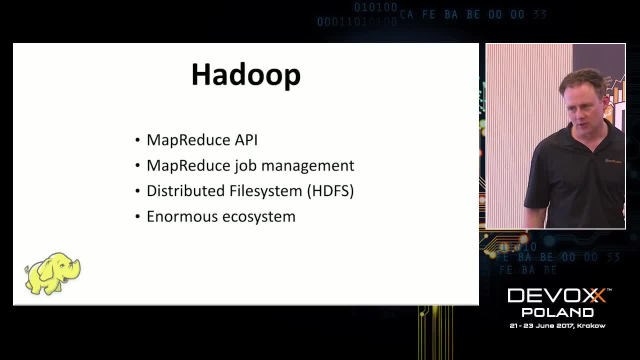 That is, in the words of one of its co-creators, a cockroach. Nobody is really building any new MapReduce systems anymore, And that's not. you don't see that in lots of new designs. HDFS is going to be with us until our grandchildren. 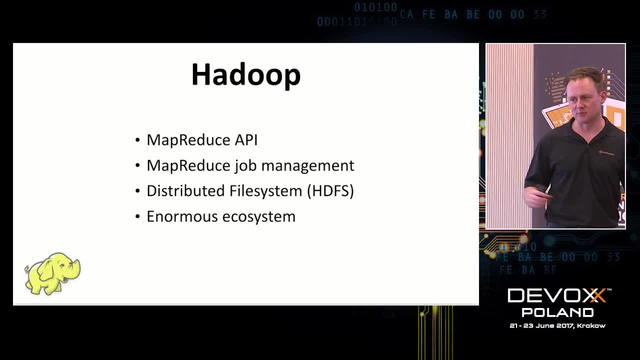 are writing software. I think It's probably going to be a very long-lived piece of infrastructure, and for good reason. It works just fine. Hadoop spouted an enormous ecosystem, and not necessarily in a good way, in my opinion at least. 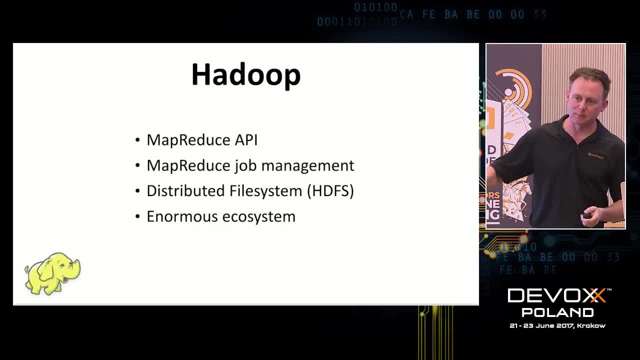 It became very, very complicated because the underlying programming model was so terrible that we needed this big ecosystem of more pleasant layers on top of it, And that's kind of what happened. Things like Hive grew up and that became a relatively pleasant way to use Hadoop. 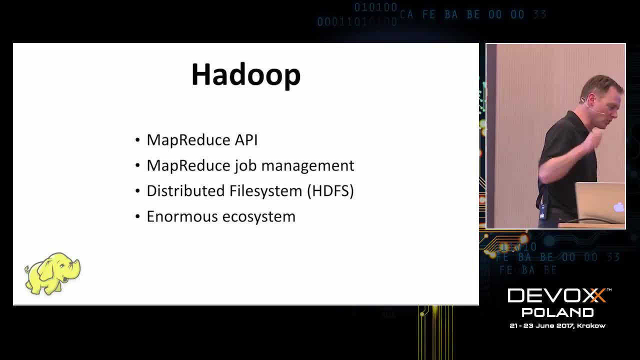 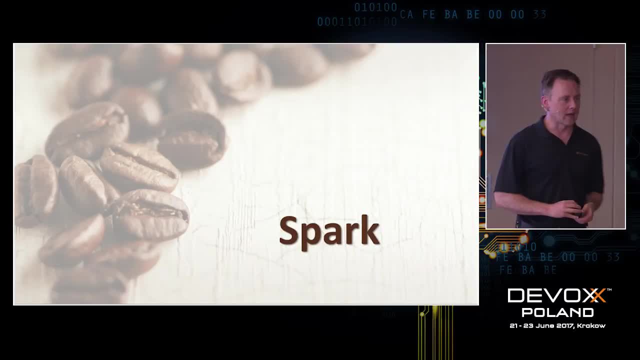 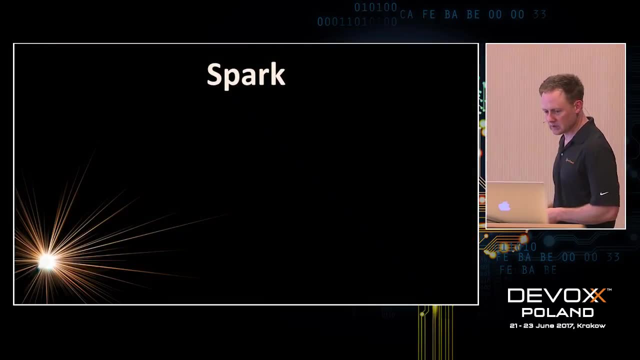 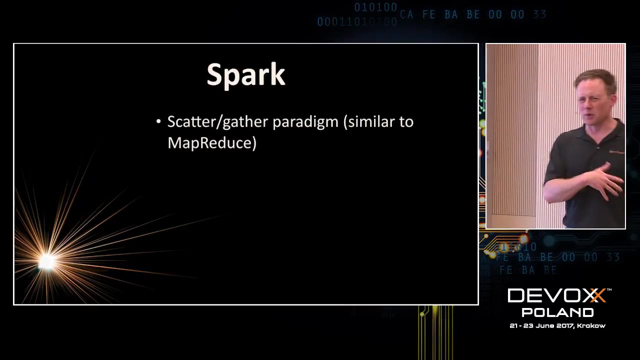 Actually programming MapReduce. not many people did that, Which is why a tool, when we keep going through the world of distributed computation- a tool like Spark, has really taken over the mindshare of MapReduce in the last three years, The way people have been talking about Spark, at least when it was new. 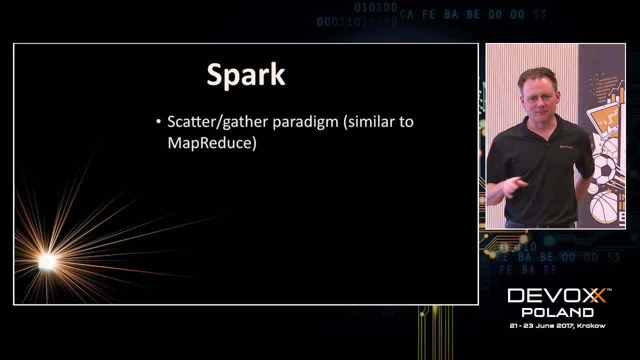 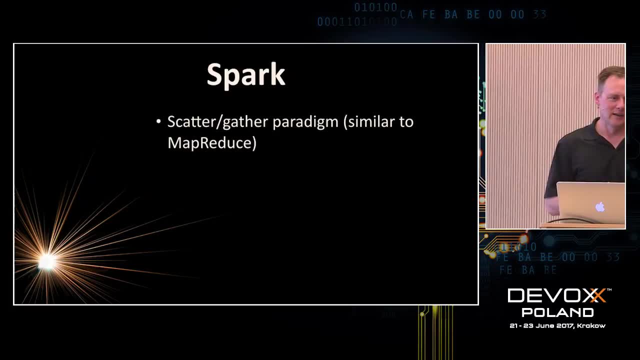 they would start off by saying, hey, this is a way better thing than Hadoop, Just believe me. and MapReduce is dumb. And then you start looking at Spark internally, you kind of learn the API. You're like, yeah, this is way better than MapReduce. 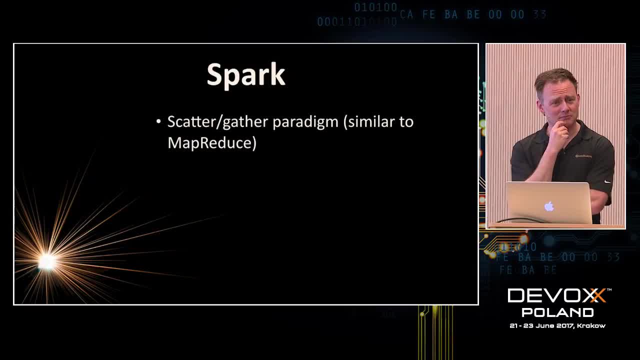 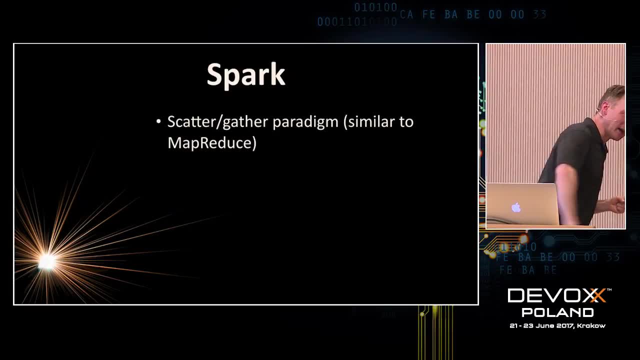 Instead of Map. I have Transform Instead of Reduce. I have Action. I like it. So the underlying paradigm is still very similar. We still assume we've got a bunch of data sitting out on a bunch of computers and then we need to go to that data and do stuff to it. 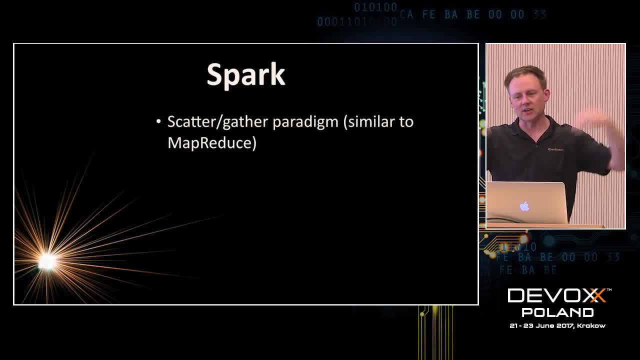 And if that's what you're going to do, then that basic scatter-gather paradigm is always going to happen And it's probably always going to follow that basic MapReduce sort of duality. Now Spark's insight was to say let's create an abstraction on top of the data. 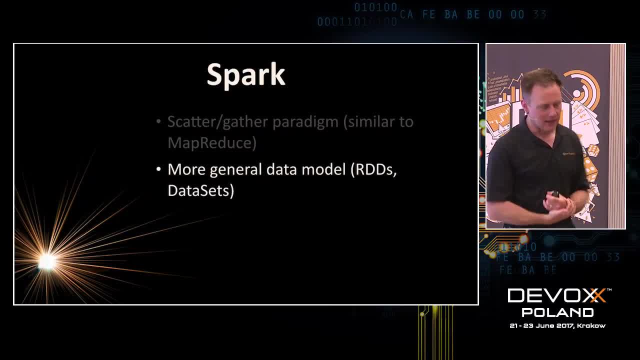 that's officially a part of our API And originally in early versions of Spark that abstraction was the RDD. Now kind of the front-facing abstraction in Spark is a thing called a data set. It's very similar but in contrast to Hadoop, Spark gave you an object. 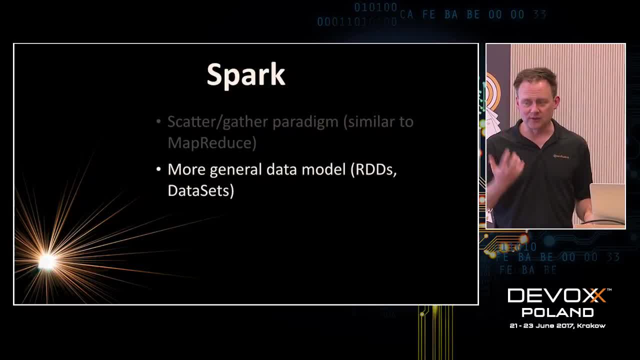 that you could program. When you're writing MapReduce code, you feel like someone is hitting you with a stick. When you're writing Spark code, you feel like a programmer. You've got an object that represents some big collection of data And what do you do? 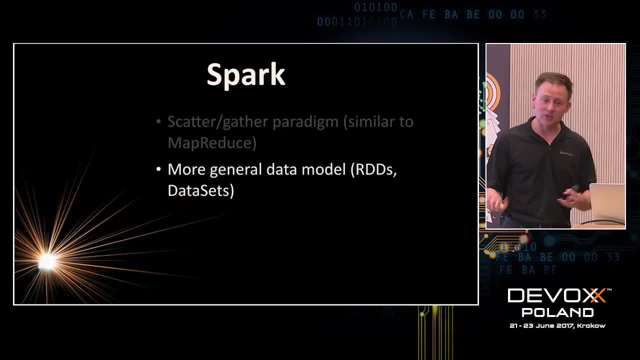 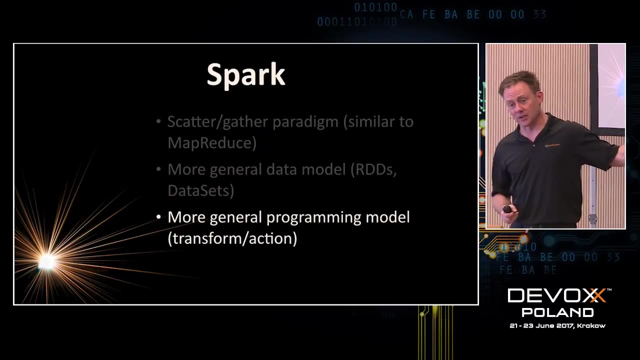 You call methods on that object and it does stuff to it. Now maybe they're essentially Map and Reduce that just have a little bit of syntactic sugar on them. but the Spark programming model is so much more developer-friendly than Hadoop that MapReduce has even in the eyes of the Hadoop vendors at this point. 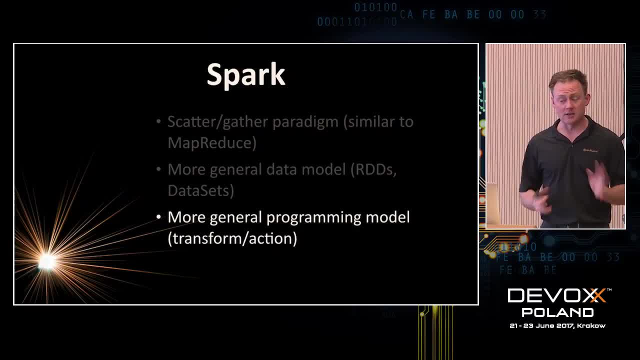 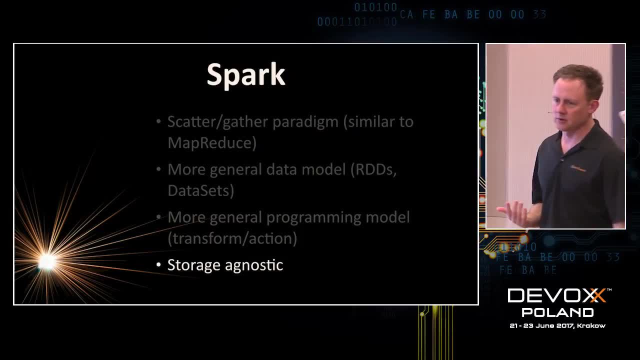 essentially been completely taken over by Spark, And it deserves it. Spark is a much, much more pleasant way to write code. It also doesn't have storage opinions. Hadoop's MapReduce really said you could put data anywhere you want, as long as it's HDFS. 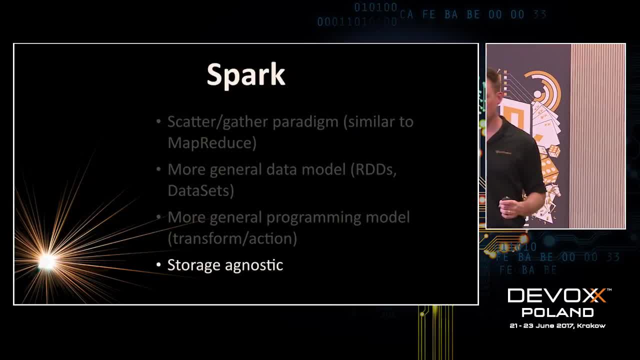 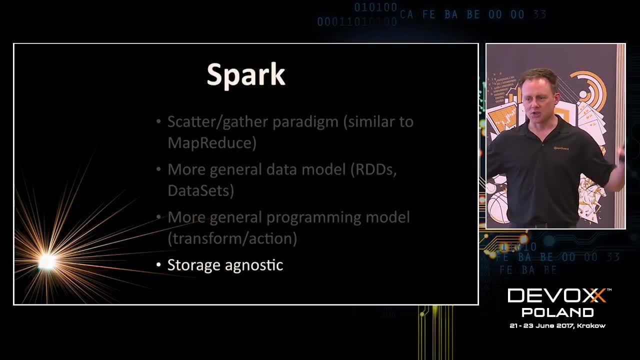 Spark says: of course, I will operate on HDFS data, I'll operate on Cassandra data, I will operate on dang, Parquet files and S3.. I don't care, It just wants to make RDDs and datasets and let you transform them and do actions on them. 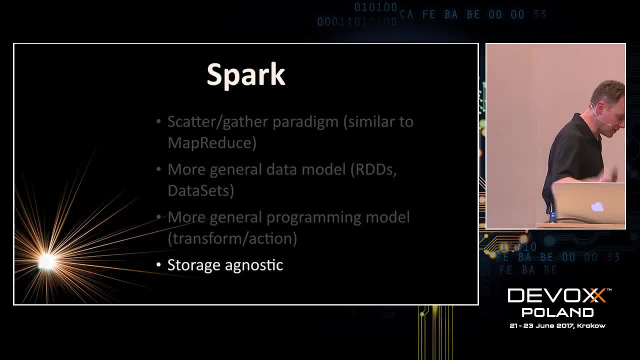 and do that distributed computation. Now the assumption is still in the world of Spark. Again, I've got a bunch of computers. I have a distributed storage problem. That's why we started with distributed storage. I have a distributed storage problem. 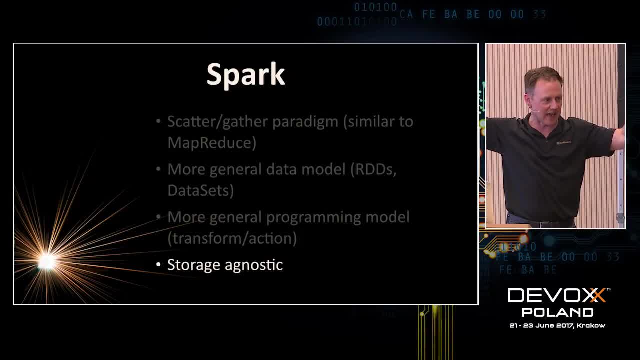 and now I have to do compute over all that data that's sitting out there. So if I have a distributed file system or a distributed database that's data at rest out there, then Spark, the Spark paradigm, still makes sense. Hadoop is the MapReduce paradigm. 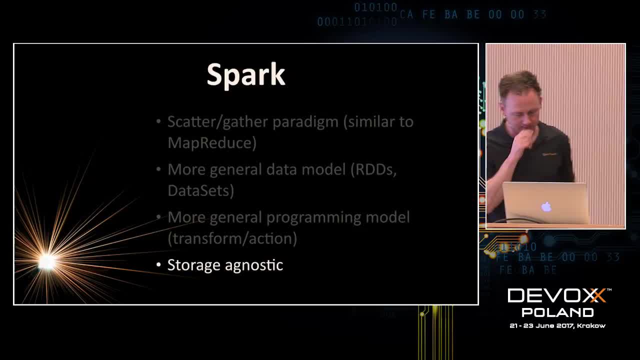 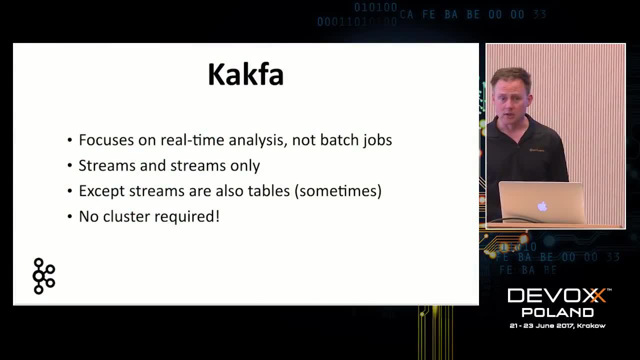 Really, you could think of that as yesterday's news, and Spark is more of a today thing. Now Kafka- it's not quite time for Kafka's day in the sun, but because we're talking about computation and in the last year Kafka has entered this world. 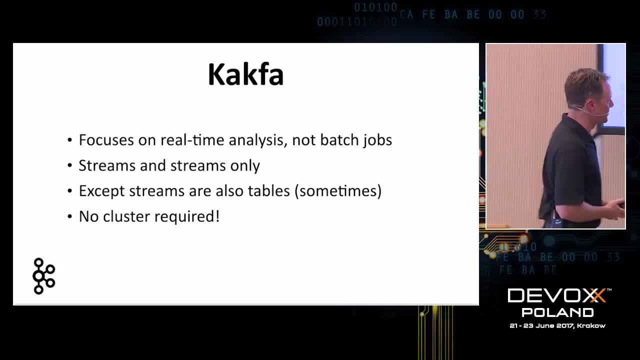 I should mention it is an approach to distributed computation in which everything is a stream. So as long as you've got streaming data, you can do computation on that streaming data. as the data is in flight, You don't have the assumption that you have put the data out somewhere. 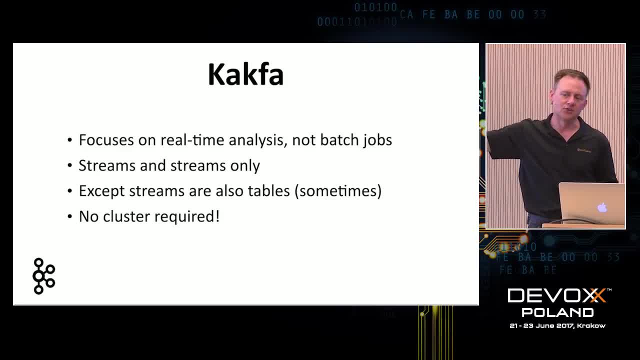 and you're going to go to that data and do compute on it. This is a stream processing framework where streams are first-class citizens and you don't even need a cluster to do. your computing Spark, importantly, also has a stream processing API. 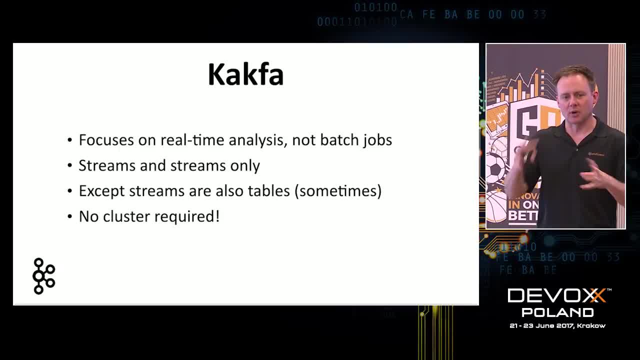 and it's not just API. There's actual infrastructure in a Spark cluster that helps with stream processing. There are other solutions to the stream processing problem, but Kafka needs mention here because it is not just a messaging framework, but is also a computation framework. 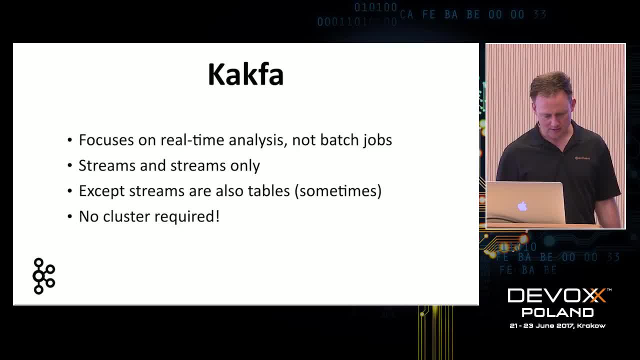 Now, all right, We are at about the T minus 15 minute mark. Oh, you know what I didn't say at first? I didn't say: if you have a question, ask it. Did you assume that It's a little late now? 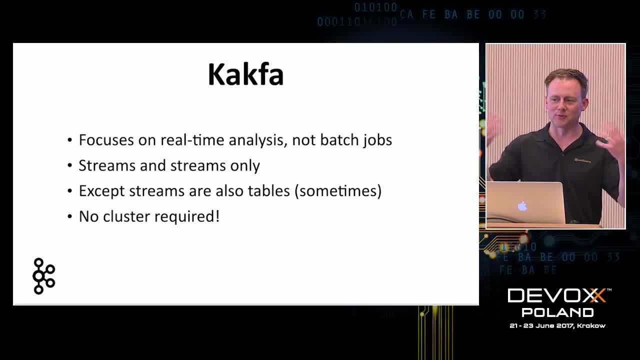 because I will never leave time for questions at the end. I always prefer that those just happen when they come Too late. Dang it Now, you know. If you've got a question, ask it. The worst thing I'll say is: I don't know. 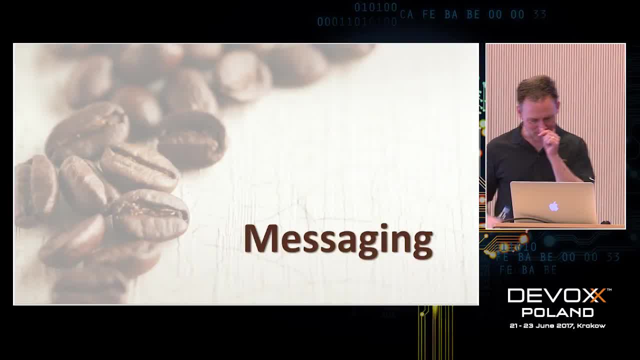 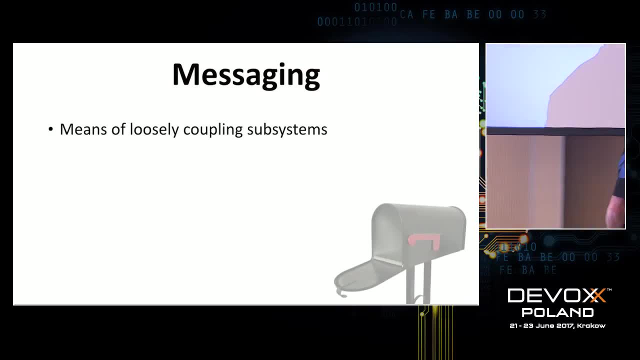 All right, Let's talk about my third promise, and that is messaging. Messaging is great because it lets us loosely couple systems and that lets us process and that lets us build little chunks of functionality and release them and version them independently and still have them communicate. 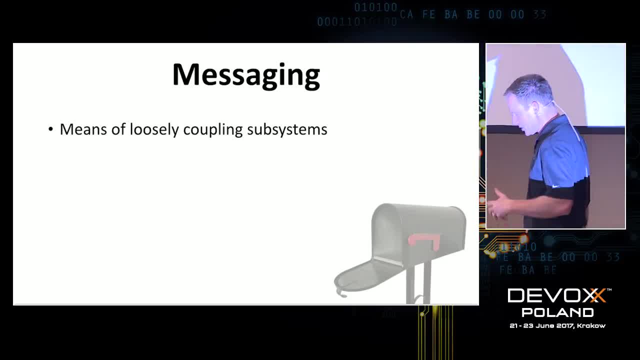 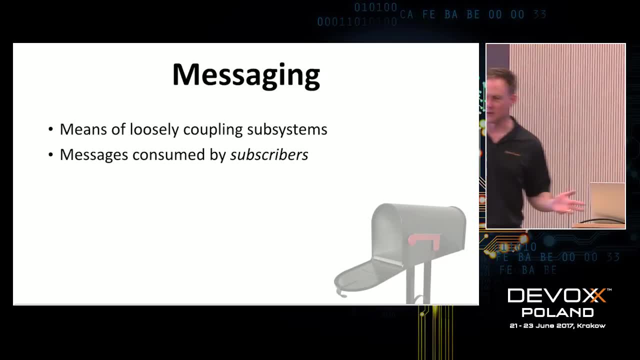 And does that sound like anything we do these days? If I say little chunks of the system that are released and versioned independently, that sounds kind of microservice-y and that's amazing. So messaging is because of microservices in the last three years. 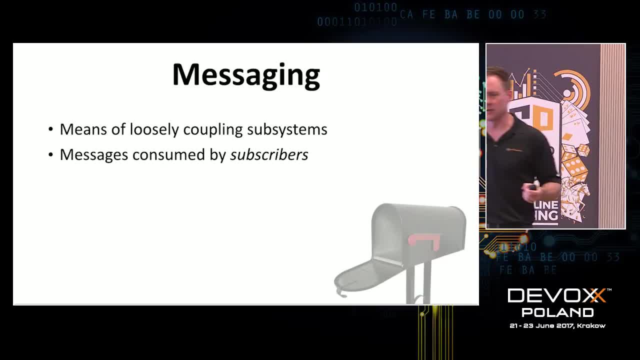 messaging and streaming I'm seeing come way more to the foreground in the last year or so. People are realizing that microservices are a super good idea for a number of reasons and people have been struggling with how to get them to talk. You know early. 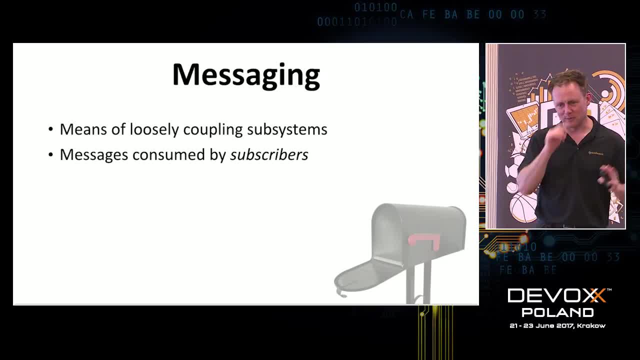 maybe this is your microservices deployment and I should be respectful but kind of an early approach to microservices is: well, let's just have a bunch of little pieces of code and one big database and they talk through the database. People realized that was a terrible idea. 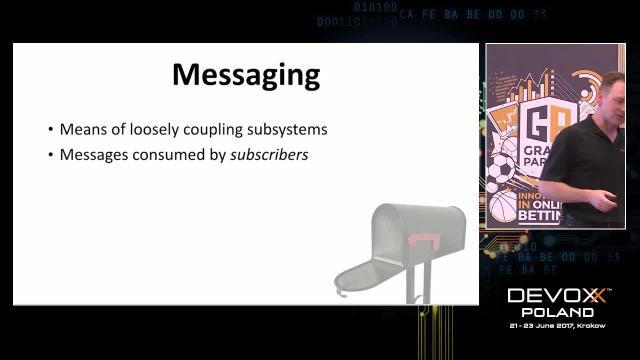 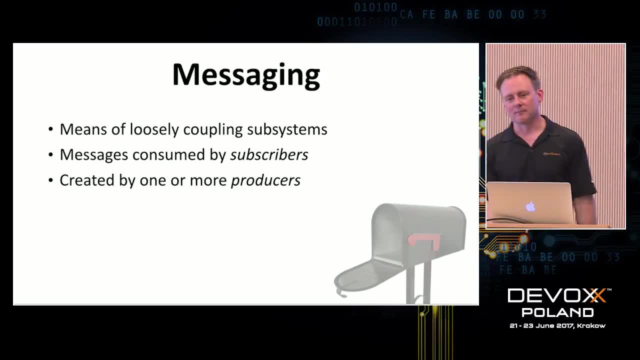 It didn't really work, And so getting those microservices to talk, suddenly messaging is coming back into the foreground, So it's a way of loosely coupling systems. We usually use the term subscribers or producers, Sometimes subscribers, we might call them consumers. 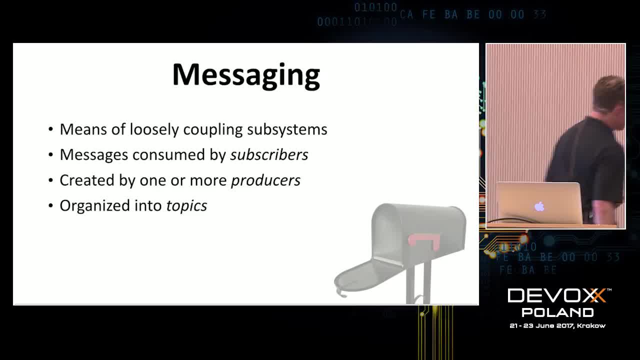 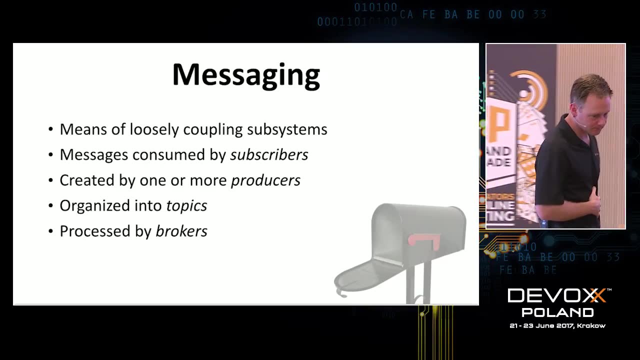 all these kind of words. We almost always in messaging systems organize them into named topics, which are just namespaces for similar messages, And there's usually this term broker, which is just a computer in the messaging framework. We typically think of messages. 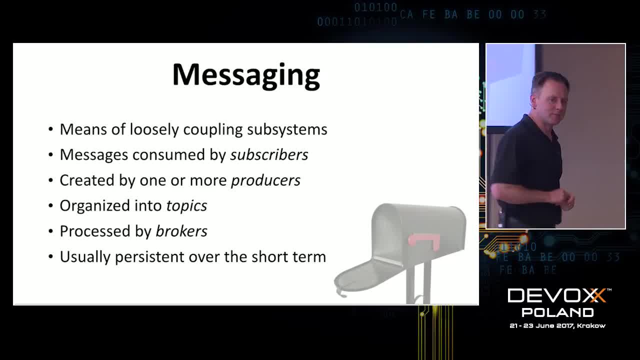 as being persistent over the short term. Now it's up to you how you define short term. The New York Times is an open source Kafka user and they keep all of their newspaper content going back to the 1860s in Kafka. 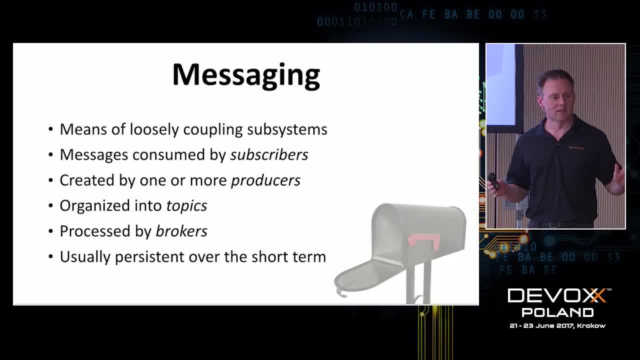 So you get to set the data retention yourself. And, believe me, 1860s in America is a long time ago, So that's a lot of newspaper data for us. Now, yeah, the basic idea here is: you've got a producer. 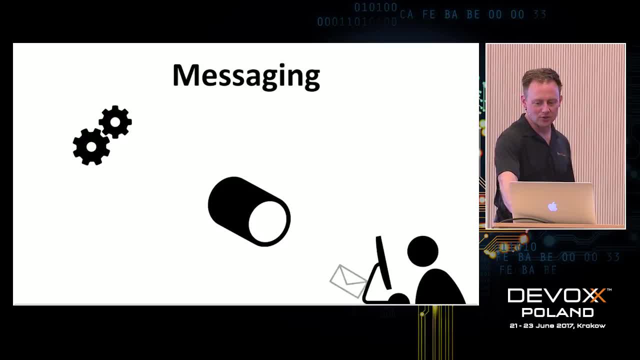 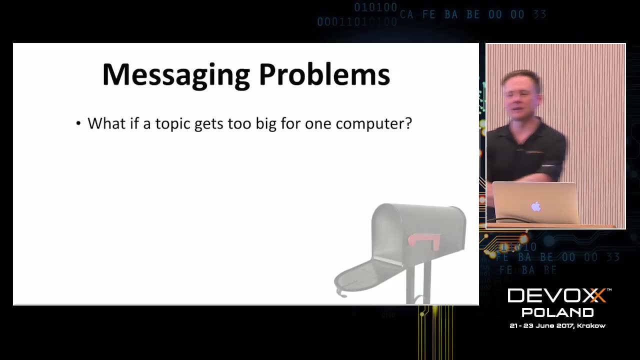 it sends messages into a topic and then the consumer gets to read those out at its own rate. The problem is when that producer gets big. What if a topic gets too big for one computer? Now, how can it be too big? Well, you can retain too much data. 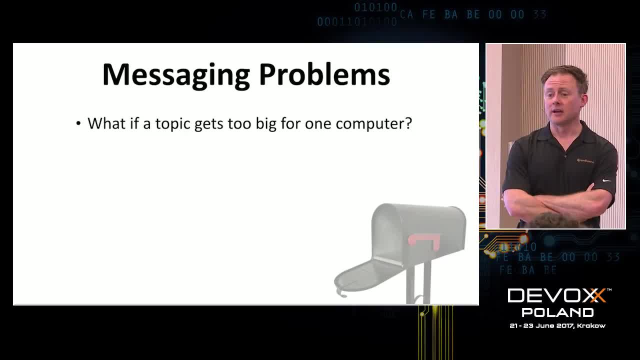 Suppose you want to retain data into the 19th century. Hey again, I'm not going to judge, It's your system. So that's big. Or your messages are big, Or you are transacting messages too fast for one computer to keep up. Maybe data retention isn't a big thing, but you're reading and writing too fast for one machine, given the fastest machine you can reasonably deploy right now. What if one computer is not reliable enough? Remember they break And you would like your system not to go down. 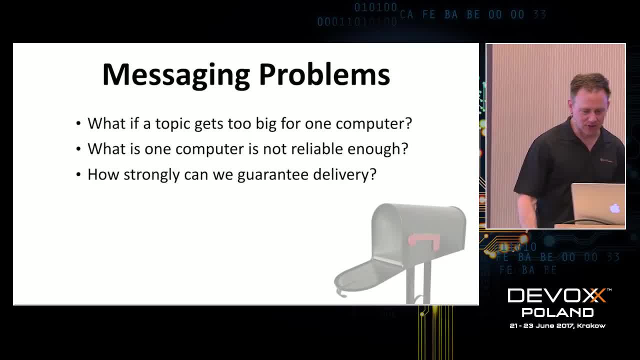 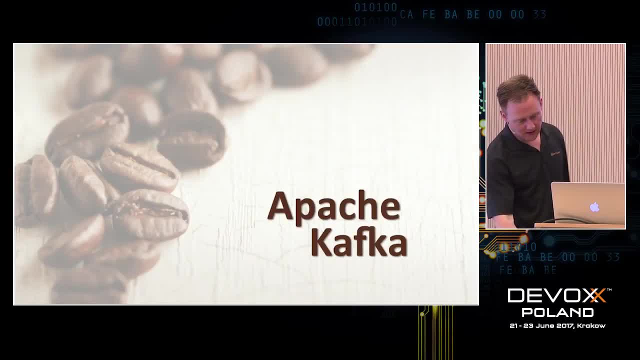 What if you really want to be able to deliver, to guarantee delivery, even if a computer is down? Well, enter Apache. Kafka, I should say. when you have a messaging system, and it is a single-server messaging system, it can do all kinds of fantastic things. 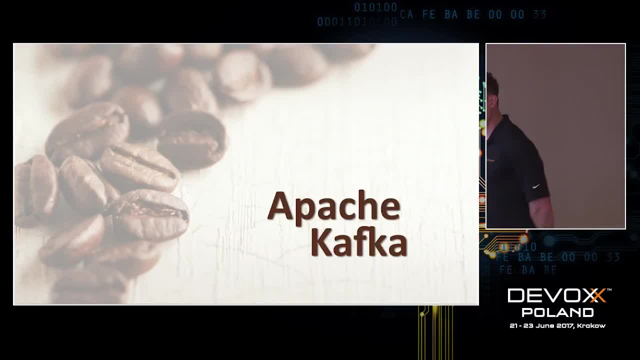 Like it can trivially guarantee that messages are delivered exactly one time. What it can't do is be particularly resilient to failure or particularly scalable. Oh, I should say also, it can always guarantee that messages are ordered. This is a message queue, after all. 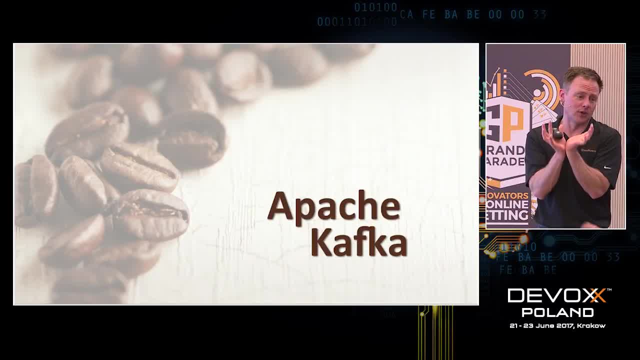 and we would expect messages to be ordered, And when I have a single-server message queue or message broker, then everything's great. My messages are always going to be in order. I'm going to have to give up on some of those things when I scale, but I'll get things in return. 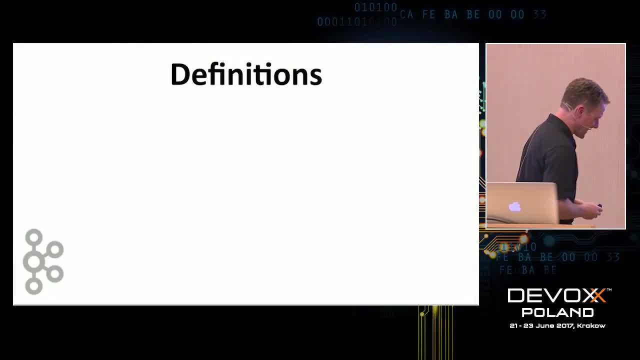 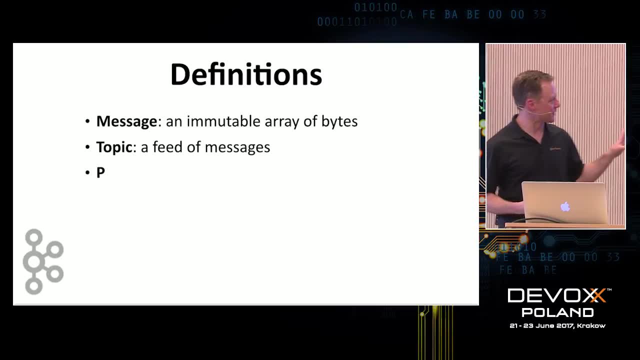 And, as it turns out, a lot of awesome things. So Kafka. Now just a few quick definitions, in case I use these words. Of course, message, that's the basic thing. Topic: I've already said that, Producer, this is a client process. 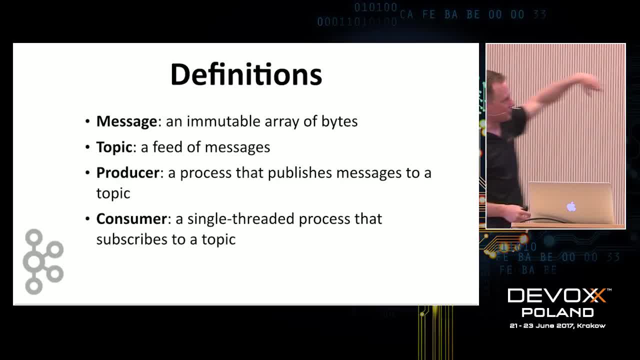 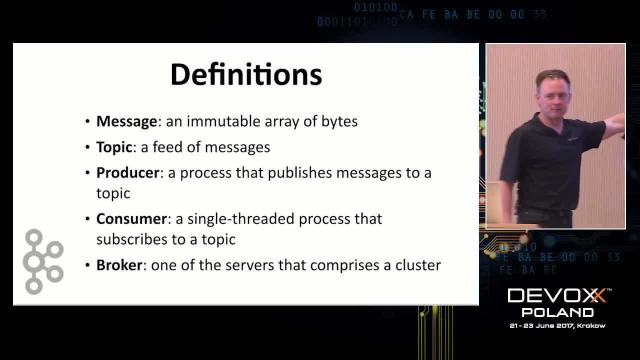 outside the Kafka cluster that puts stuff in Consumer. this is a client process outside the Kafka cluster that takes messages out, And broker is simply one of the computers that the Kafka cluster is made up of, So a broker will have many topics, for example, 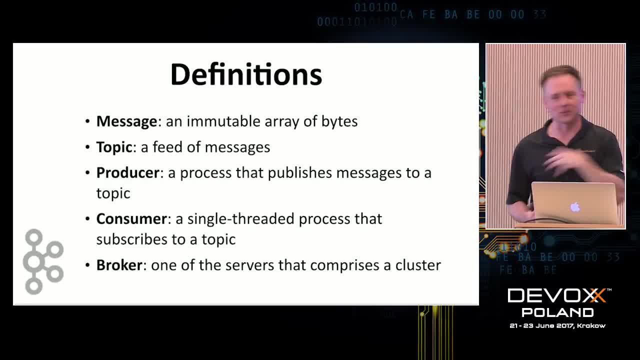 I'm not really deep diving on Kafka here, just like I wasn't deep diving on Cassandra. So it does things like replication also and it answers the consistency question also in various ways. So all of those problems come up and all of those problems are solved. 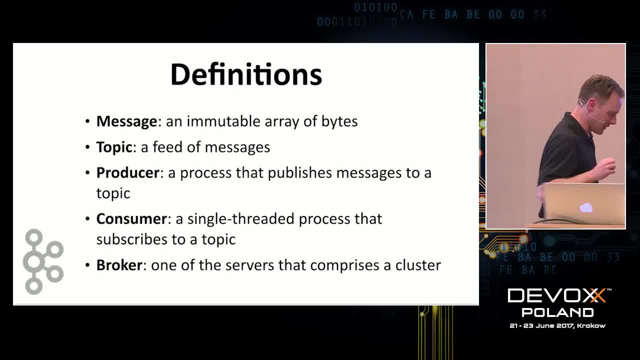 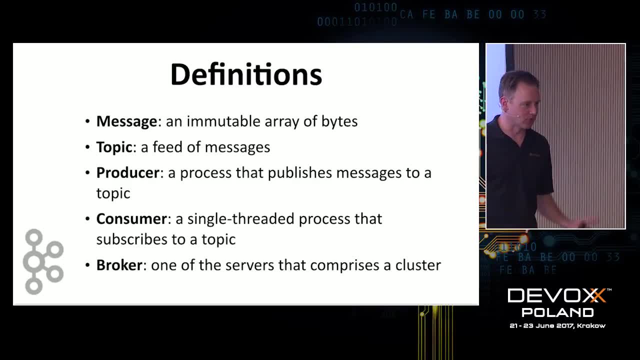 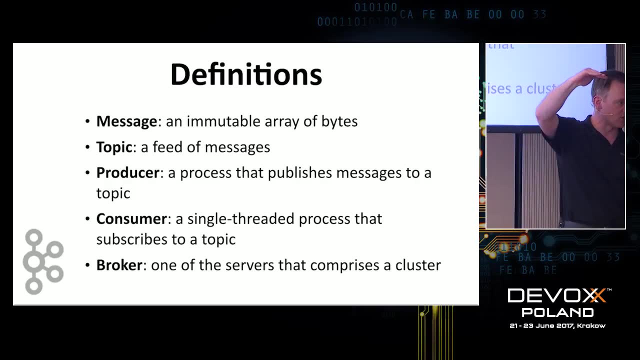 by this particular distributed message broker. But the money in Kafka. the really interesting thing is when we get past just being a message queue. So I want to show you how it works as a message queue and where the distributed system ugliness creeps in. 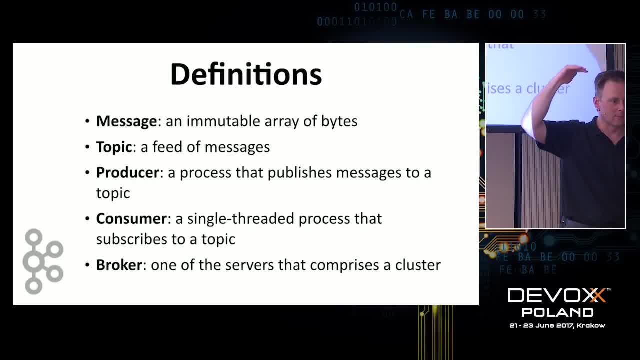 like what Kafka does to you. that's mean because it's distributed, and, of course, what we get in return for that. Then I want to talk real quickly in closing about what happens when we have made everything into a message Like: how thoroughly can you live that life? 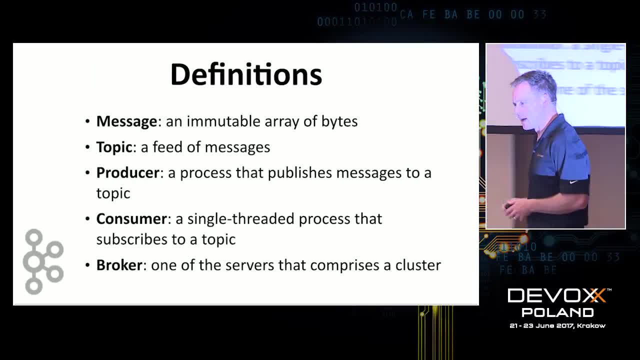 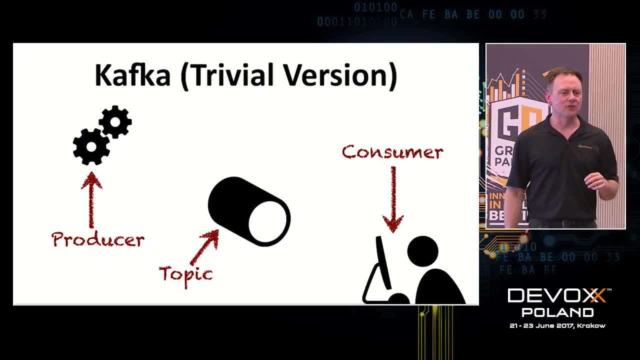 and what sorts of things happen when you do So. Kafka: all right Again. producer-consumer topic. This is the trivial account of Kafka: Kafka as a pipe, And this is currently how most people think of Kafka, because its value-added features. 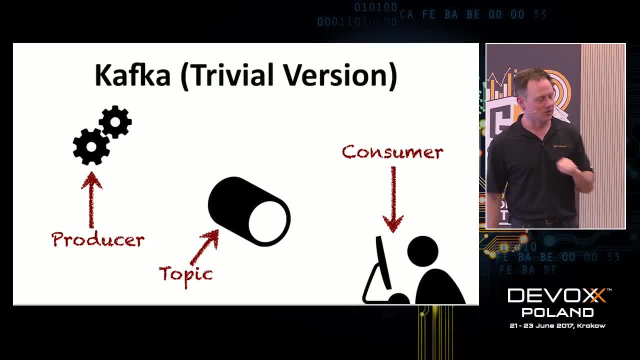 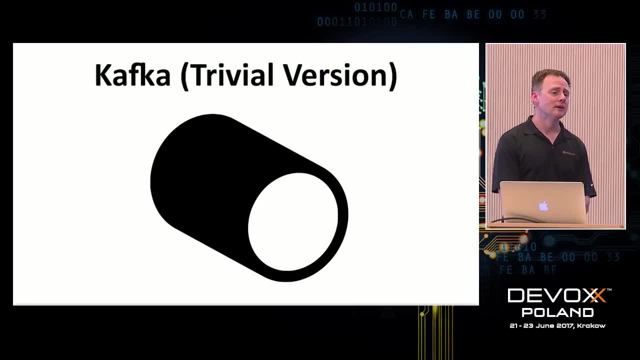 that are more than just pipe are really only a year old, So let's just go through the pipe version. When that topic gets big, what do we do? Of course we partition it. We'll just split that up onto several computers. 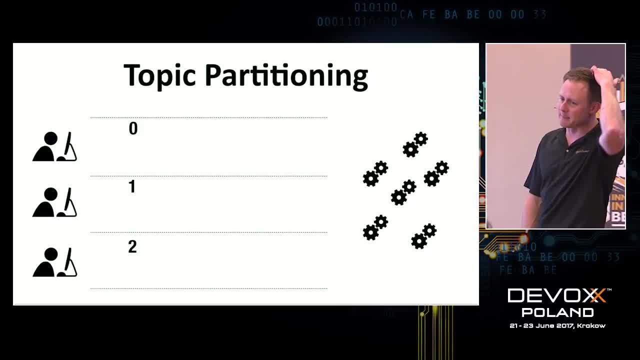 So let's say, instead of one computer, I've got that single topic partitioned over three computers. Now, each of these partitions, of course, I would also replicate. Just put that to the side for a moment. We're not going to talk about that. 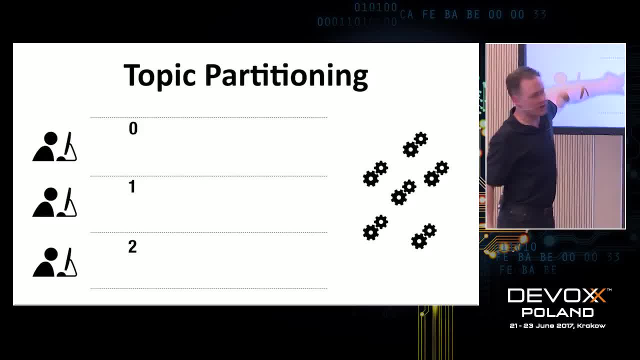 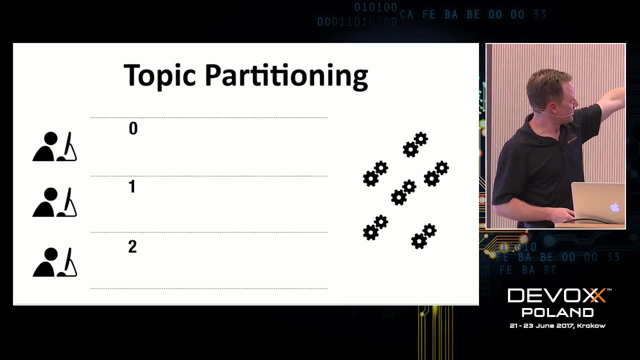 We've got these three partitions, So these three rows. here are those three brokers, each of which has one partition of the topics. These are independent computers. The gears over there are producers- They're going to produce messages- and the people working at, like, 2010 IMAX. 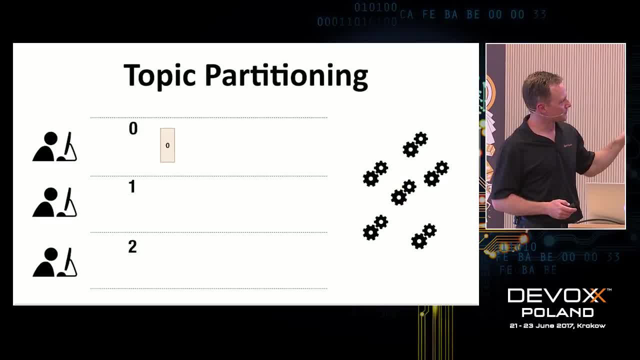 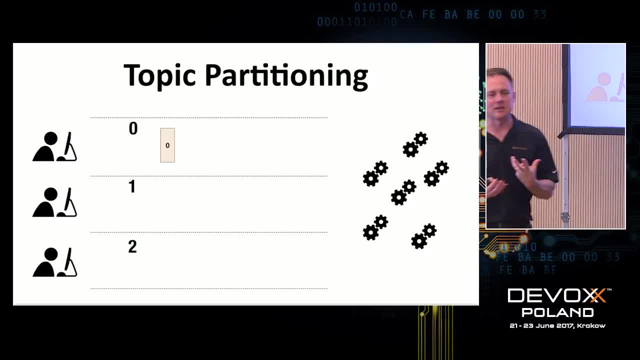 those are the consumers. So when I create a message as a producer, what's going to happen is we're going to look at some part of that message. Now, maybe I'll just hash the whole message, Maybe I'll look into a field of the message. 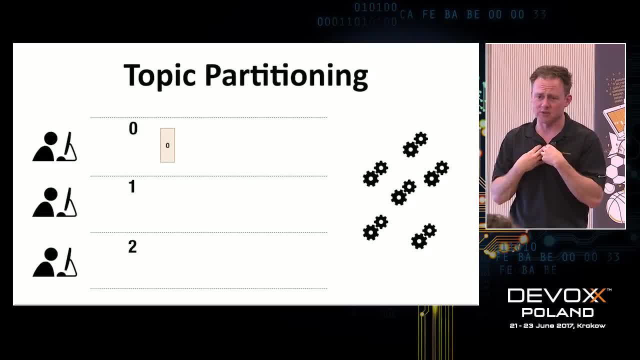 like username or IP address or something that means something to me as a producer. But I'm going to take some part of that message up to all of it and I'm going to hash it Now. this is like consistent hashing over there. 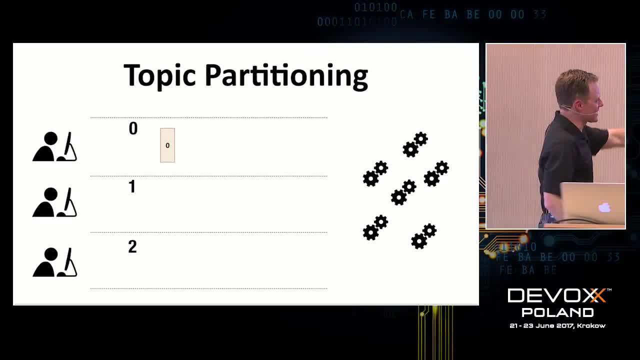 poking its head up and winking at you, like I warned you it would. I'm going to hash that message, mod the number of partitions and that's going to tell me what partition to write to Within each partition. I will be able to keep things in order. 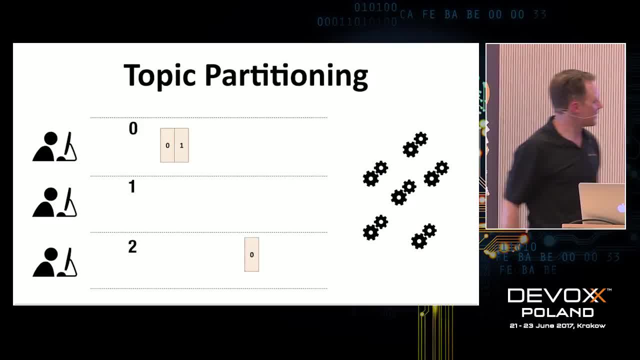 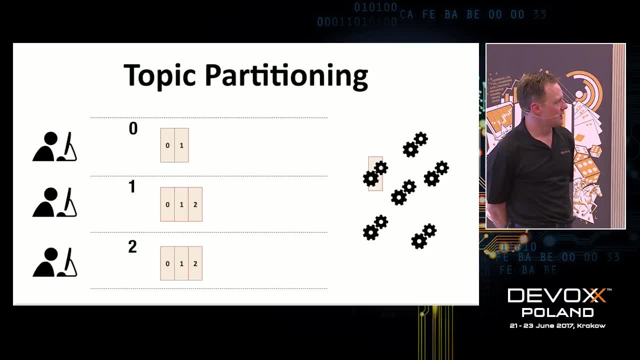 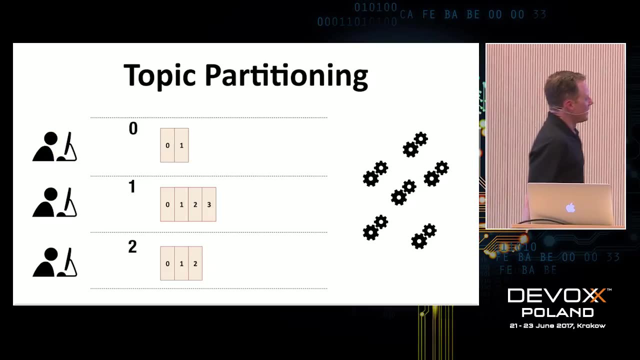 Each partition is ordered, So I'm going to keep writing in here and I will kind of randomly, really, or uniformly, have these messages assigned to my partitions. Oops, I consumed one. Let's not consume that yet. Now, already, you can't remember. 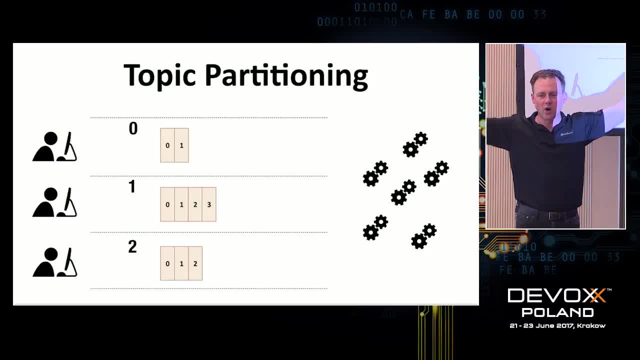 what order these happened in. System-wide or topic-wide ordering is lost Because this is a distributed message queue, I can only have ordering within a partition. That's a limitation I have to accept. I don't get global topic-wide ordering. That's a bummer. 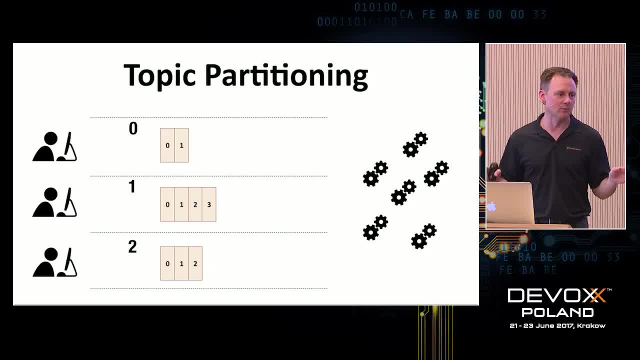 I would love to have it. There is no day I will wake up in the morning, roll out of bed, have a cup of coffee and say I literally do not want global ordering on my topics. Darn it, I wish I didn't have it. 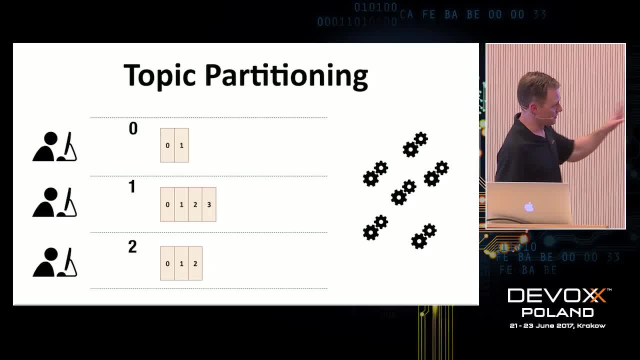 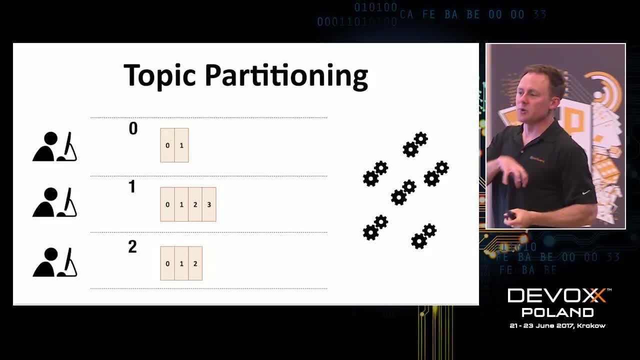 Shake my fist at the heavens. It's just not going to happen. I would always want it but I can't have it. It's just not a possibility. But I do have it within partitions At the user level. you can be smart. 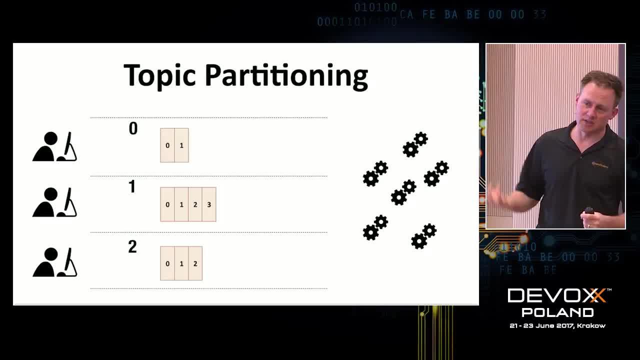 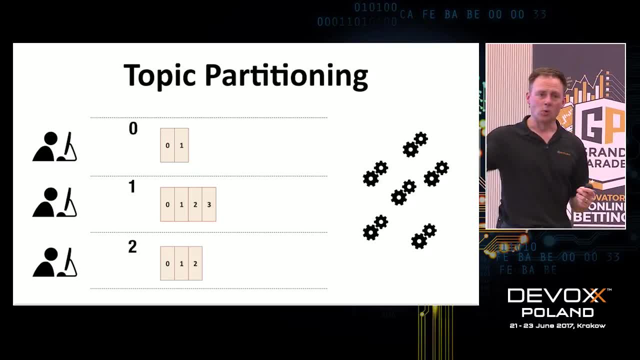 about what part of the message gets hashed, And so I can guarantee within a topic that messages from the same user or from the same host, or from the same whatever, will always end up in the same partition, And then I can consume them in order from each consumer. 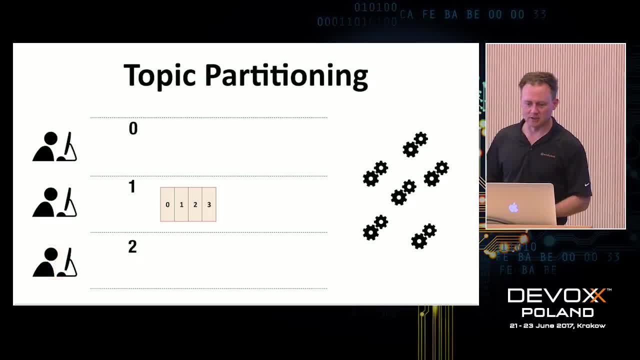 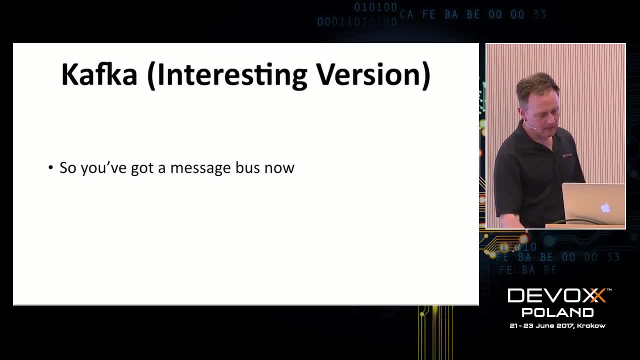 And those consumers are independent computers operating independently, scaling my system like a boss. So cool, I have a message bus. I have solved the problem of distributed messaging. I already came up with a way to solve distributed storage. We talked about one. 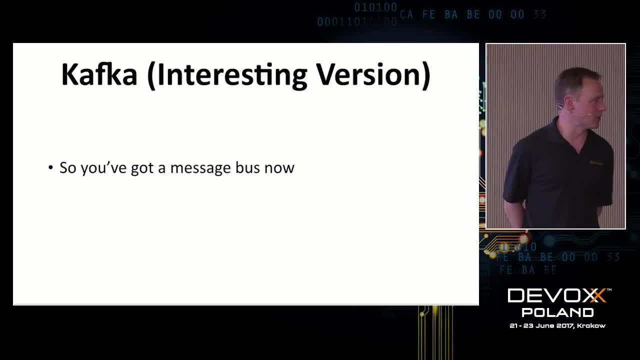 I came up with. there are a few different ways to solve distributed computation. Now I've got this distributed messaging system, So all my services can communicate with one another through topics in this elastically scalable- essentially infinitely scalable- message bus. That's great. 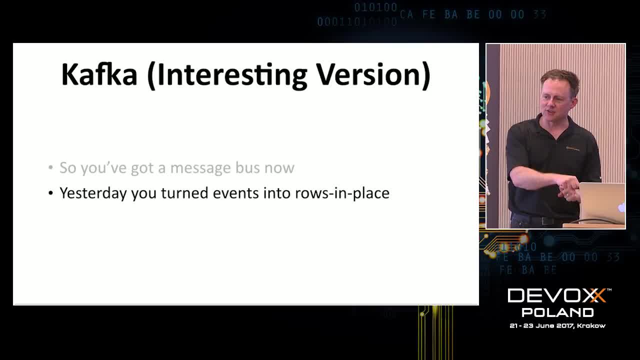 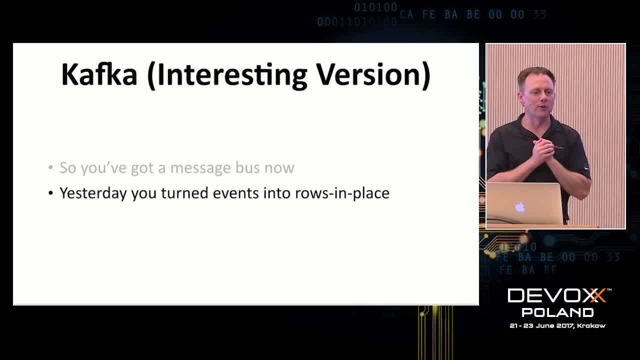 And that's what I did. I would generate events into this bus- This is kind of how people start out- And then I would consume service, would consume one of those messages And what do I do? I write it to a database. 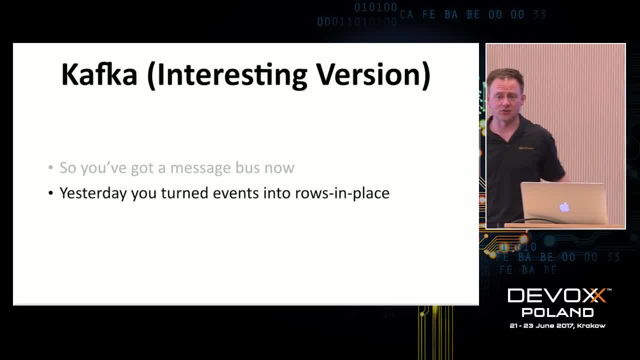 So I've got this event and I turn that event into a row And that row sits in a place. The data is sitting in a place somewhere, Maybe tomorrow. instead of doing that, instead of saying here's an event, I'll put it here and I'll go back here. 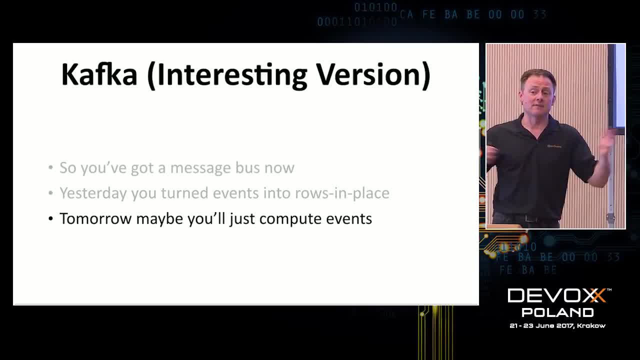 when I need it. maybe tomorrow I could just do computation on the events. I've got a giant message bus sitting there and everybody has an API. Everybody is coupled to that bus. through that API they're producing, they're consuming. Maybe I could do that. 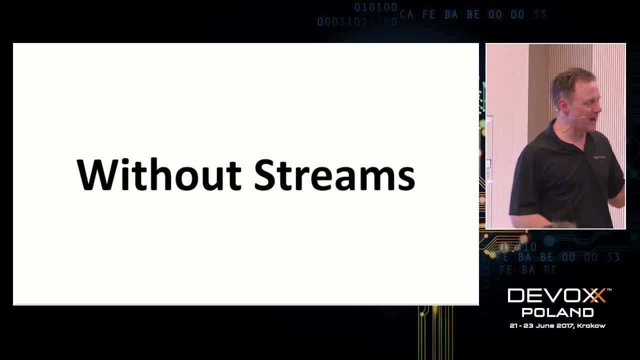 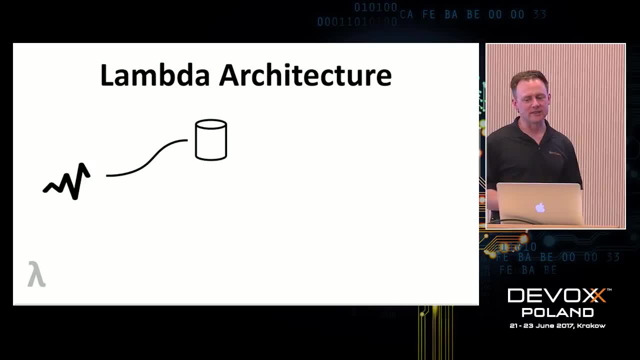 So without that, what is now really an anti-pattern emerges. About seven years ago this was considered pretty cool, and it's the so-called lambda architecture. That means I've got all these events out here and I have to build two parallel systems to process them. 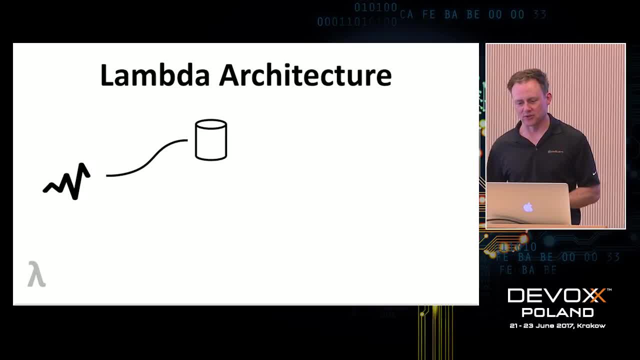 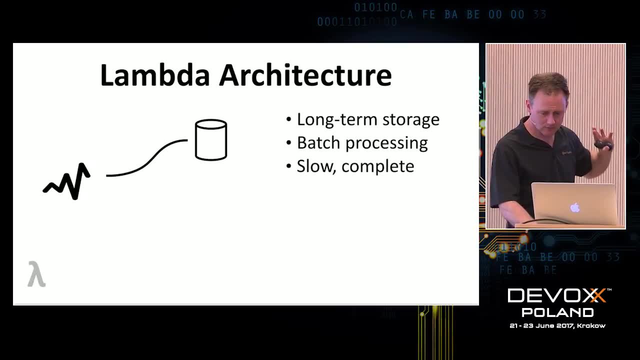 This is what happens if you don't use your message bus thoroughly. I have one system that all my batch processing takes place in. That's my distributed database. Those are slow but they're very thorough, Those jobs up there. they can take minutes or hours. 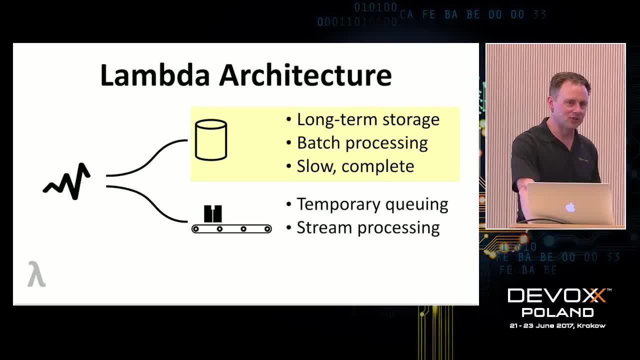 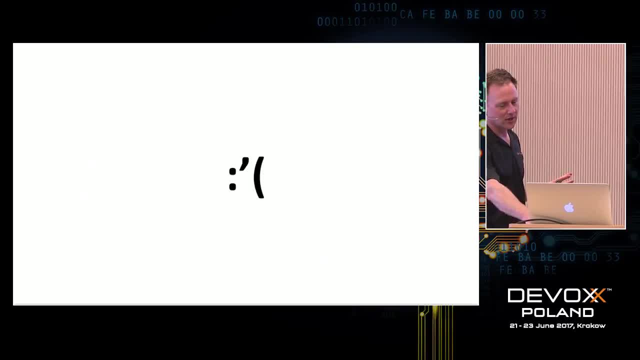 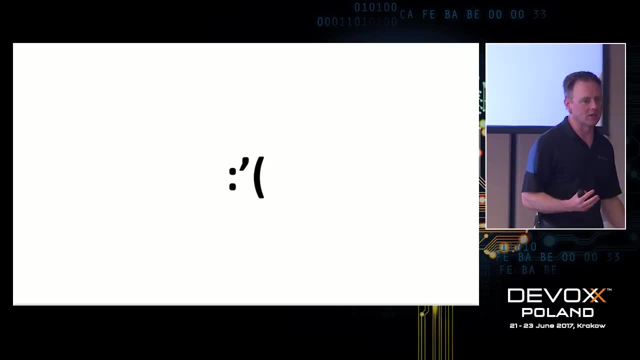 And then I've got this other system down here. that really is just my temporary message bus thing and I might do little bits of stream processing. for quick summaries, This lambda architecture emerges. This is bad because essentially what it did to us, and if you come to my talk this afternoon, 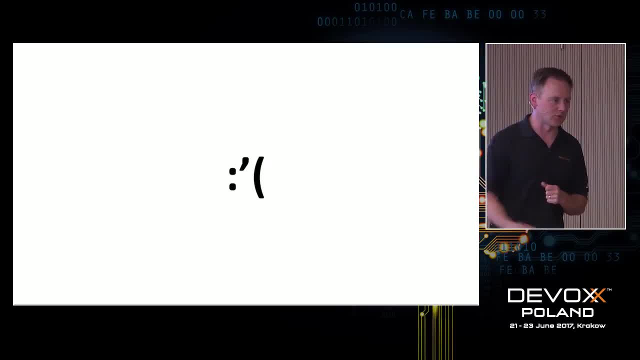 I'll talk about this in more detail. is it forced people to write the same code twice? You had to write the stream code and the batch code, And they say the best code is the code you never write. Well, the worst code would be: 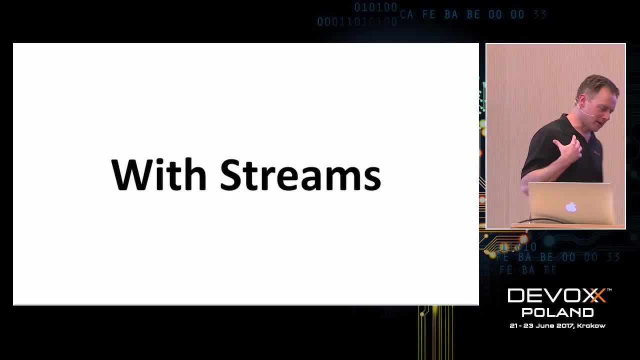 the code that you write two or more times. That's a terrible idea. So the basic idea: once I've got a message bus and I say: hey look, how about I stop obsessing over writing them to some place in a database and why not just? 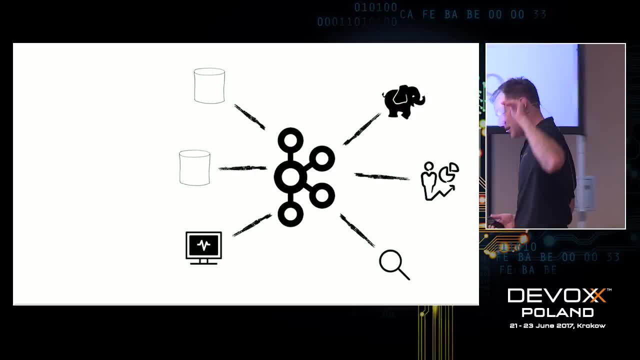 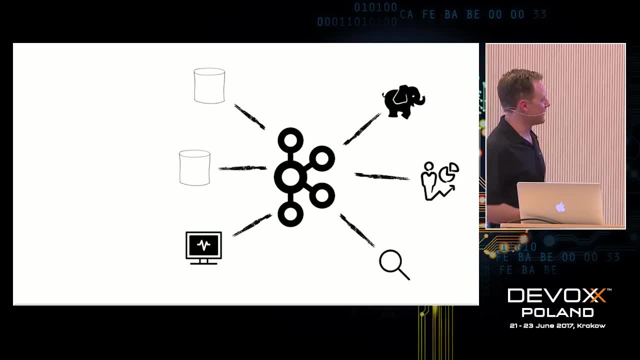 let them be events and process them in place through the, you know, through a stream processing API at the very top level. I could do something like this. I've got a Kafka cluster and I've got various services attached to it. I've got some service maybe. 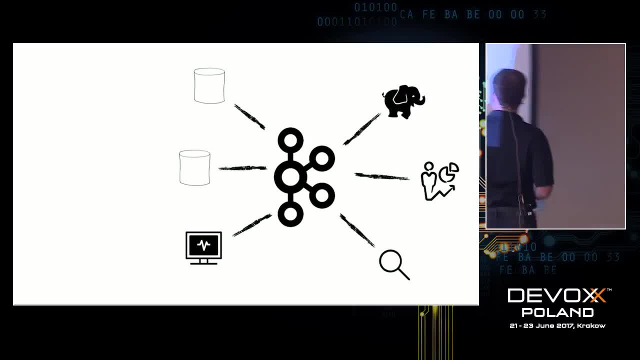 that's doing some analytics, or some monitoring- a service that's doing some analytics. I've got a couple of little databases. I might even maintain a local database, but all of these are services. I might even have a Hadoop cluster, because it's still there. 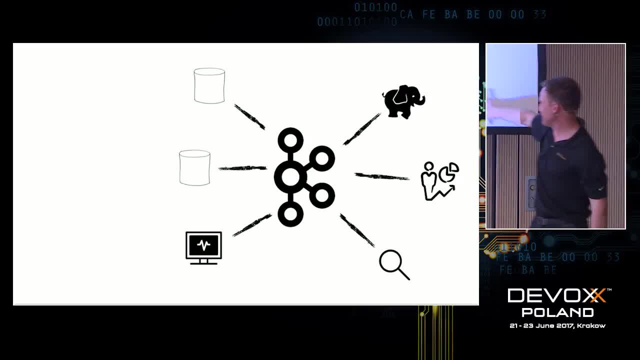 and we spent a lot of money on it, and the CIO doesn't want to get in trouble for not using it, so you have to keep using the Hadoop cluster. I might have an Elasticsearch cluster down here, all doing different kinds of things. 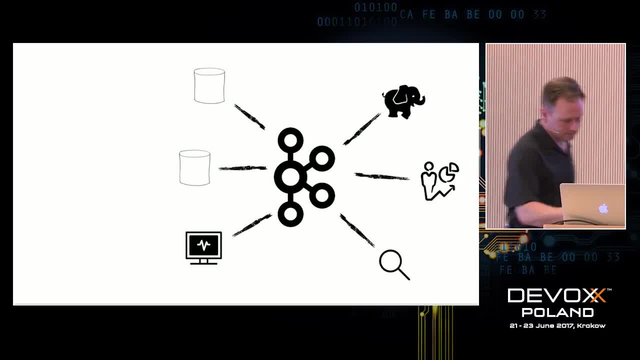 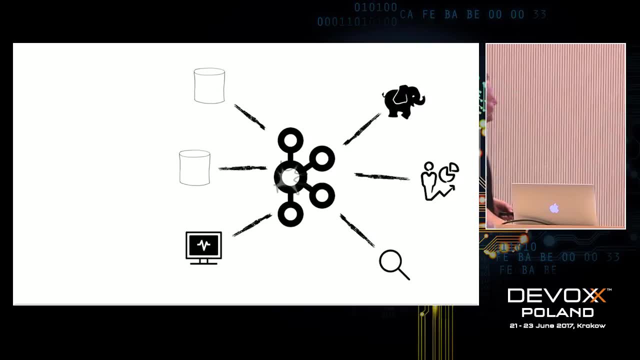 that my system needs, based on this messaging bus that they all talk to. Pardon me, Oh, I already did this and I just wasn't looking at the screen. You have events out in the world that go into that cluster and get propagated to the services that need them. 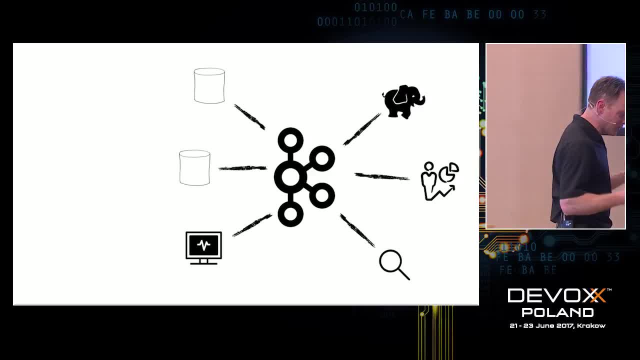 And the nifty thing here is each service doesn't really need to worry about what other services might be doing with it. An event is just an event. It happens, it's there in a topic and a new service can grow up and say, hey, I'm interested in that event. 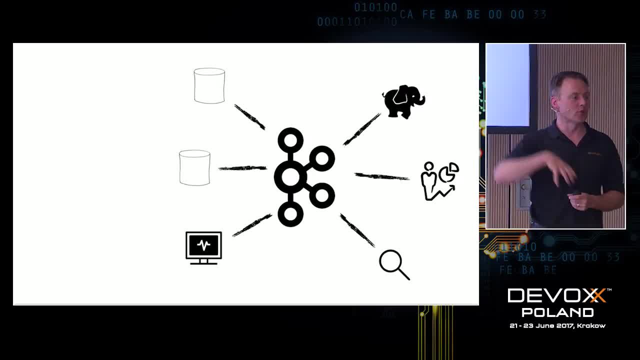 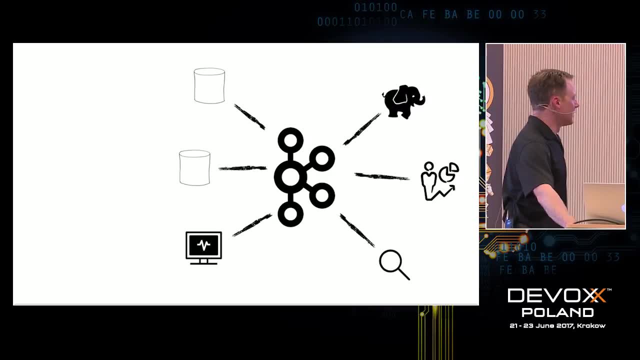 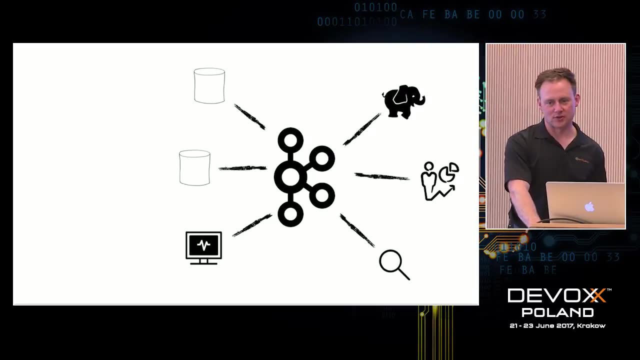 without having to have any coupling to the way that event is produced or who else might consume it. So once I start putting things into a message queue, I can be. It can cause me to think very differently about the architecture of the system. This can be an impactful thing. 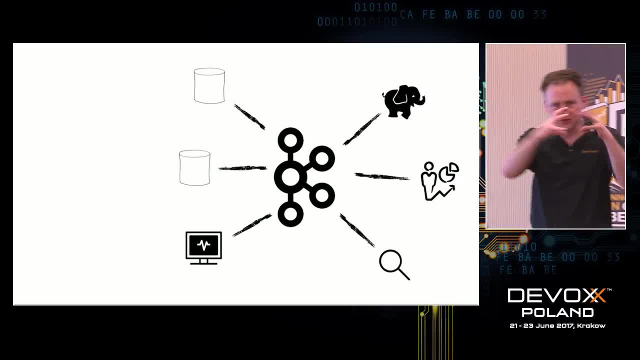 this distributed messaging thing. It's possible to go from my single-server relational paradigm to a distributed Cassandra paradigm. I have to change my mind about some things: about the way consistency works, about the way data modeling works. That's a big deal. 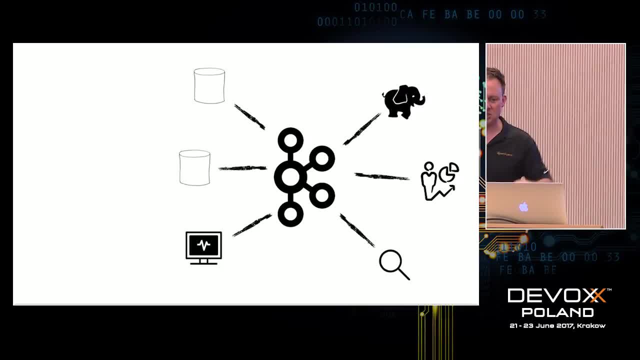 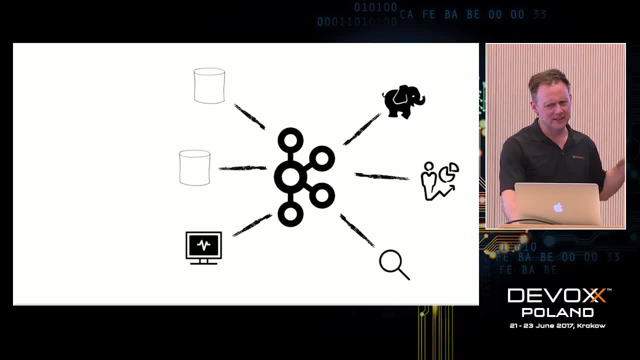 When I go from single-threaded programming to distributed computation. that's kind of hard. That's a tough thing to do When I get streaming into my blood suddenly the world is very, very different and I start building systems in a very different way indeed. 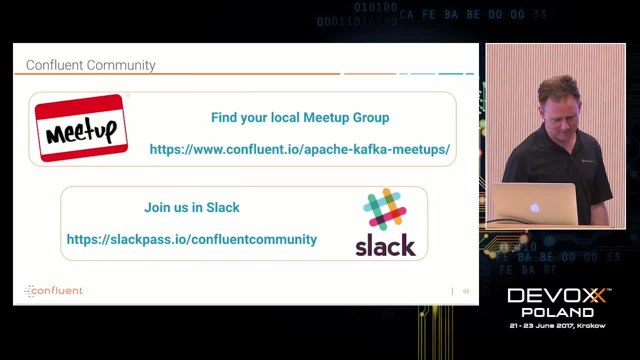 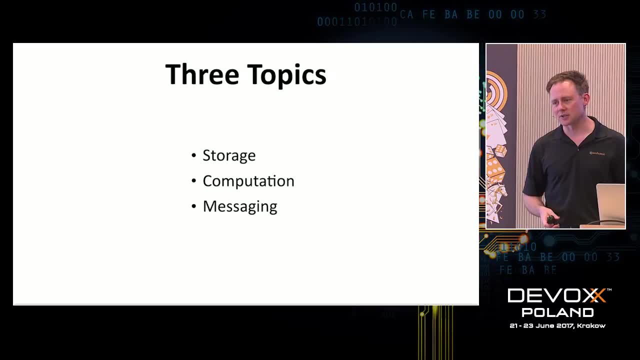 Now, with that just about out of time- and we have covered storage, computation and messaging- a brief introduction to a few things that go wrong and right when you build distributed systems and how a few open-source projects solve them. Shameless plug. 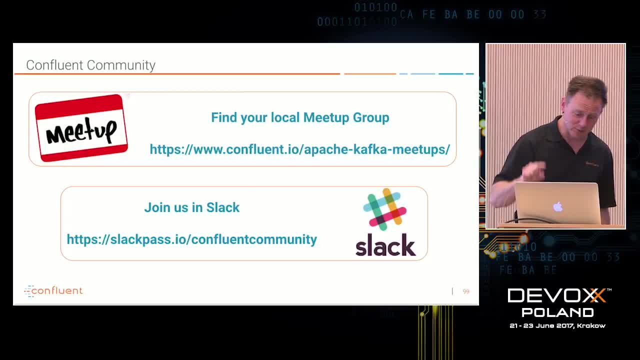 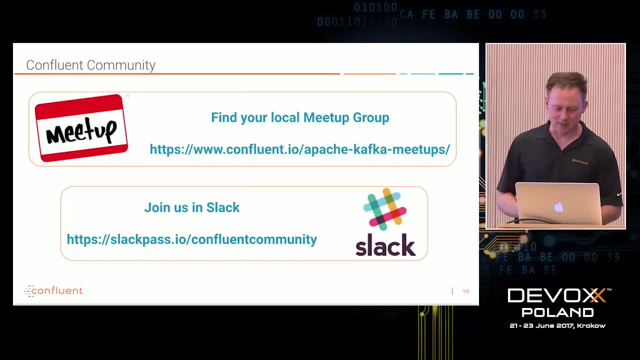 videos by the same name on O'Reilly if you care to learn more. Absolutely not shameless plug for Kafka meetups, because this is what I do. If you're interested in more, check that out. Take a picture of that slide if you want to go to a Kafka meetup. 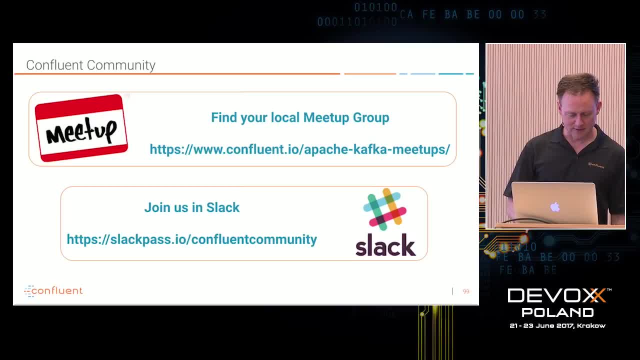 I would love to see you there. Sometimes I am even seen in Europe, not often enough. Thanks for having me here today. Have a good day.